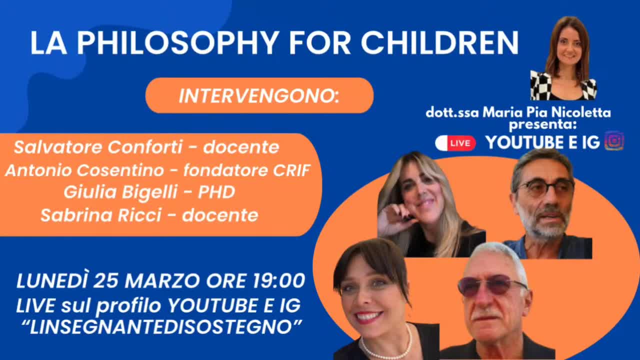 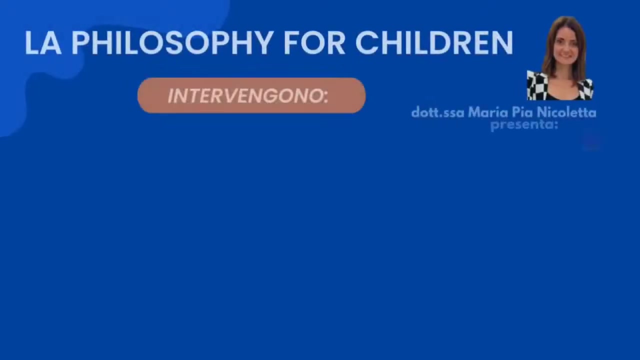 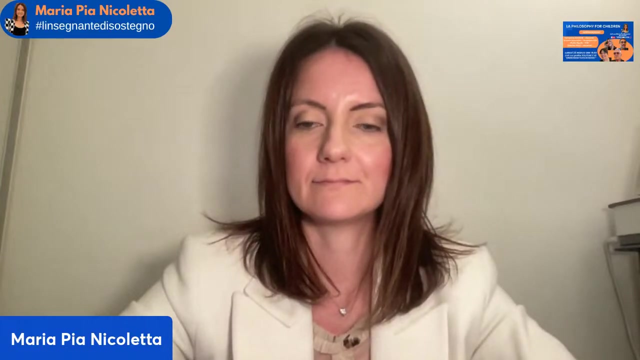 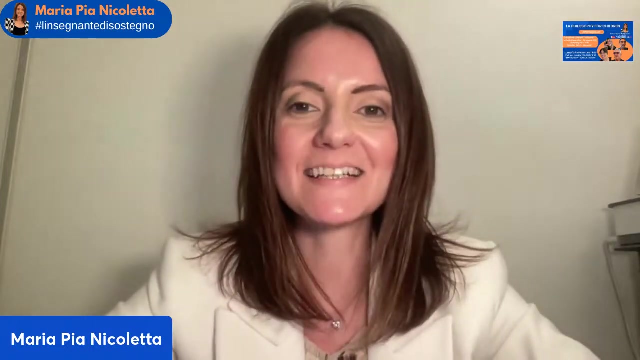 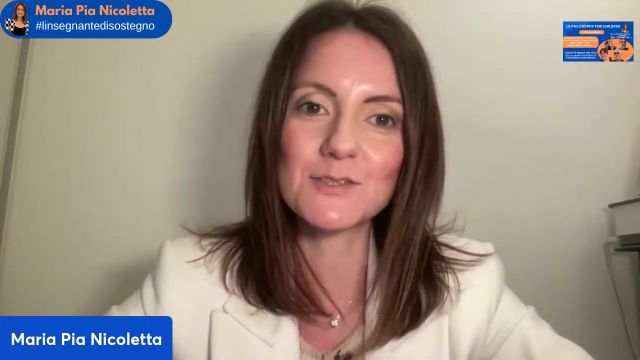 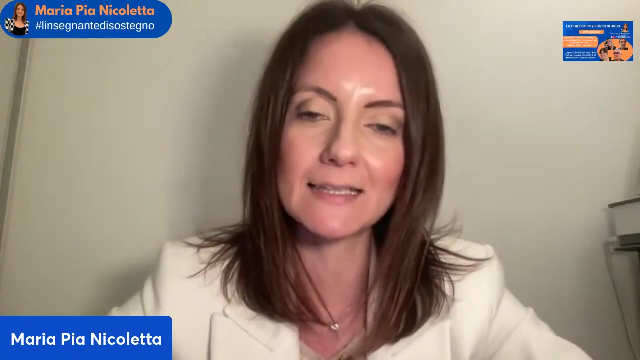 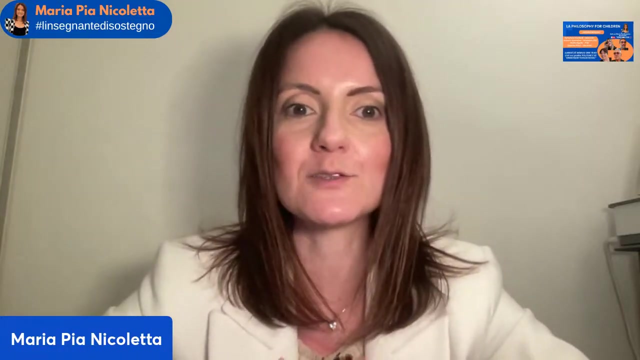 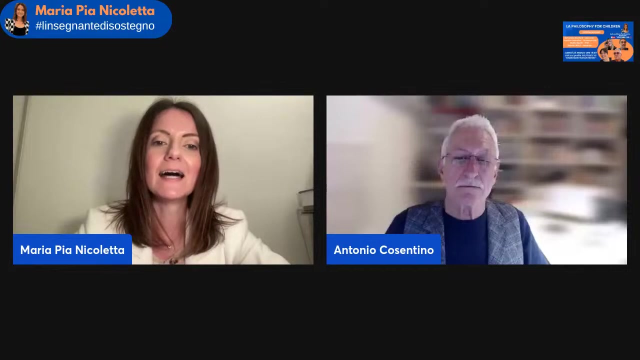 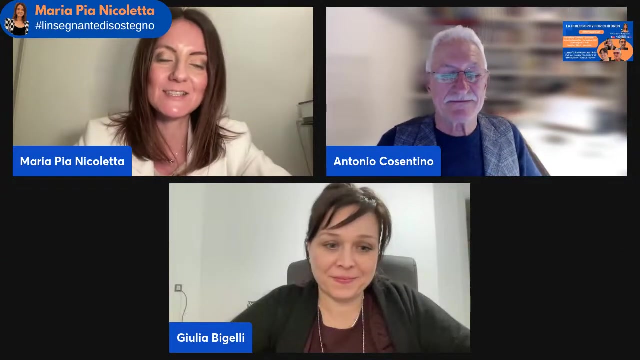 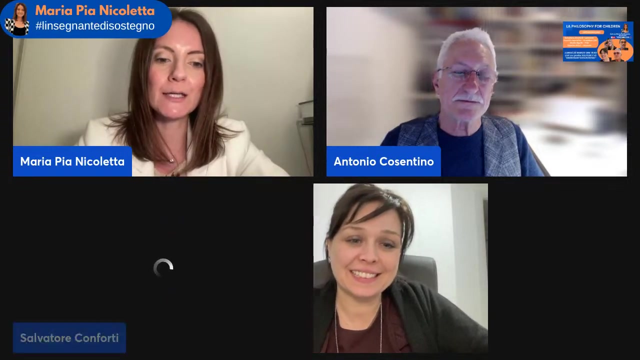 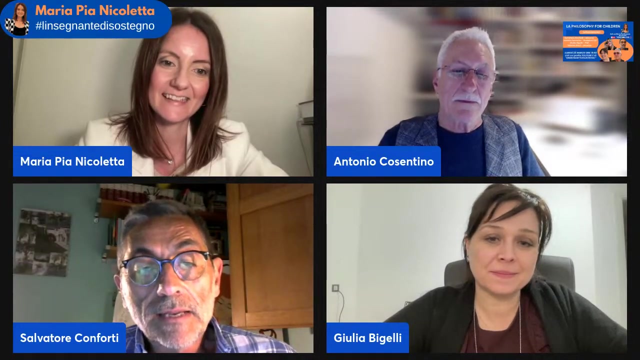 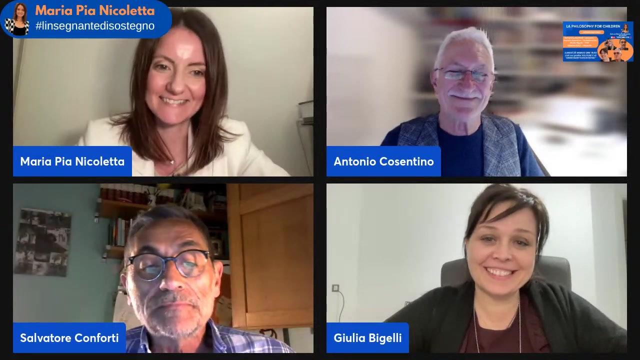 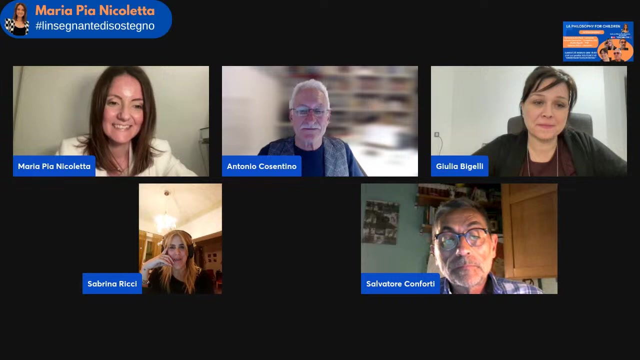 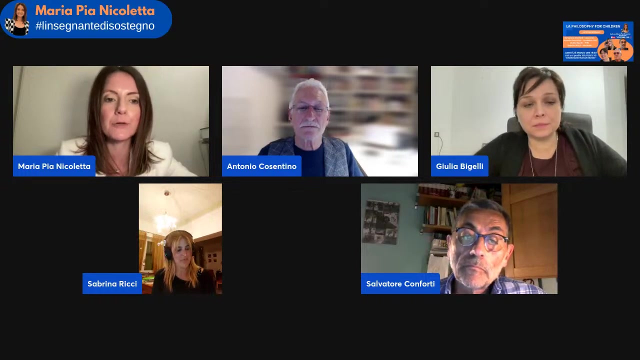 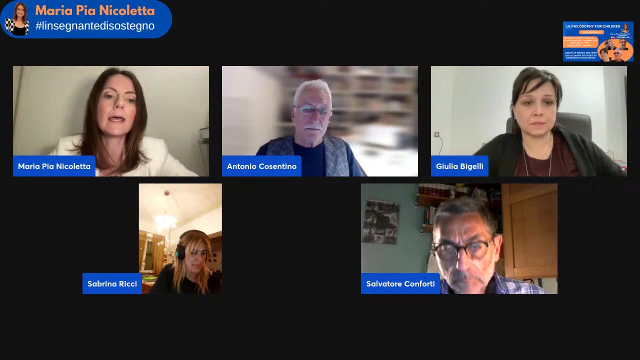 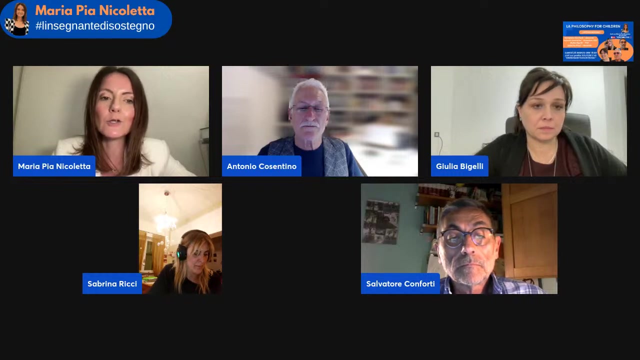 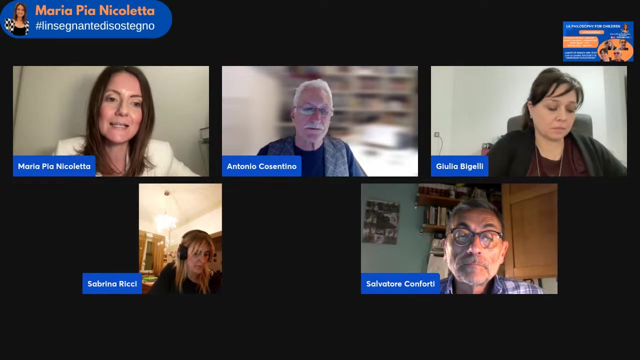 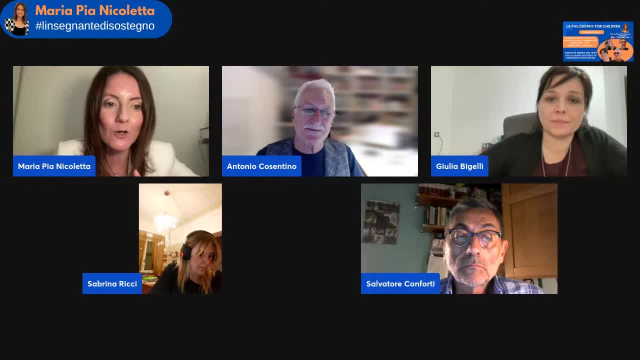 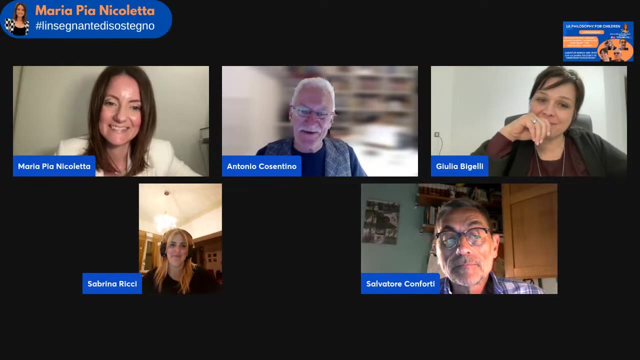 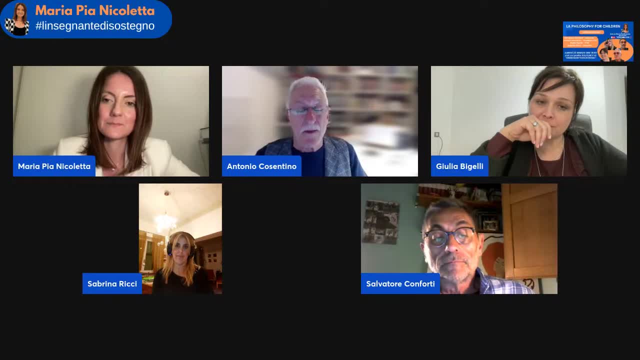 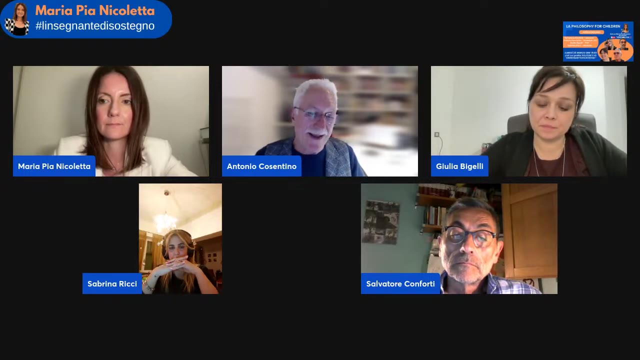 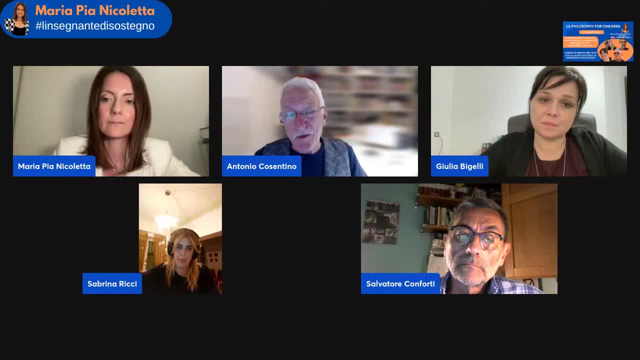 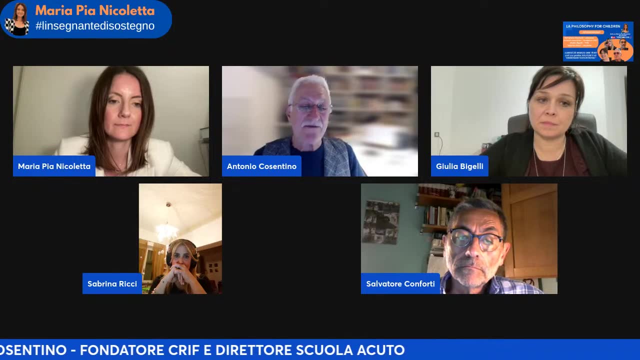 Thank you for watching della didattica, cioè preoccupato dal fatto che i ragazzi si li vedevo piuttosto annoiati e poco interessanti alla filastrocca, tale che ha detto che canta, detto che era simandro e platone, eccetera. 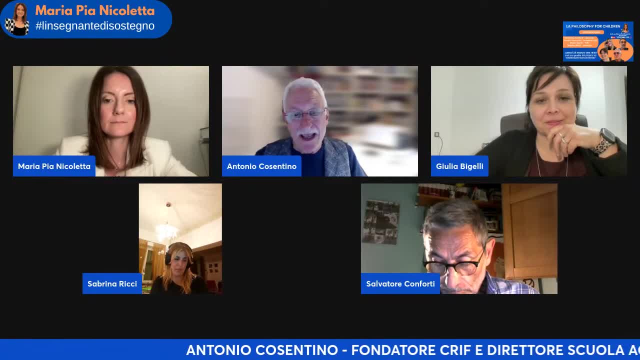 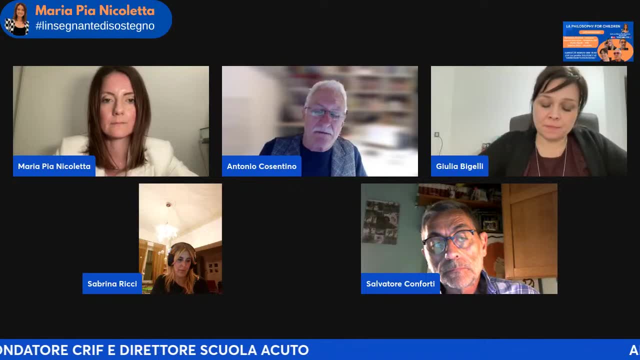 eccetera. questa filosofia come filastrocca delle opinioni era qualcosa che preoccupava non solo me, ma insomma un gruppo di insegnanti, per cui c'era un animato dibattito su questa questione. 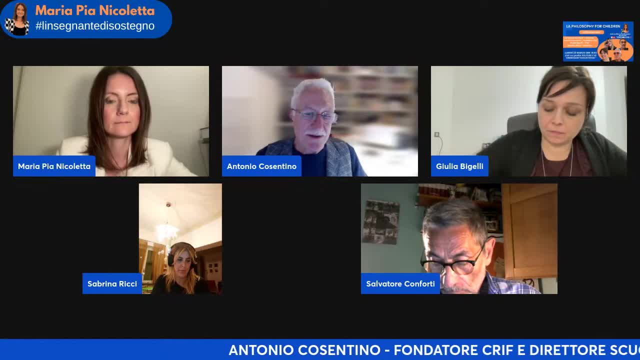 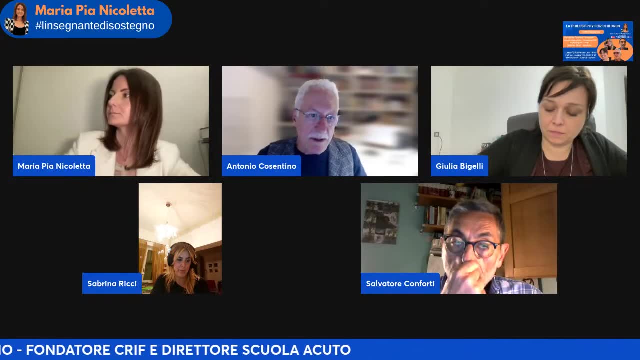 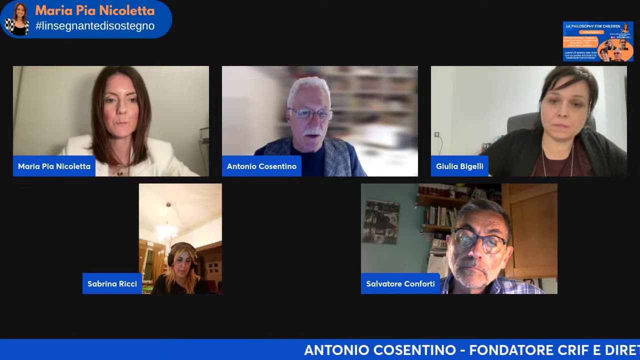 quando ha incontrato l'ip man. 1988 è stato pubblicato in italia un primo suo articolo e mi si è illuminato il mondo perché ho, ho visto lì quello che stavo cercando. non ho detto con parole precise, lucide, consapevoli e soprattutto con gente che partito così, poi però l'ho. 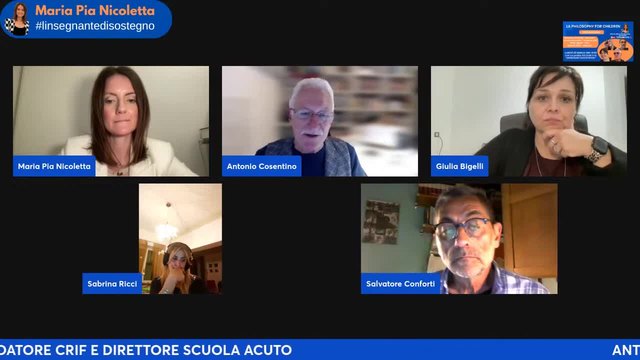 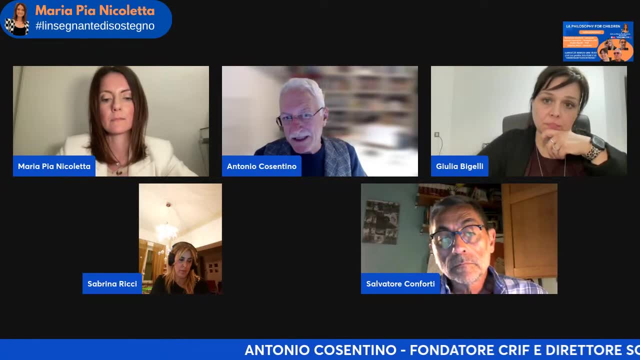 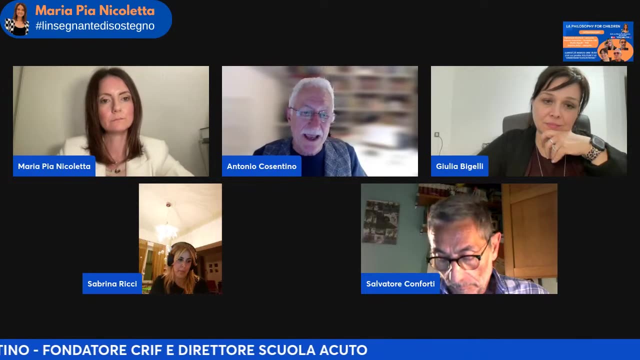 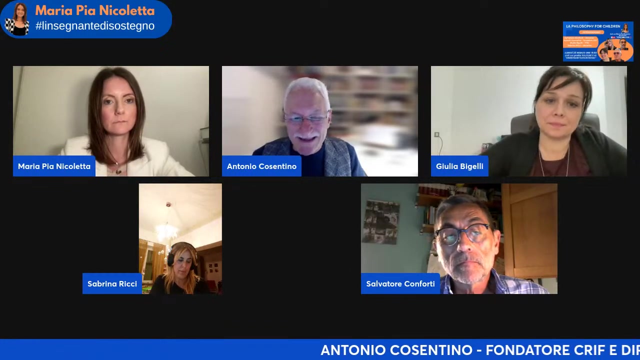 visto e ho capito che c'era anche molto altro. ecco, se saltiamo dagli inizi alla fine, quello che vedo adesso, quello che è comparso negli anni, anche attraverso le esperienze, e che si tratta, no, non di una didattica della filosofia, che non c'entrano quasi niente gli autori testi. 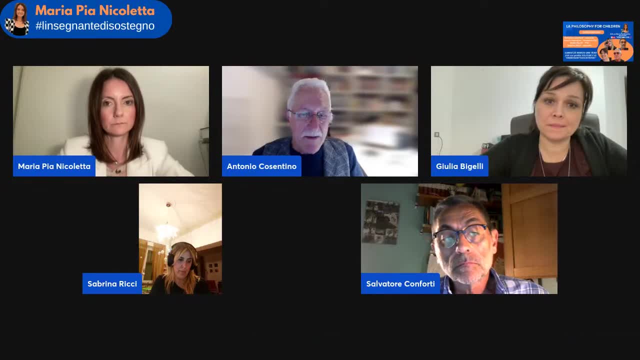 la storia della filosofia, quella che si insegnano, dice: ma c'entra molto una didattica generale, una didattica che io chiamo una didattica della comunità di ricerca. e la comunità di ricerca poi, se uno entra nel curriculum, capisce che è il soggetto principale, il fulcro su. 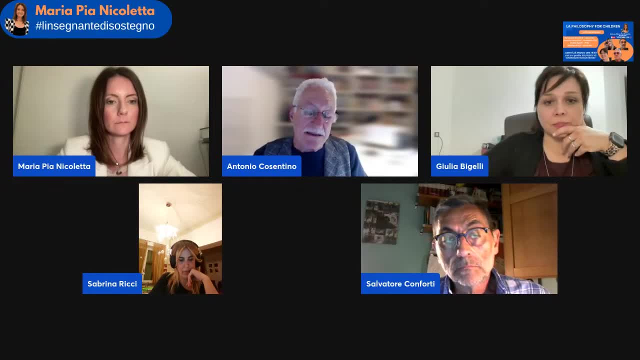 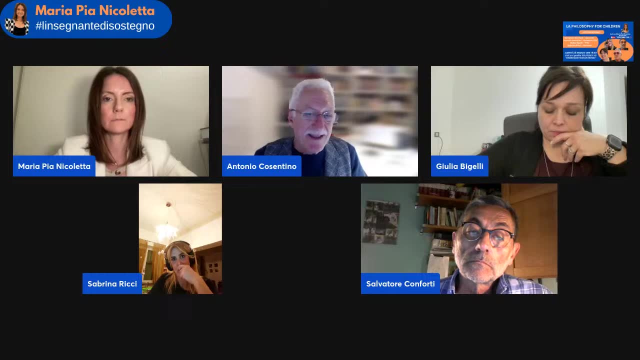 cui poggia un po' tutta l'imparcatura. la storia è stata quella di che ne so degli incoscienti, di quelli che in un'italia che ha questa tradizione, di quelli che in un'italia che ha questa tradizione, di quelli che in un'italia che ha questa tradizione. 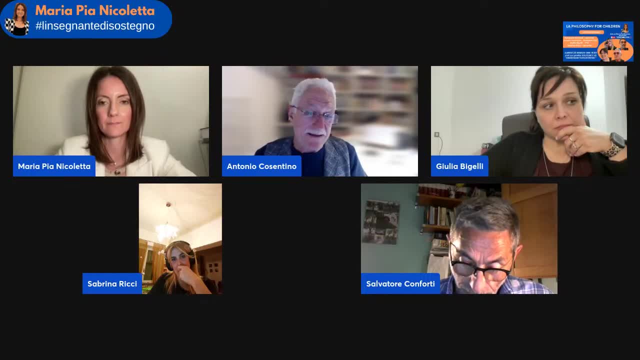 della filosofia orte, insomma anche dell'insegnamento della filosofia. abbiamo le spalle figure come gentile. e dire che la filosofia si poteva fare come una pratica sociale, come un esercizio di dialogo. 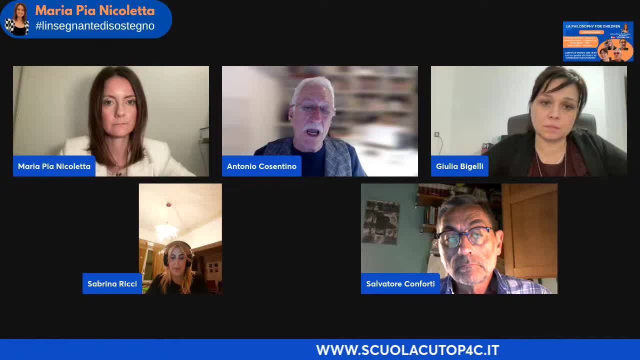 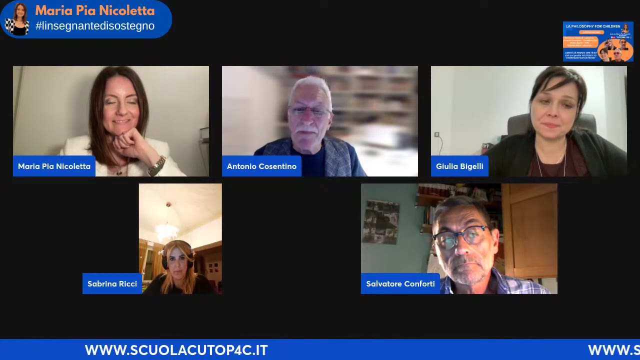 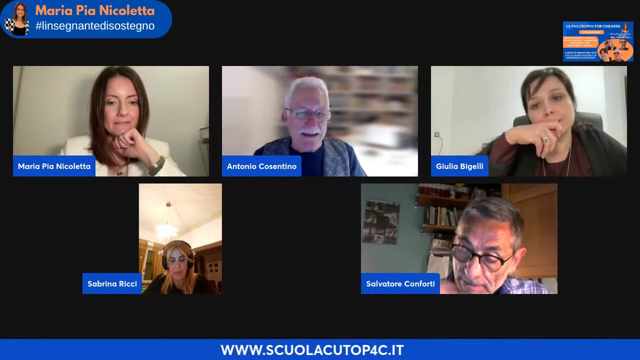 comunitario, seduti in cerchio anche con bambini di prima classe della scuola primaria. era una, era una sfida molto alta. insomma, però ecco, nel 1999, dopo che la notizia era un po circolata e qualcuno 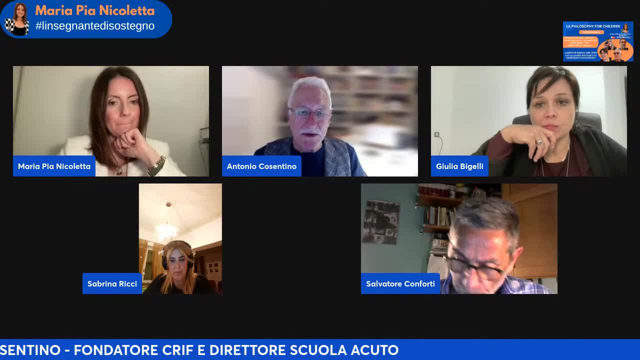 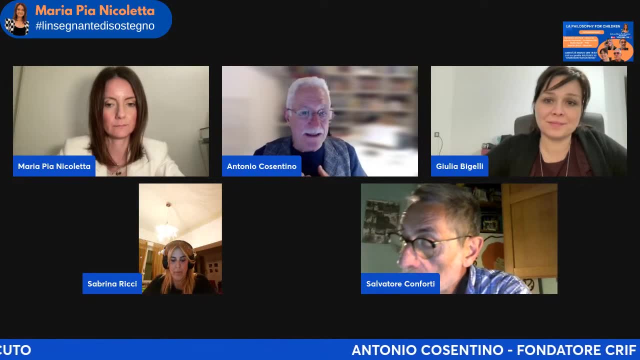 cominciava a saperne qualche cosa. io ho proposto un corso di formazione sulla modello di quello che io avevo frequentato nel new jersey, insomma lì nella montclair university, dove lippmann aveva il suo istituto. 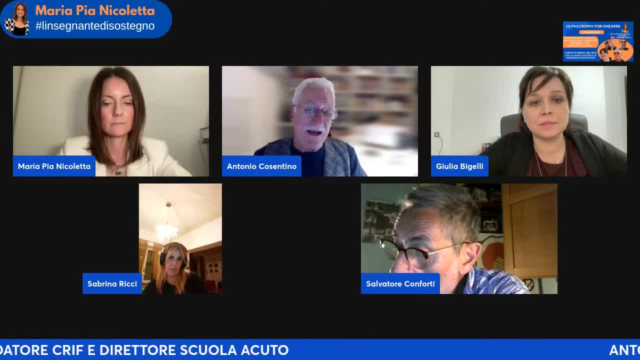 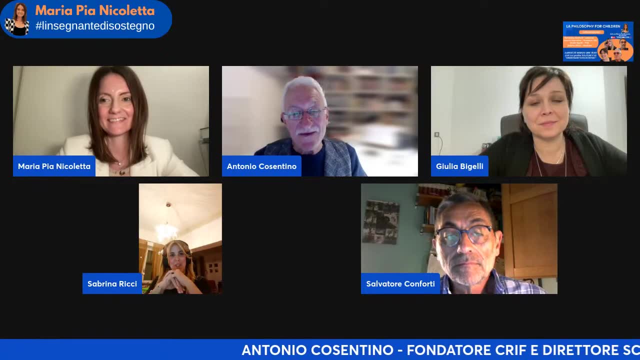 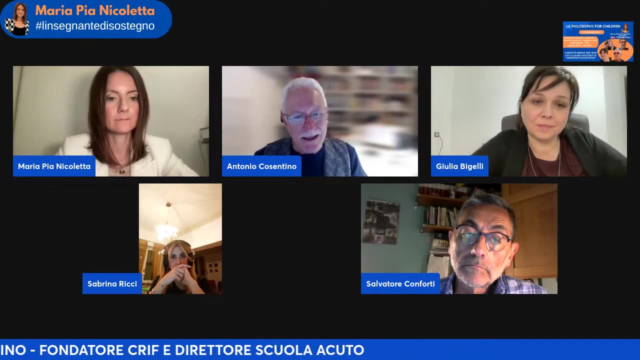 un corso residenziale, quella americana, di 14 giorni in un bosco, quindi in una situazione in cui tu vivi l'esperienza di costruzione di una comunità che succede, che quello che succede, che persone. 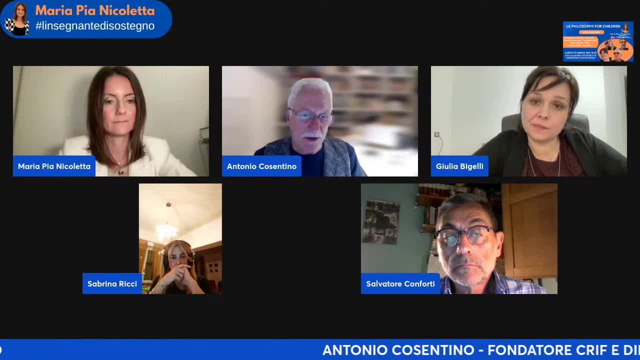 che arrivano il mondo, in quel caso, che non si conoscono, 14 giorni diventano una comunità, ma, devo anche sottolinearlo, è una comunità di ricerca, perché si può fare, si può formare una comunità in base. 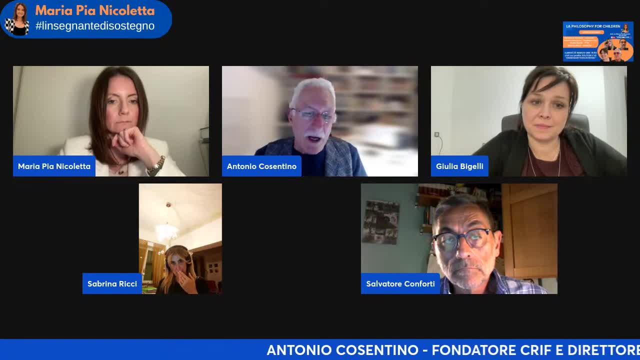 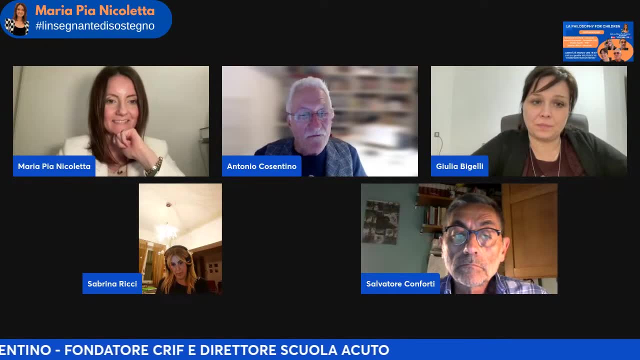 alla condivisione di tante cose. no, ci sono anche le comunità del calcio, la tifoseria, per non dire poi, tra l'altro, lì in america era- eravamo in un convento, un ex convento- quindi l'idea di comunità. 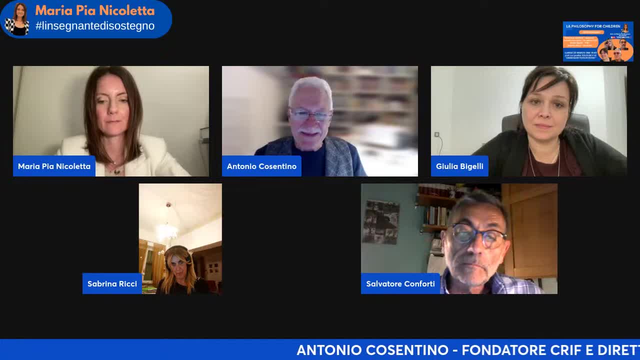 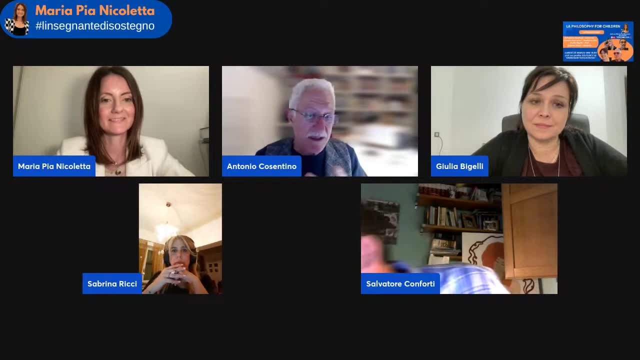 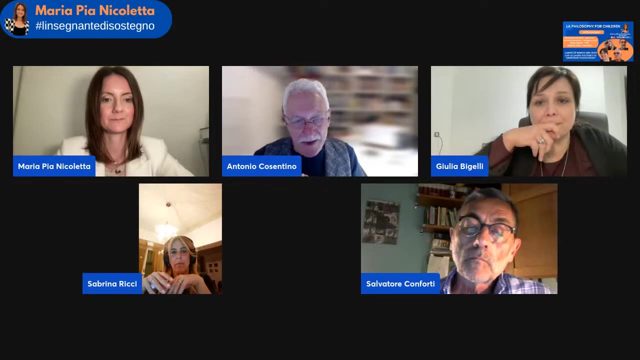 in qualche modo, ma era emanata un po da tutte, da tutto il luogo, dal posto di isolamento. insomma, nel 1999 ho proposto questo primo, questa prima, la prima volta, la prima edizione del corso che adesso quest'anno arriverà la ventisesima edizione sarà l'albano laziale. quell'anno eravamo a frascate. 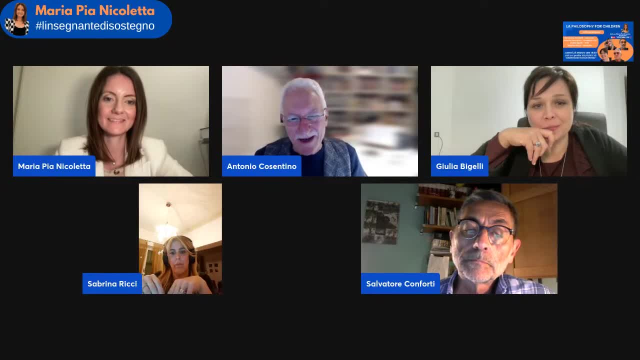 poi ci siamo trasferiti ad acuto. siamo rimasti lì per molti anni. ecco perché appunto, però adesso appunto significa animare comunità utopiche. è un omaggio anche al luogo, questo paesino, la cerceria, dove siamo stati per tanti anni. quest'anno sarà. 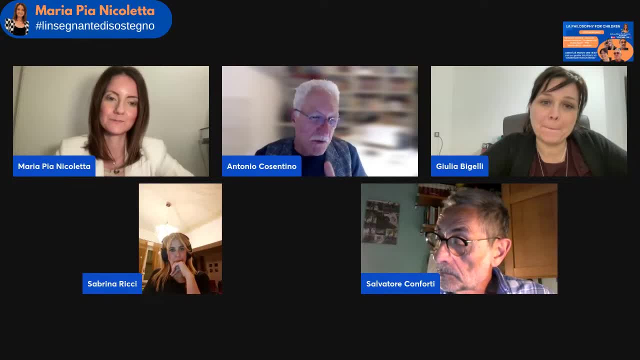 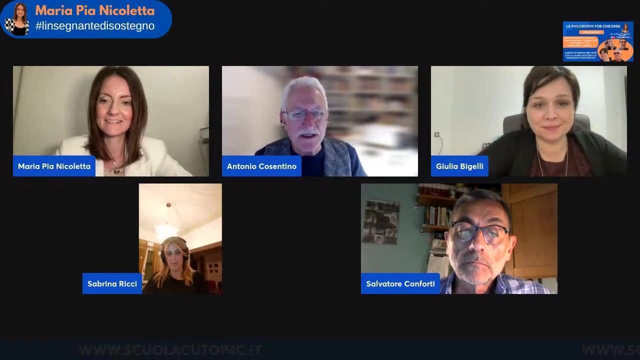 la banca. insomma, questo corso era una sfida. non verrà nessuno, mi sono detto, saremo in tre o quattro. invece sono arrivate 32 persone. c'era dirigenti scolastici, insegnanti, anche ricercatori universitari. 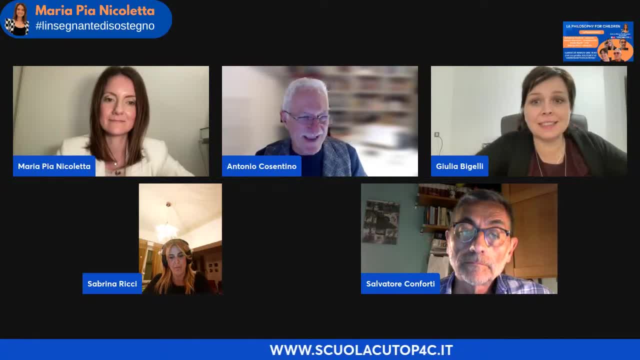 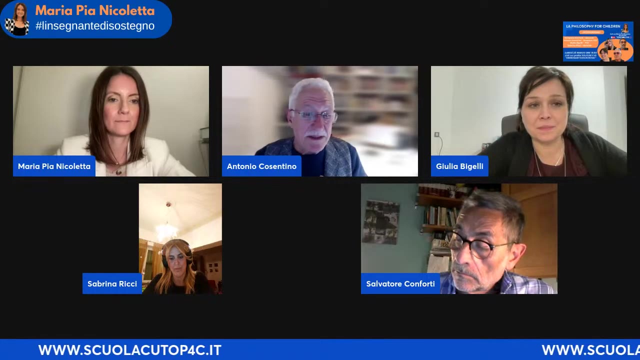 di qualora si può fare. e siamo partiti già eravamo partiti un po con maura, stiano come rena santa tradurre il curriculum. abbiamo trovato questo editore coraggioso che liguori, che l'ha pubblicato, e siamo partiti con. 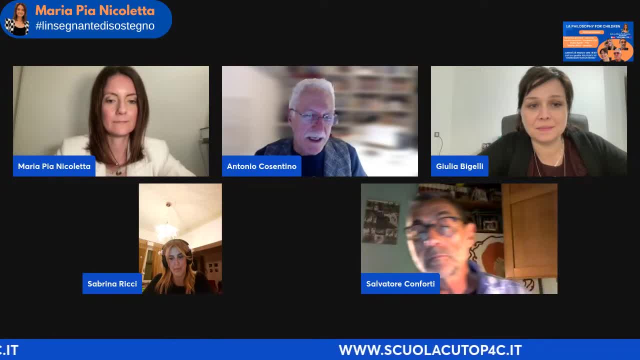 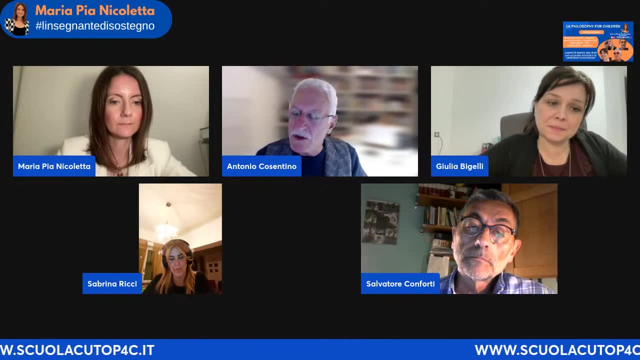 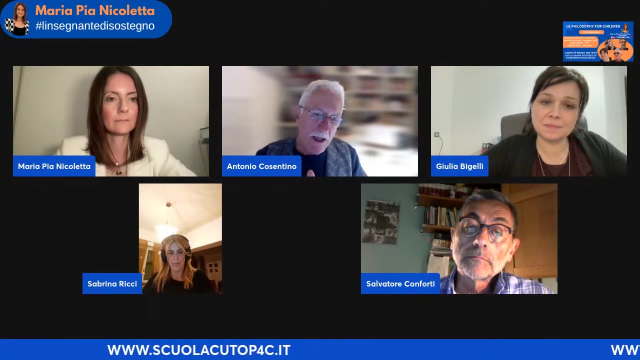 la formazione di insegnanti con la traduzione alla ricerca, la sperimentazione sono questo successo. adesso ancora per tornare verso, per dirigere lo sguardo verso la fine della storia, negli anni. e la scuola, la voce è filosofica, con bambini trova una montagna di cose. quindi uno dice: è fatta ce. 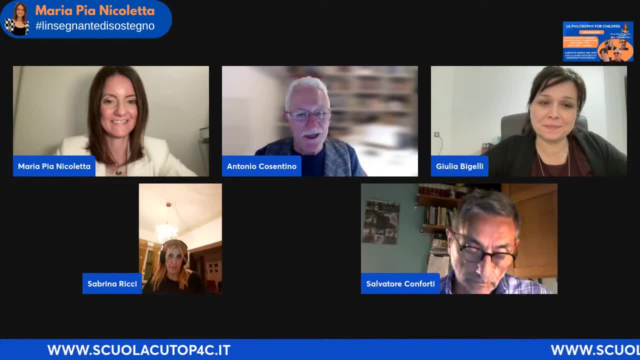 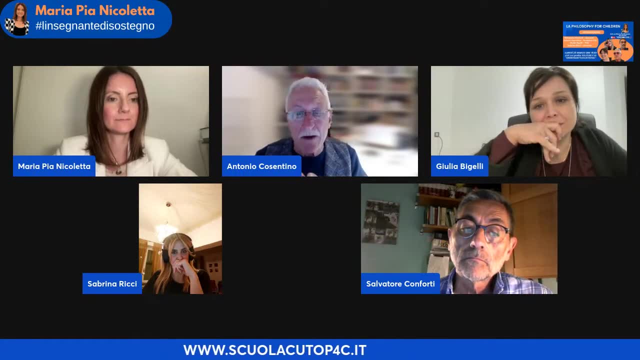 l'abbiamo fatta, cioè siamo riusciti a farla, a diffondere questo, questo progetto, a farlo conoscere, anche discutere, insomma anche criticare, perché no? però devo dire una cosa: che le apparenze 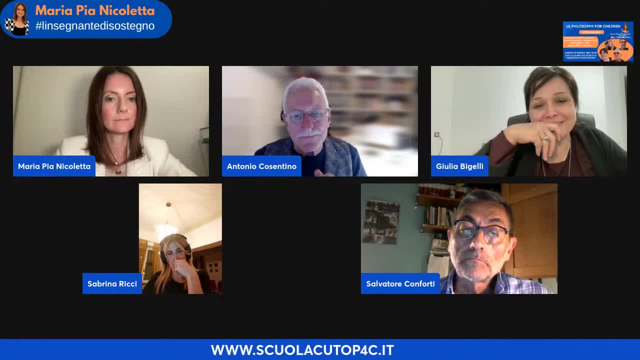 in questo caso di un po in gamma, cioè è vero che se ne parliamo tanto, se ne parla un po dappertutto, è vero che ci sono, ogni anno noi facciamo il cristo, bandisce un concorso per le tesi di laurea e ce ne sono tantissimi, quindi anche nelle università da. 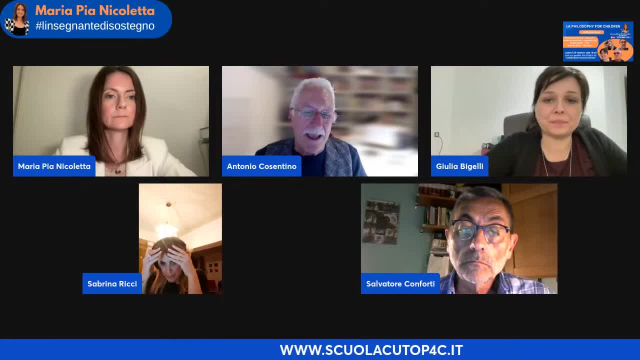 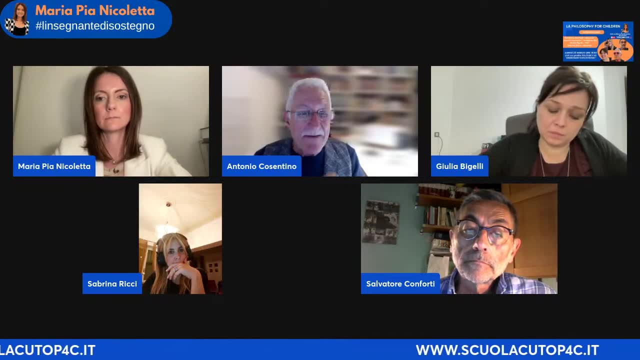 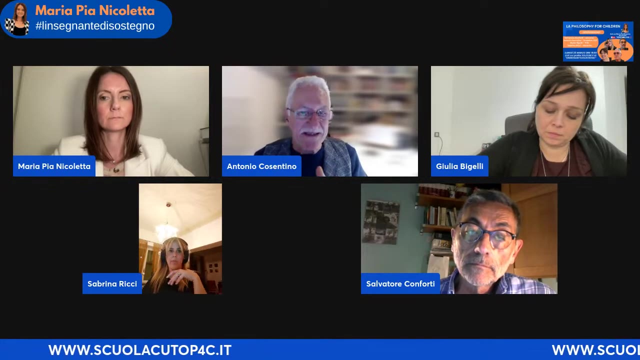 cassino, a padova, a napoli è conosciuta, a verona dove io tengo un laboratorio, insomma, è penetrata. però se andiamo a vedere quante scuole in italia la offrono come esperienza di formazione ed educazione dei bambini, ne troviamo poche. rispetto a questo c'è una. 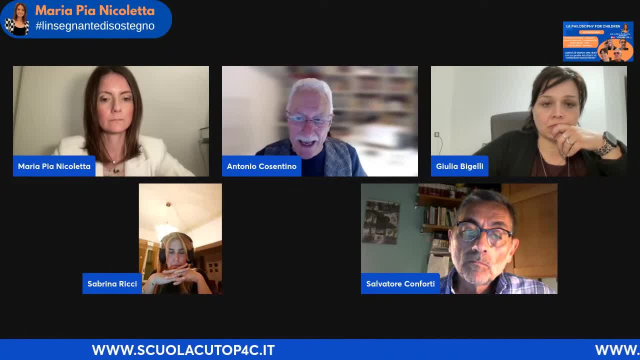 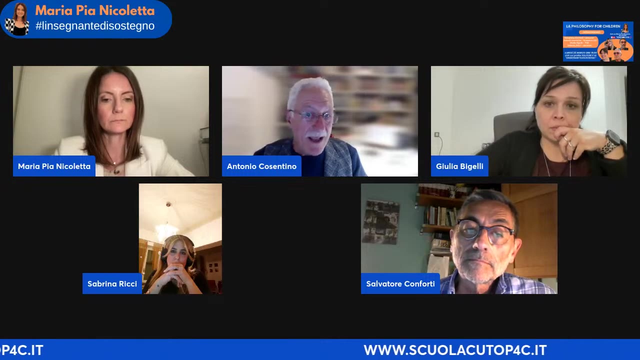 sproporzione. quindi c'è una domanda anche perché non entra in modo così massiccio nelle scuole ed è una questione culturale, istituzionale, politica ovviamente. insomma, è una questione aperta. la 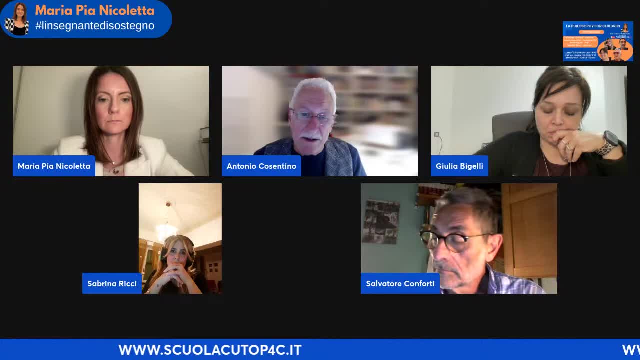 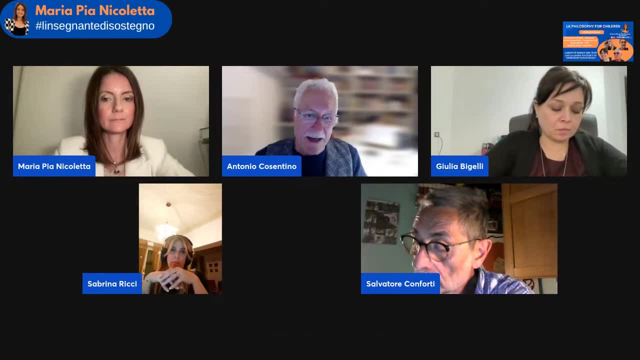 questione aperta. noi continuiamo la nostra battaglia perché siamo convinti che è una proposta in quanto didattica generale. è una proposta che può entrare in tutte le classi, può interessare anche le discipline specifiche, la matematica, storico e non. 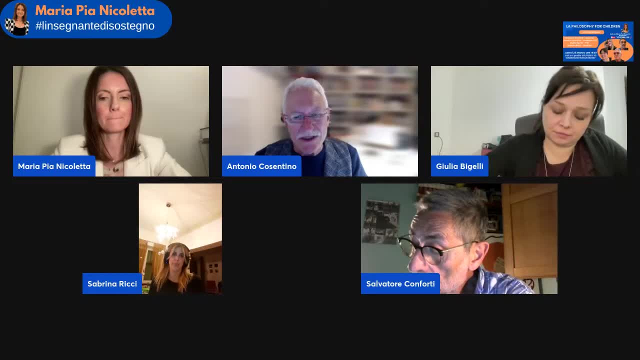 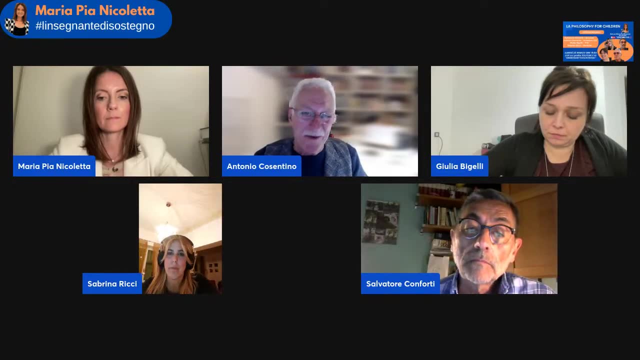 soltanto un esercizio che filosofico, perché non è disciplinare, interdisciplinare, se vogliamo. però, come si fa poi con questo? è tutta una cosa che si deve dire a parte, ma fermerei qua. 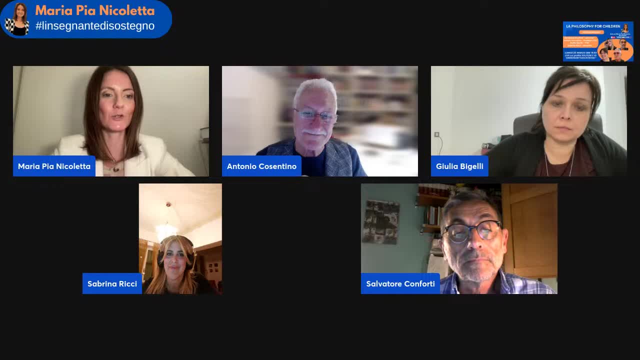 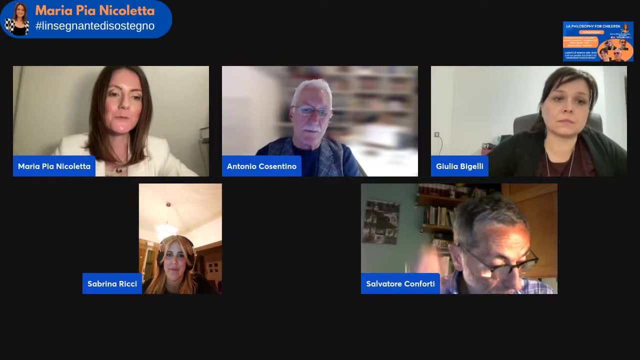 grazie, grazie mille, antonio. magari dopo vedremo qualche tua pubblicazione. lancerò le immagini di alcuni dei tuoi testi. io passerei in questo momento la parola alla dottoressa giulia bigelli. lei è una. 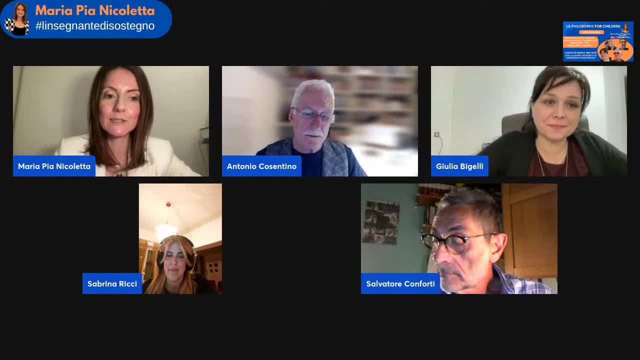 ricercatrice di in didattica generale. correggimi, giulia, se faccio errori. siamo conosciute. ciao giulia, ben arrivata. io innanzitutto ci terrei a precisare una cosa: che, quando si ha a che fare con i propri follower, 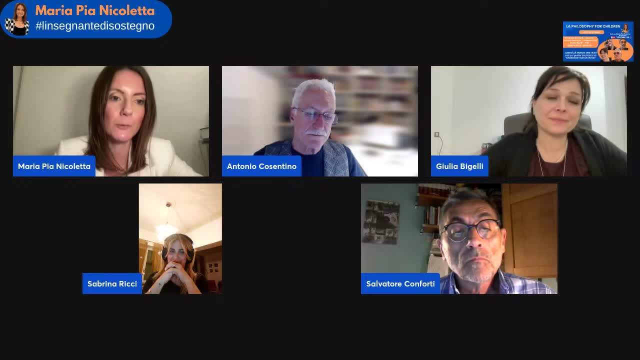 anche se non mi piace chiamarli così, perché dietro non sono numeri, sono persone. con giulia abbiamo iniziato proprio discutendo a seguito della pubblicazione di un mio post sulla filosofi for children, e abbiamo iniziato a disquisire su cosa fosse giusto riportare. no, lei ne sapeva più. 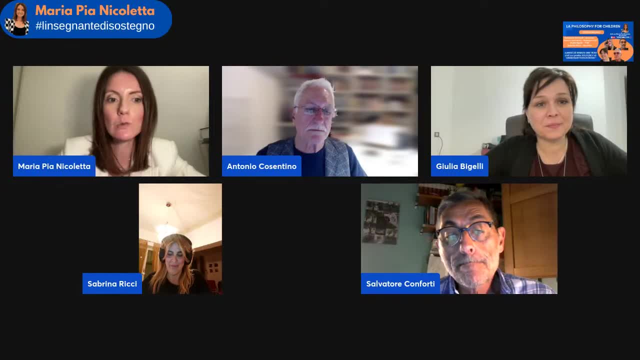 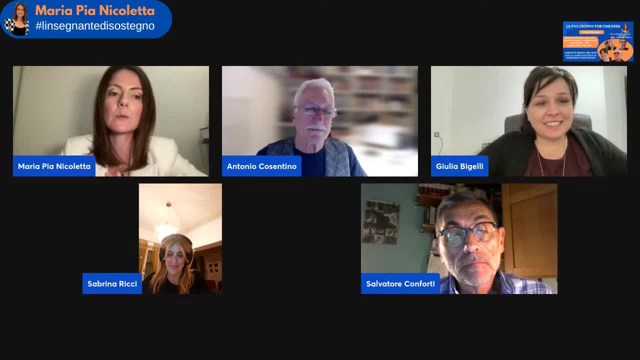 sofi col cidrani, perché teniamo dalle tue labbra. e quindi, giulia, raccontaci un po di te: quale è la tua formazione, è di cosa ti occupi e cosa ci vuoi dire rispetto alla filosofia. porci, brenna, allora. 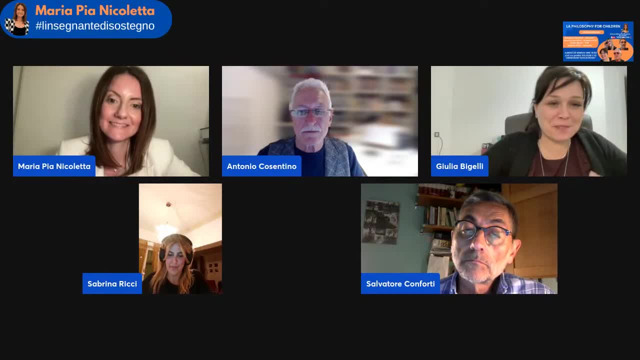 è vero, maria via fun. uno scambio di opinioni, di punti di vista molto coniche, poi ha portato no a qualcosa di molto bello. eccoci qui, allora. io sono un po la testimonianza di quello che antonio, which Antonio has talked about so far, because I participated in one of the editions of the 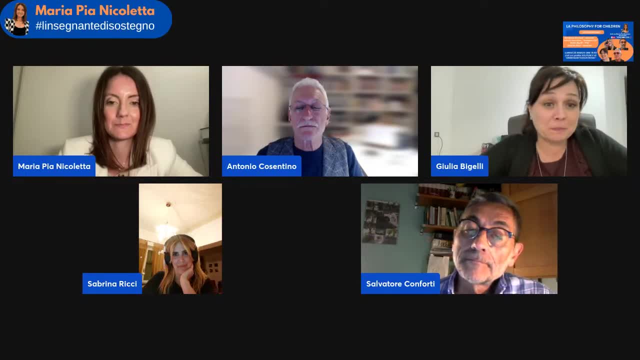 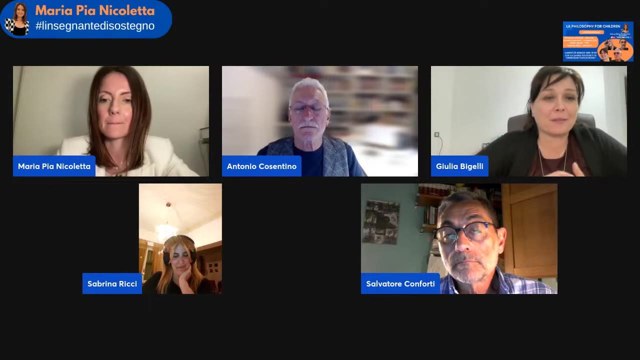 high school in 2009,. I had recently graduated in philosophy and I was also a bit looking for something that, how to say, would respond to a perhaps more to a need, to a curiosity. I say, ok, beautiful, this degree in philosophy has been wonderful for me. it was really a. 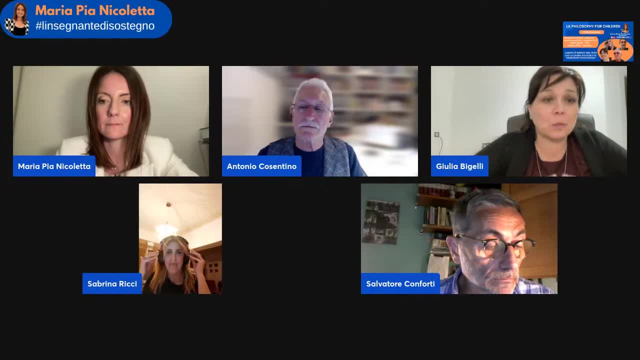 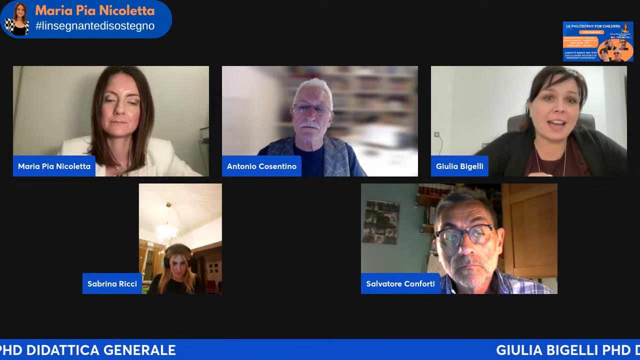 path. it was an enlightening path, a motivating one, but in the end, what do we do today with philosophy? And I also started looking and little by little, I began to approach myself with the world of philosophical practices. so I also tried the philosophy counseling school. 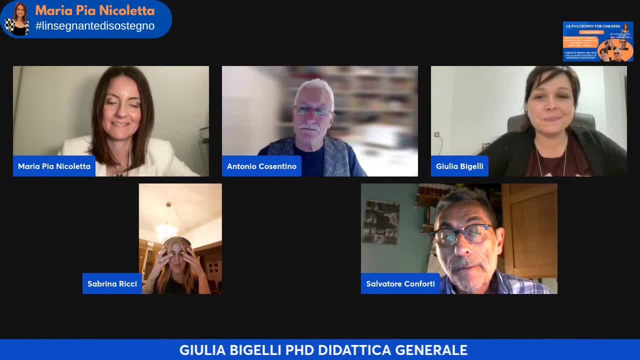 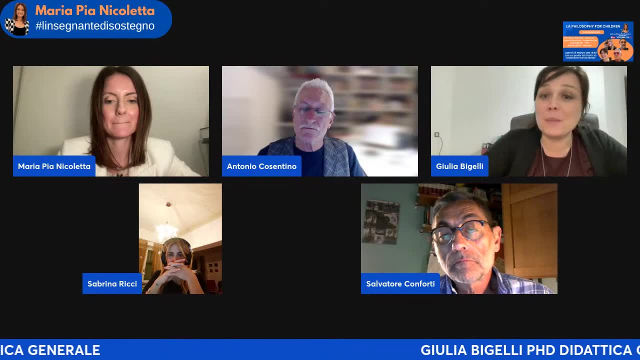 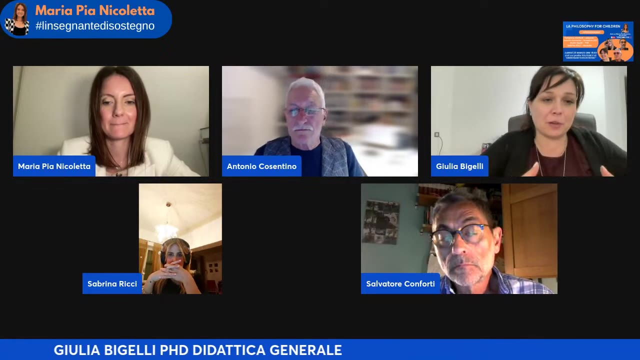 but there was something that did not do for me. it was not. it did not fully convince me and, continuing to look, I started to frequent this world. I met philosophy for children, As Antonio says. even at that time, there were many proposals for philosophy for children, among other things, I was already working in the world of 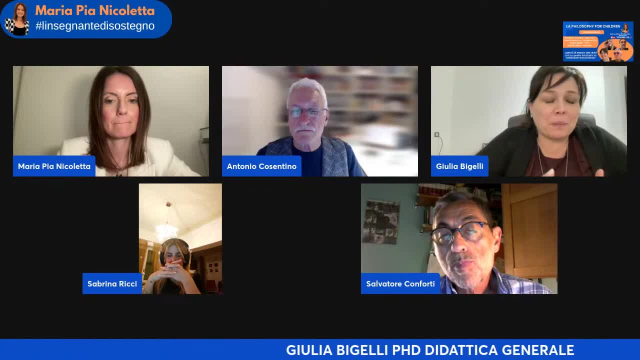 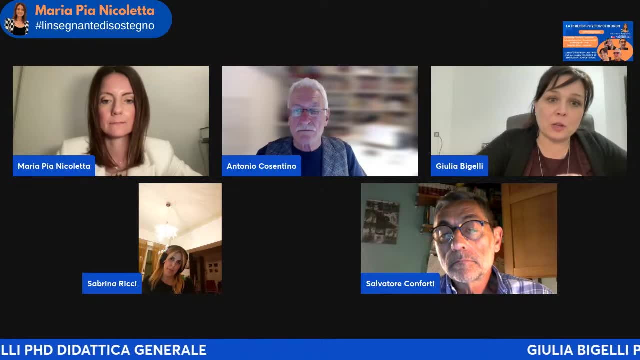 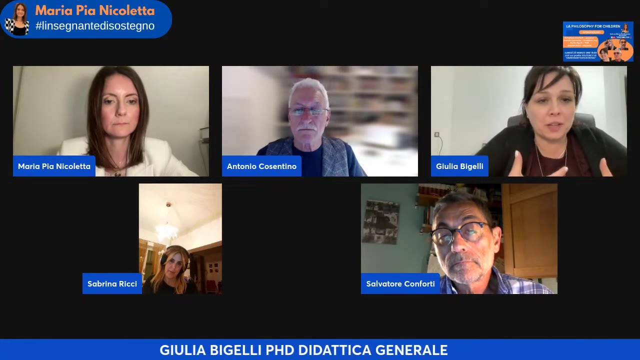 childhood, but in another field. so it was for me, in short, something new, something stimulating to investigate. I chose to focus on philosophy for children, why? Because it was the one that had a foundation behind it, that is, there was something that 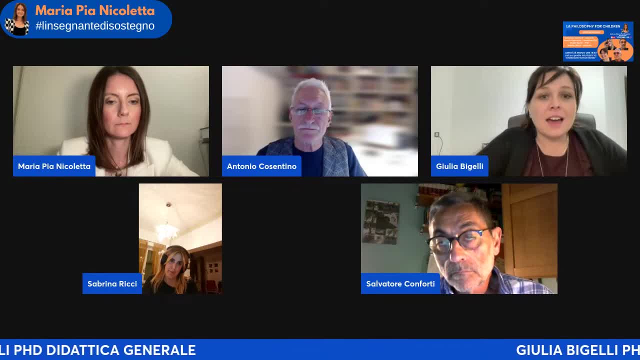 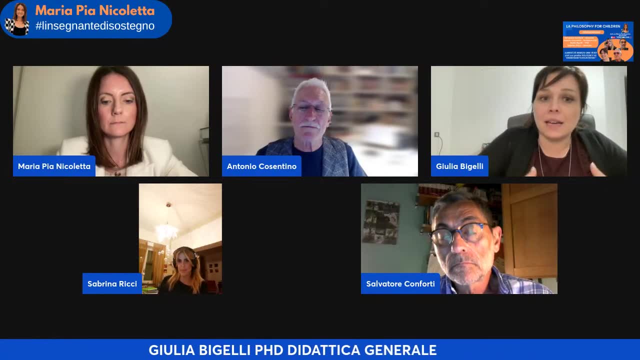 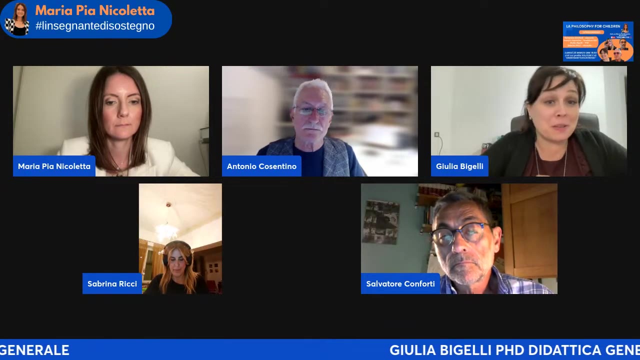 upsets me because there was a beautiful history, an extraordinary history. but there was also something that increase me and I said, ok, but it's true, it's not a chat, but we have a curriculum to follow, we have- how should I say- so-so important theoretical bases, and so I arrived. 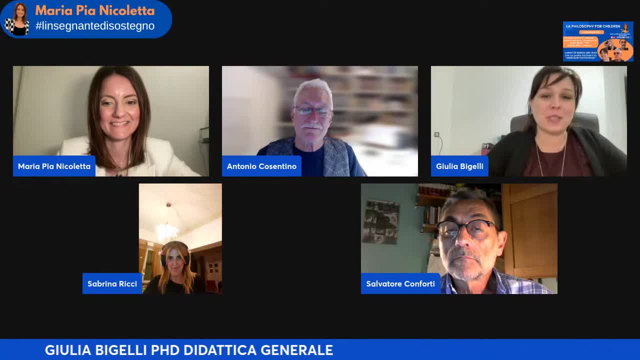 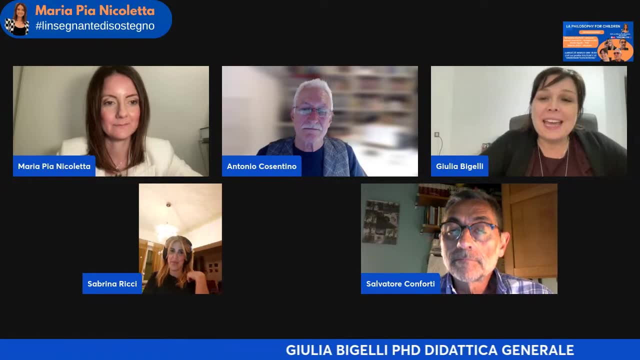 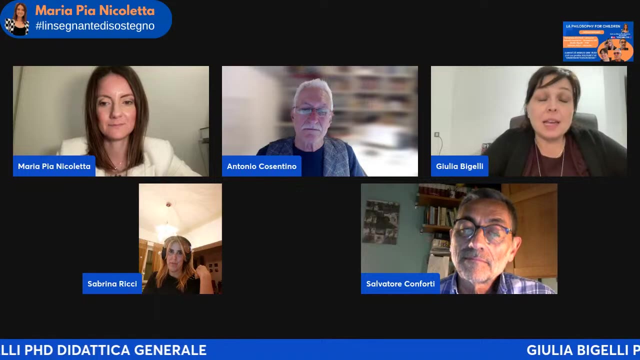 precisely at the school, at the highest, It was 10 wonderful days- I confirm what Antonio- su praticamente tutto il giorno. e quindi c'era modo, davvero no, di di esperire quello che poi io iniziavo a studiare, e fu un percorso, un percorso intenso, un percorso intenso prima. 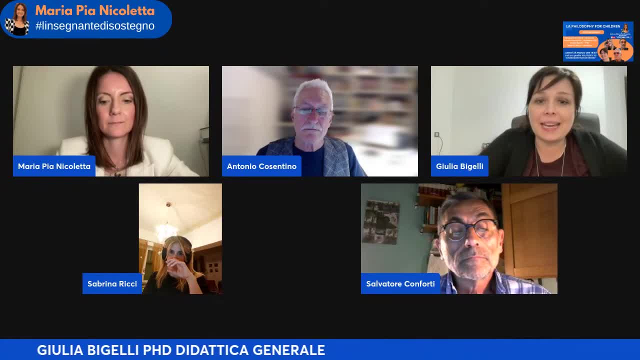 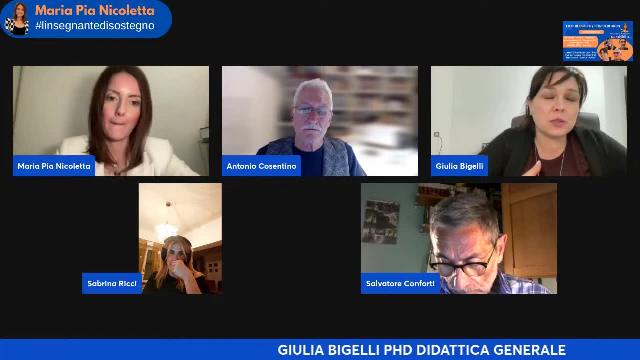 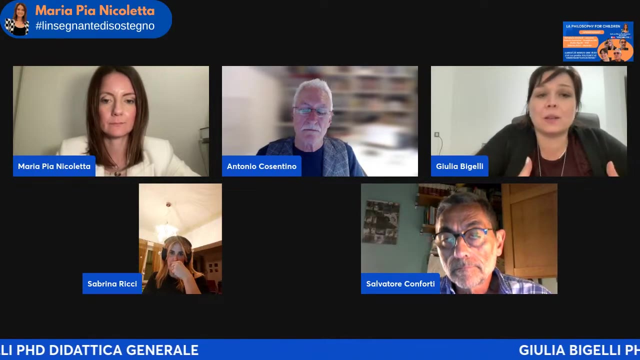 di tutto, per per me, perché? perché capisci quanto praticare la filosofia in un certo modo va, in un certo modo va a smuovere davvero delle competenze, delle dei talenti, delle delle abilità che non che mai avrei pensato, devo essere sincera. e quindi ecco, la scuola di acuto furono. 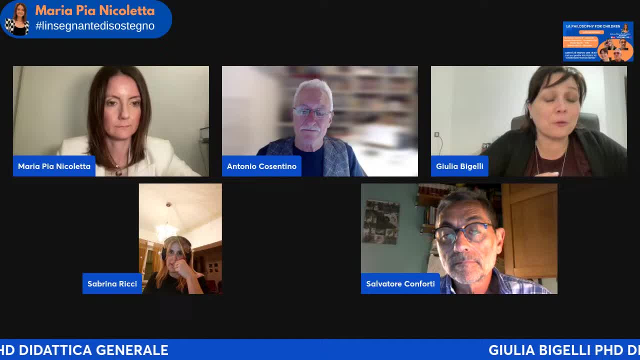 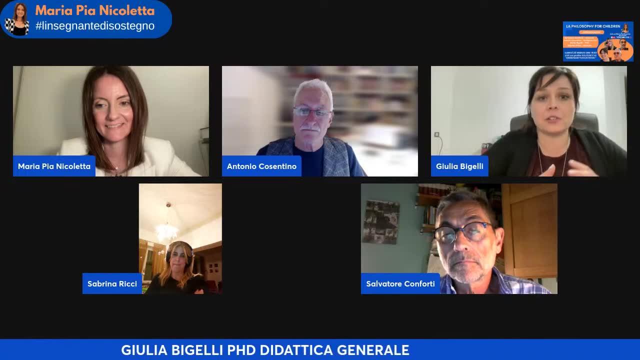 dieci giorni veramente toccanti, formativi, anche perché poi, ecco, era organizzata. c'erano dei momenti tanta pratica, ma c'erano anche dei momenti di teoria. sono dei momenti di riflessione. poi c'erano: 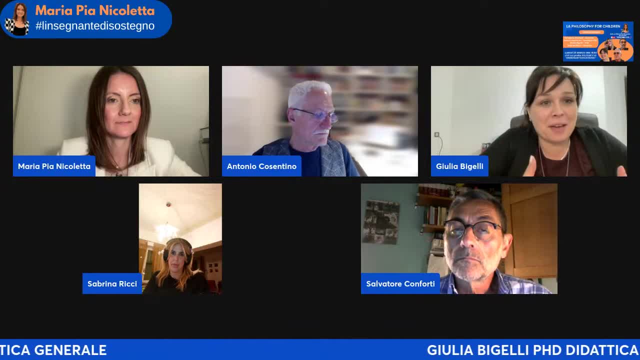 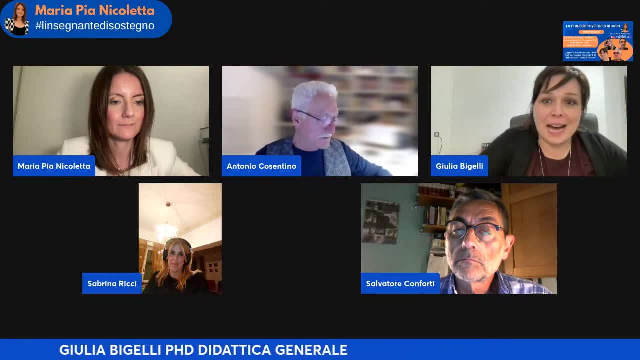 come dire anche serate, no, in cui si stava tutti insieme. e lì, ecco, vedevi proprio come, come dire, questa pratica filosofica poi in realtà smuoveva anche le abilità sociali, smuovevano il saper fare. 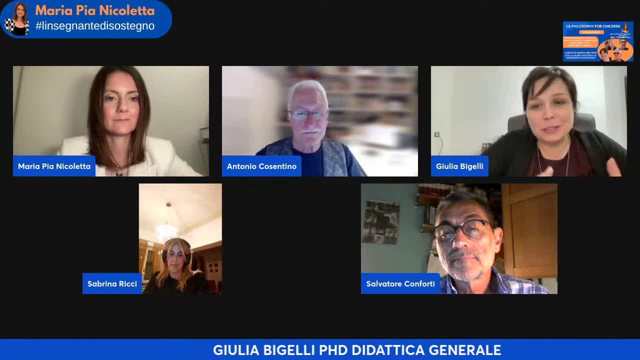 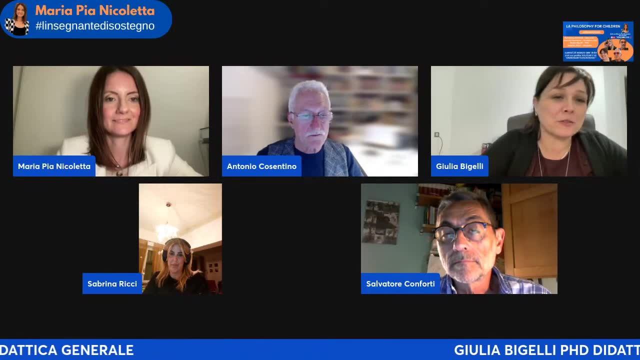 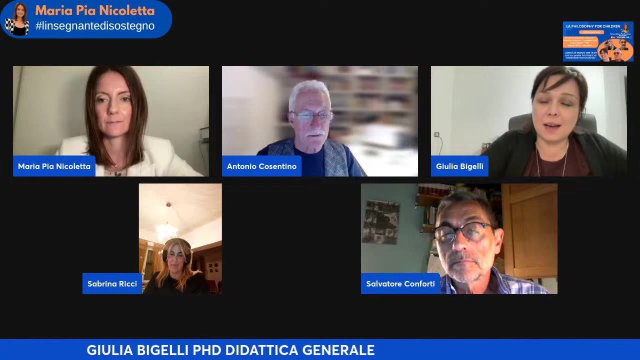 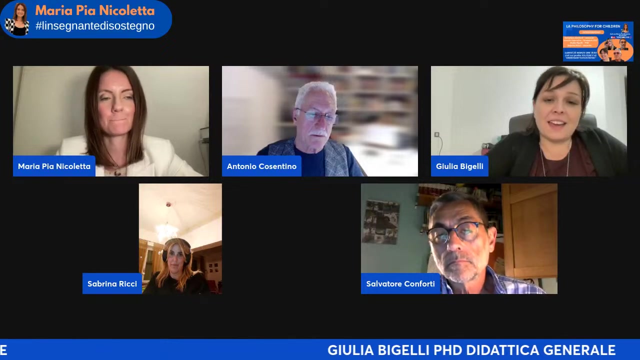 rete e dopo qualche io ho continuato poi nella ricerca. dopo qualche anno provai un dottorato, ma avevo capito che non era più la filosofia sola non mi bastava e quindi ho iniziato a- come dire, a studiare in maniera più, in maniera più profonda il campo dell'educazione. ci fu chi? 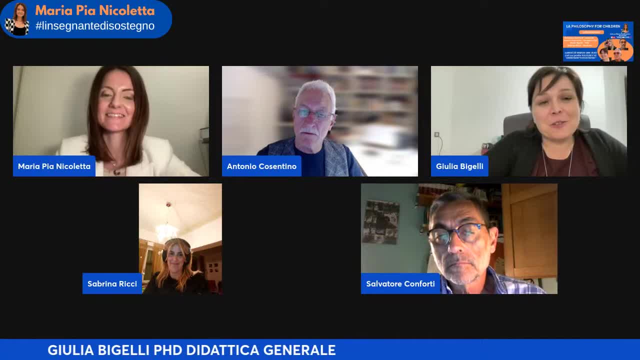 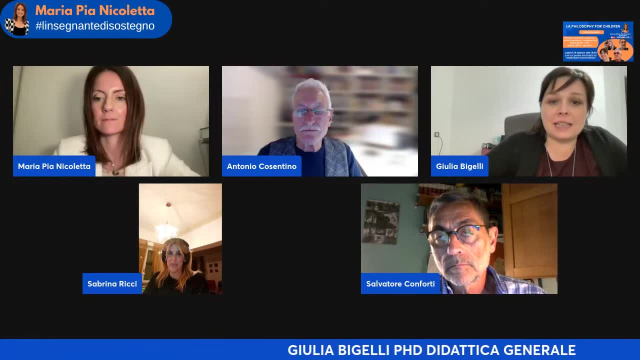 diede fiducia al mio progetto di ricerca. quindi nel 2013 inizia il dottorato di ricerca, la l'unsa. e quelli furono anni altrettanto illuminanti per me, perché? perché lì c'è stato proprio il passaggio. 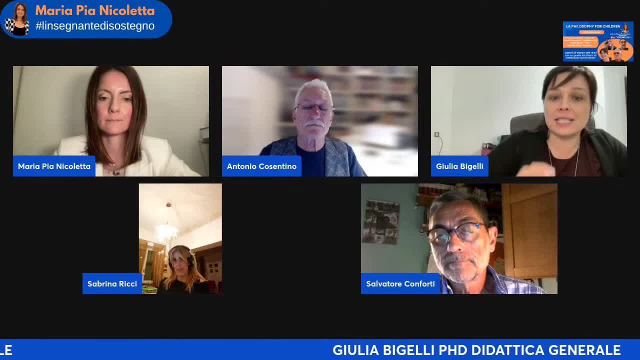 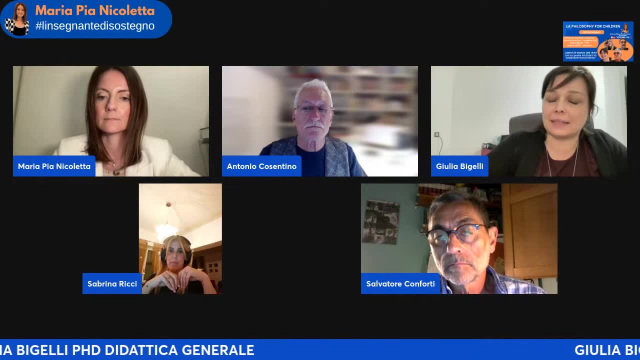 la pratica filosofica poteva davvero essere una strategia didattica e in particolare io, in quegli anni iniziai a studiare come la pratica filosofica attraverso la costruzione della comunità di. 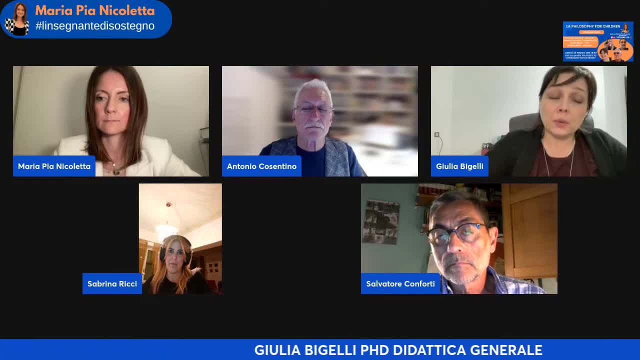 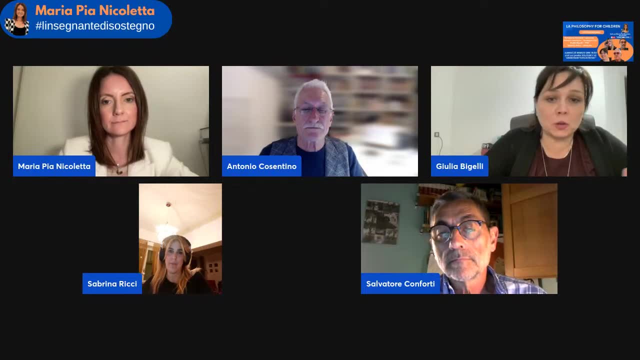 ricerca, la, la nascita della comunità di ricerca poteva essere considerata una strategia didattica di apprendimento cooperativo. d'altronde, c'erano, ci sono tutti, no? gli elementi tipici. c'è l'interdipendenza positiva, c'è una leadership distribuita, c'è 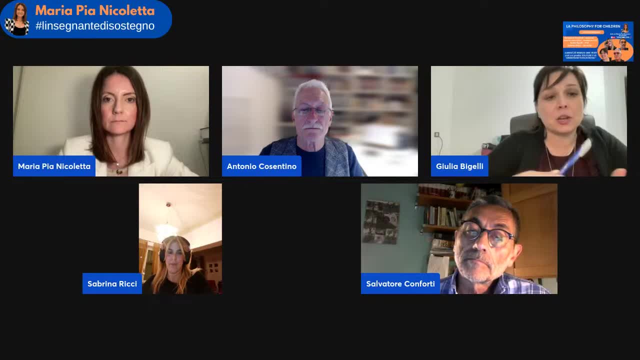 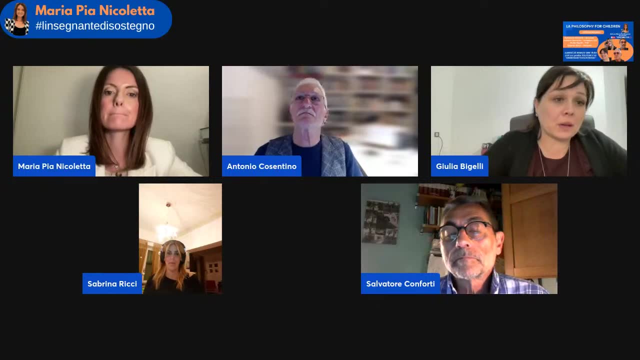 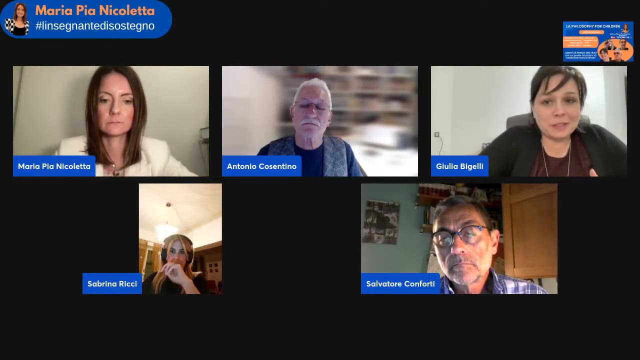 una valutazione nitinere, c'è un autovalutazione e c'è una valutazione finale ok, in una pratica di philosophy for children. e quindi ecco, nel mio percorso di ricerca cercai proprio sia da un punto di vista teorico e sia da un punto di vista in pratica. quindi feci tantissime ore in classe. 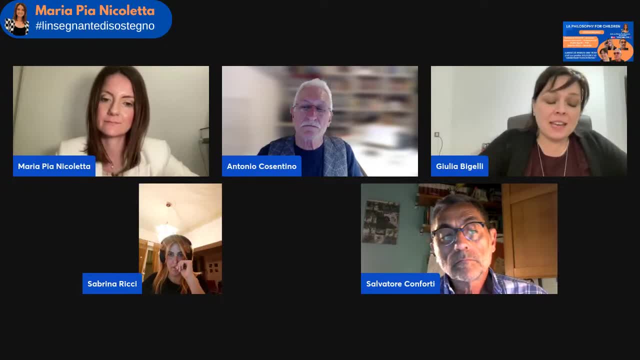 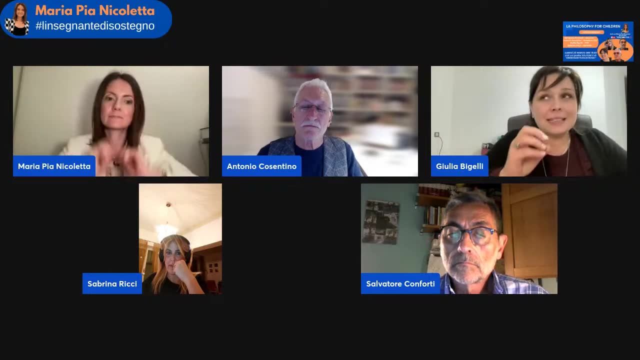 con i bambini, feci molta osservazione, registrai tantissimo tutte le sessioni, che, insomma, che I was attentive to the words that each of them used and I was able to see how their ability to ask questions during the sessions changed completely. 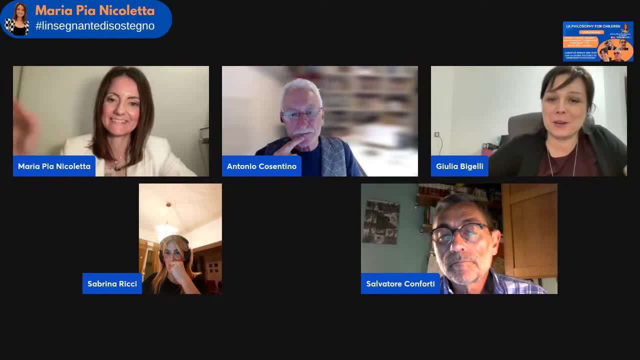 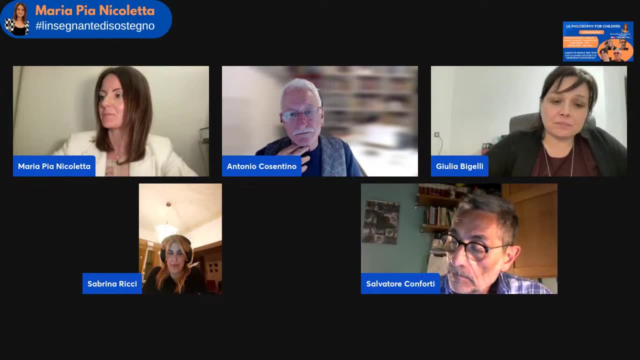 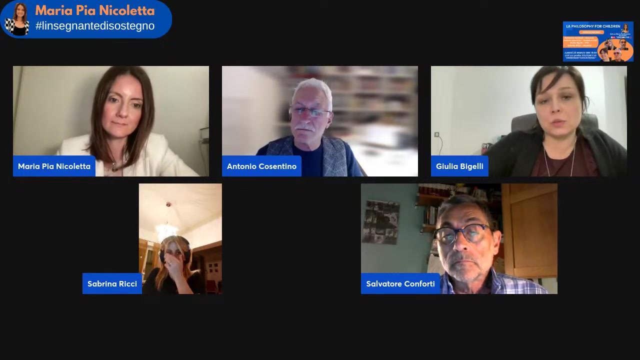 Salvatore will surely tell us even better than me about all this. So from there I started to study the cooperative and meta-cooperative character of Philosophy for Children. Why? Because, from a didactic point of view, Philosophy for Children is also a metacognition tool. 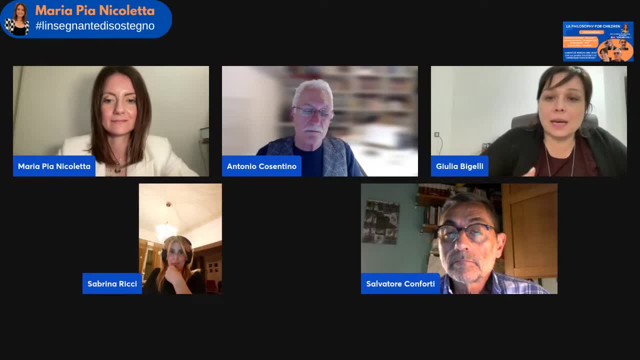 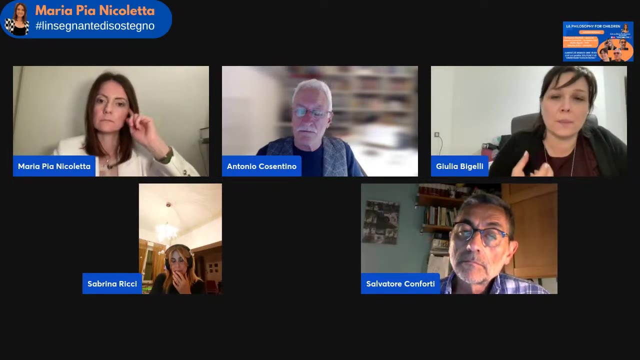 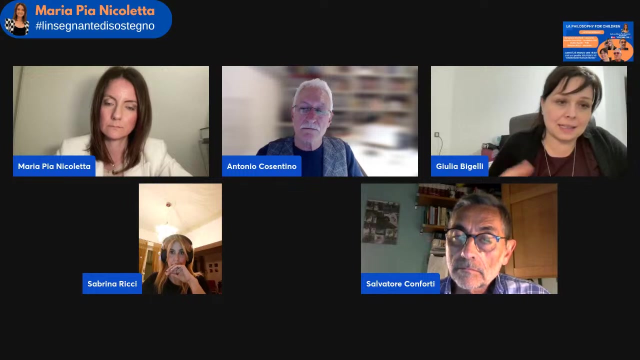 Why? Because it invites us, It invites children to consolidate all those to make the self-reflection thought even stronger. So how am I learning? How does my thought work? In the final part we ask ourselves this And then. another fundamental element is precisely the whole emotional valuable field that there is in Philosophy for Children. 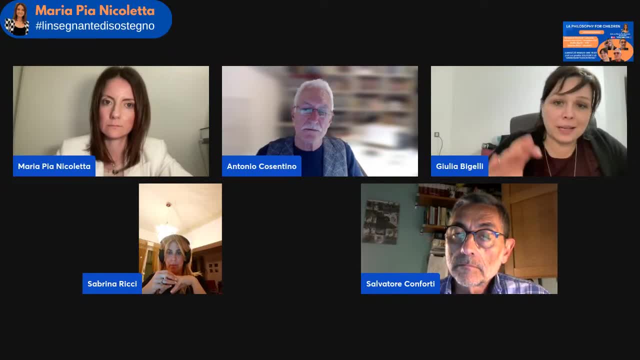 And then another fundamental element is precisely the whole emotional valuable field that there is in Philosophy for Children. And then another fundamental element is precisely the whole emotional valuable field that there is in Philosophy for Children. My research in those years where it stopped, it stopped at the time of evaluation. 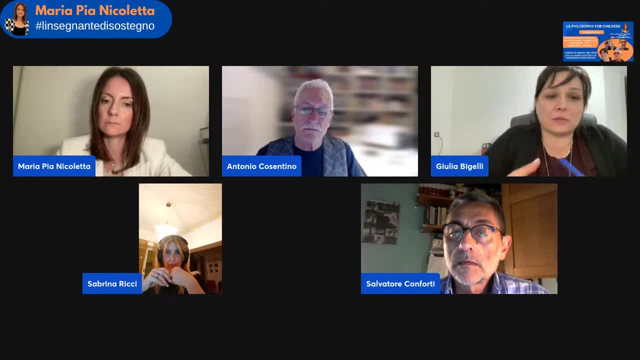 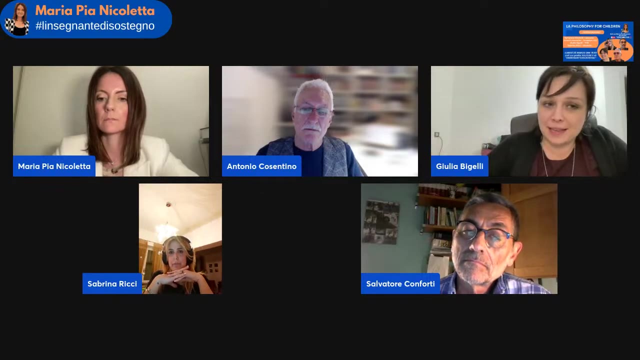 Why? Because evaluating Philosophy for Children is difficult. Why is it difficult? And why is this, in my opinion, also a Why is it difficult to enter schools? And why? Because it is difficult to evaluate a thought process, And so what I proposed was a kind of authentic evaluation. 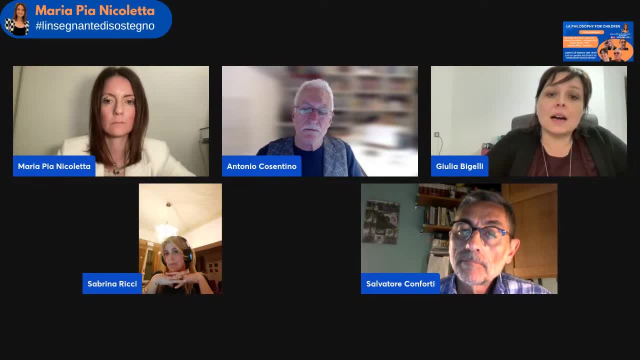 And so what I proposed was a kind of authentic evaluation, And so what I proposed was a kind of authentic evaluation. So evaluation categories, So here is a type of evaluation that focused not so much on the result as on the process, And let's say that this was a challenging element. 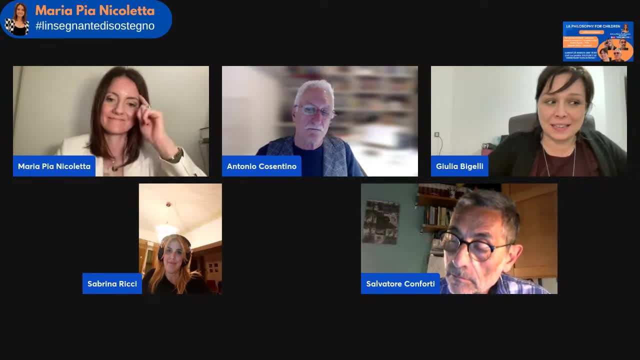 It seems little, but it has been almost nine years now. Things have changed in the educational field. We know that research has gone much, much further. We know that research has gone much, much further. But here it is. my doctorate research stopped there. 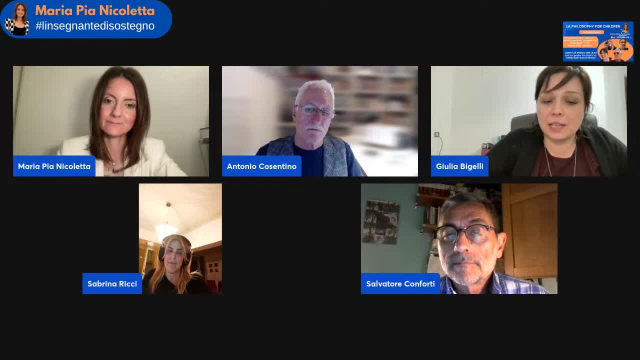 But here it is. my doctorate. research stopped there. What is my job today? I continue research. In particular, now I am focusing on how Philosophy for Children works on self-efficacy. My thought is valid. Philosophy for Children is my thought, that is, it has value. 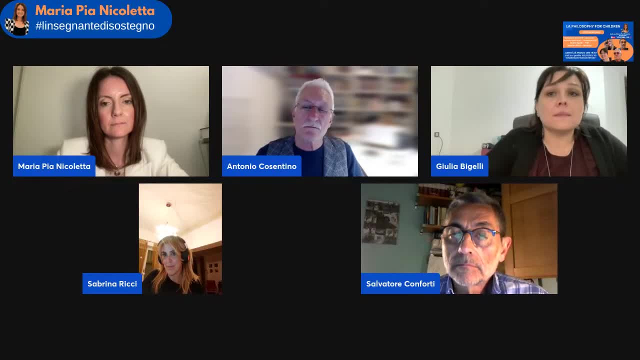 Philosophy for Children is my thought, that is, it has value. My thought is a strong thought. My thought is a strong thought. I know how to build thoughts, I know how to make reflections, And so this can help me feel more confident. 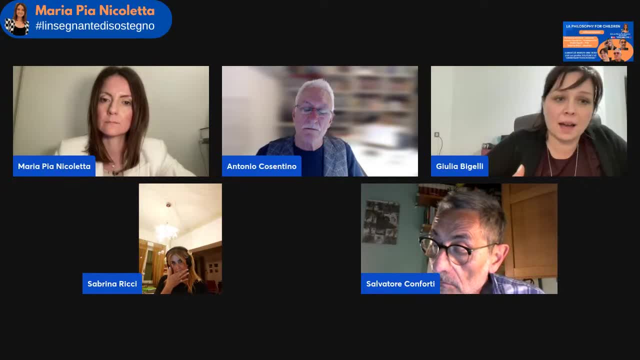 può aiutarmi a sentirmi più autoefficace a scuola? può aumentare la mia motivazione? queste, diciamo no, sono le domande su cui mi sto soffermando, soffermando ora tra la mia attività di insegnante. 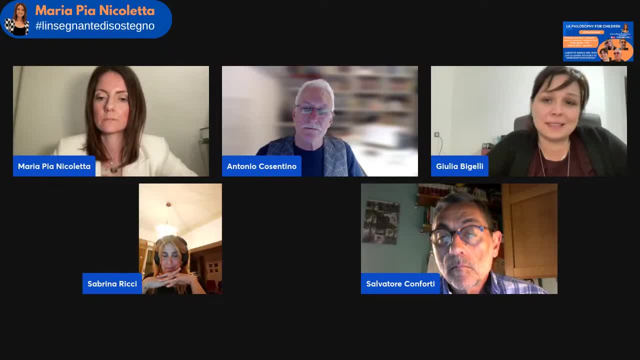 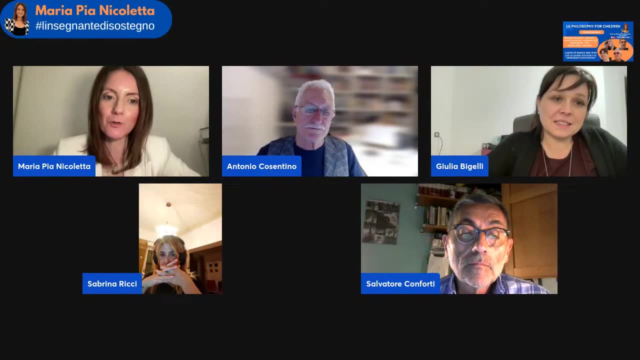 perché, appunto, sono un insegnante di scuola primaria, la mia attività invece di ricerca. perfetto, sei stata molto chiara. magari dopo facciamo un ulteriore domanda per approfondire il tuo lavoro di ricerca e la tua attività attuale, perché so che sei anche docente. ci hai tenuto. 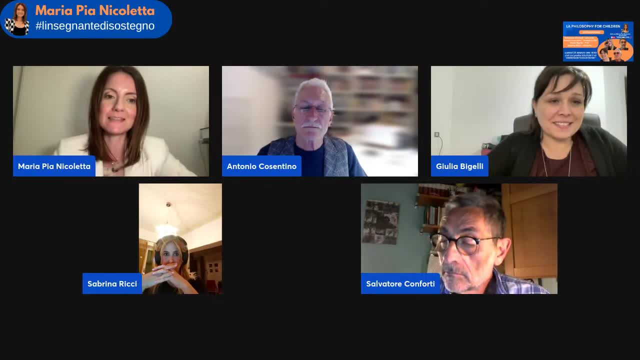 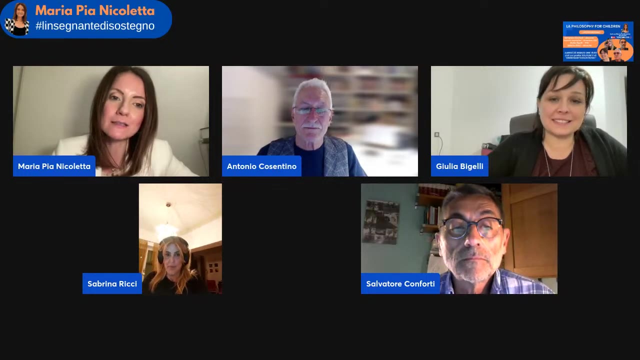 molto a esserci. io ti ringrazio per la tua disponibilità doppia, perché sei anche mamma. hai tantissimo da fare. grazie, passerei la parola al maestro salvatore conforti, maestro di p4c. la possiamo chiamare anche così, salvatore? 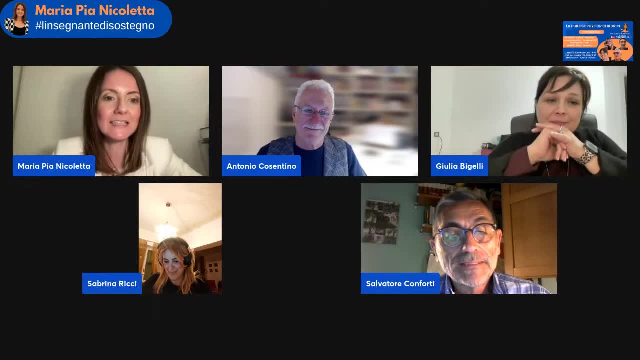 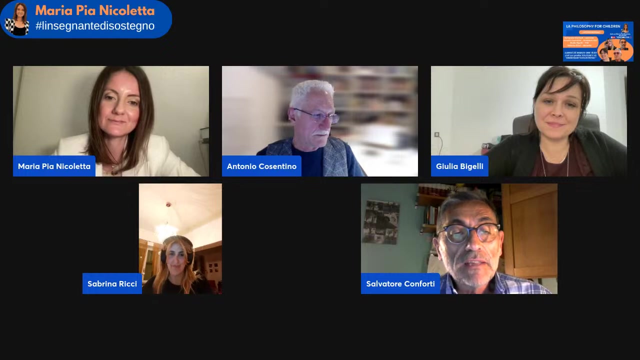 certo, perché è anche divertente vedere quelle che sono le varie. esatto, raccontaci un po', tu ora sei docente di una scuola di roma. fai solo questo, cioè applichi la philosophy for children all'interno del tuo istituto. bene, maria p, è una cosa che possono far tutti. se l'ho fatta io diciamo: 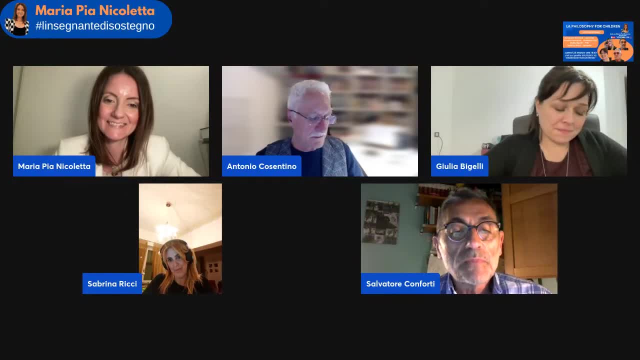 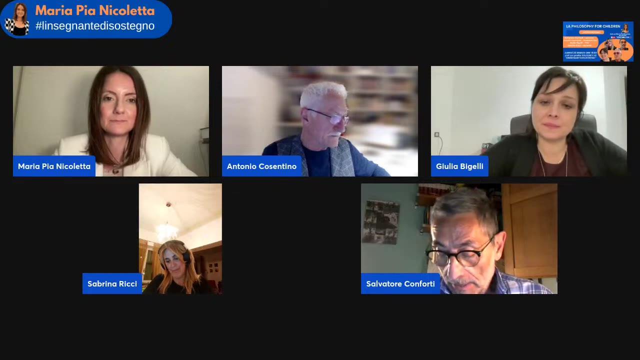 partendo da zero- credo che tutti quanti possano in qualche modo sperimentarlo- ma soprattutto trovare quella soddisfazione e soprattutto quel gusto di dare una risposta a quello che in pratica è stato un po un processo strano della serie mano mano che la nostra scuola. 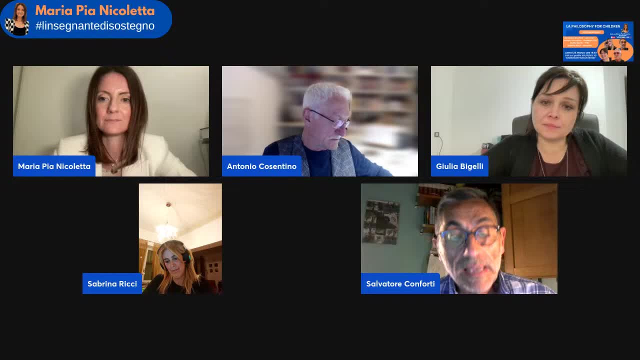 credo che tutti quanti sappiano, i nostri ascoltatori, ma anche qui presenti, che la nostra scuola elementare è stata una delle scuole, diciamo, all'avanguardia. era arrivata, se non sbaglio, al terzo o quarto corso mondiale. venivano a studiarla da fuori, dall'esterno, per. 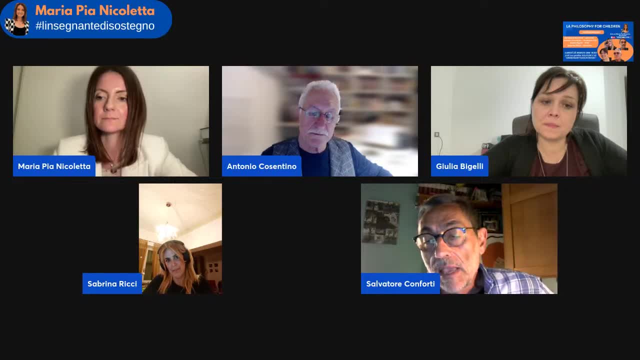 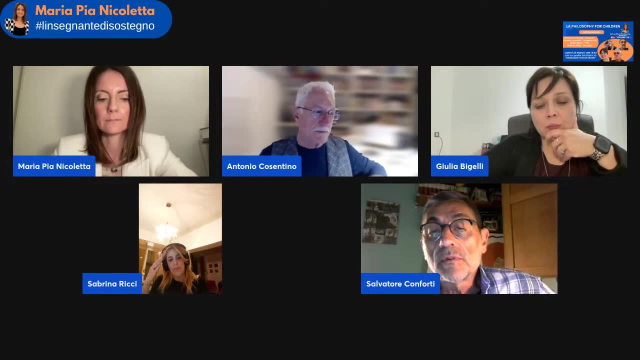 l'impianto pedagogico che funzionava, perché in effetti ci si era un po abbastanza investito su questo. poi, un certo punto qualcuno ha pensato all'improvviso di tagliare ben 9 miliardi alla. 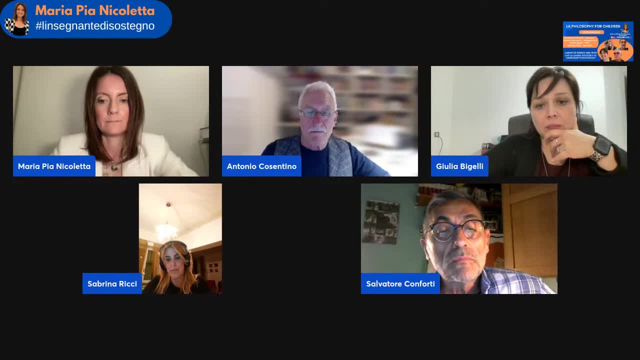 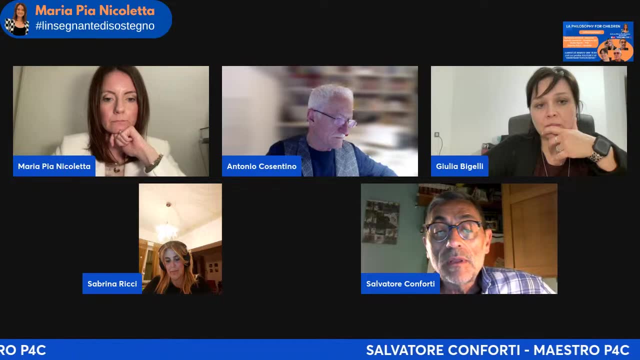 scuola pubblica. da quel momento in poi, quell'impianto non ha trovato più nessun sostegno, appunto, a proposito di insegnante di sostegno, quello del sostegno fondamentale e quindi, come tale, cominciare un po a perdere un po quello che era l'inclinazione. no, 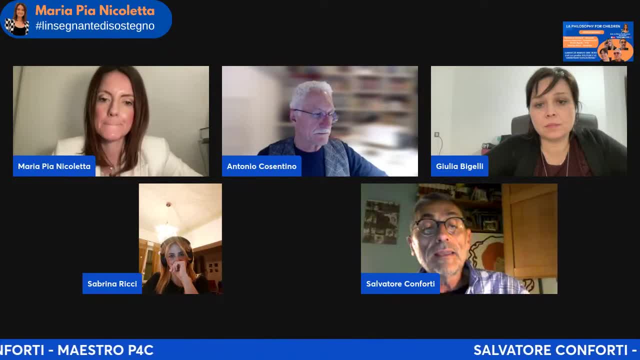 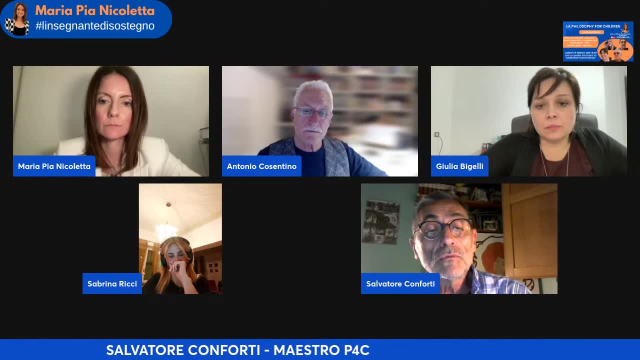 a farti, cioè a provare gusto in quello che fai. no, anche dal punto di vista personale, quando vedi che i ragazzini in qualche modo rispondono a quello che tuo insegnamento, alle esigenze loro, eccetera. 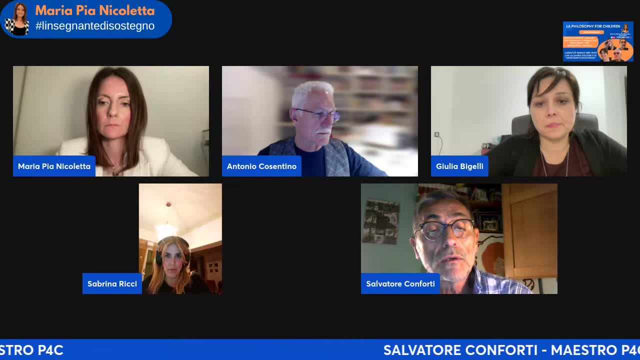 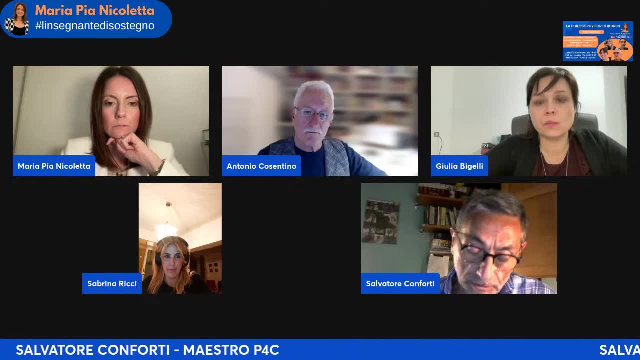 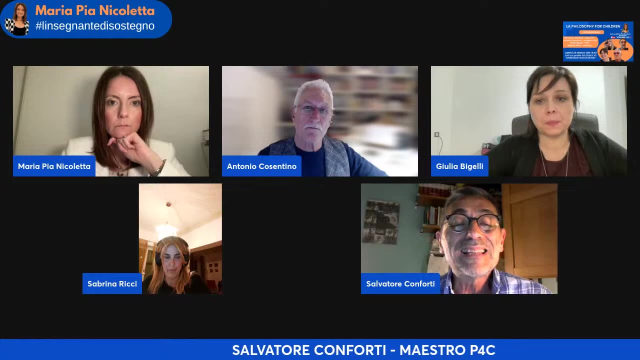 tutti gli effetti, vai avanti così con quella motivazione: forte, necessario, eccetera. quando appunto ha cominciato a venir meno questo aspetto, diciamo che l'insegnamento ha cominciato un po a perdere un po di più delle soddisfazioni. no, fino a quando trovo sulla mia strada, appunto, 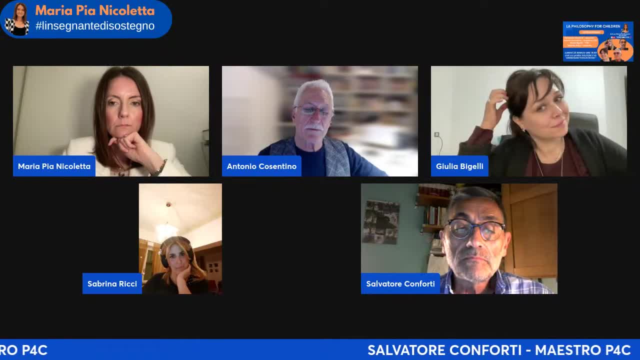 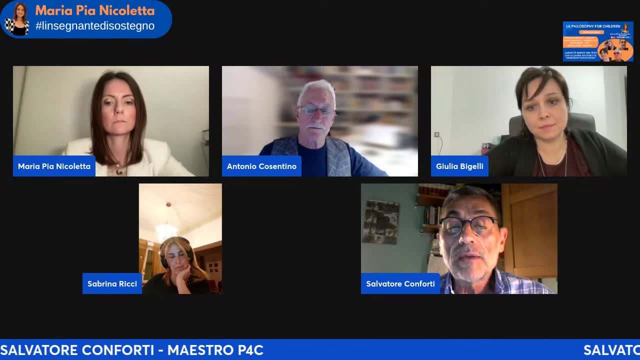 qualcuno che mi dice: ma facciamo un po di filosofia con i ragazzini, ma non dal punto di vista della filosofia cittadina, cioè gioco. amo io una collega delle scuole medie luciano, l'anna, professore a. 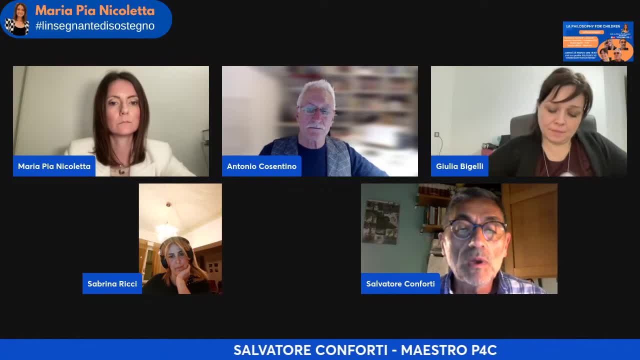 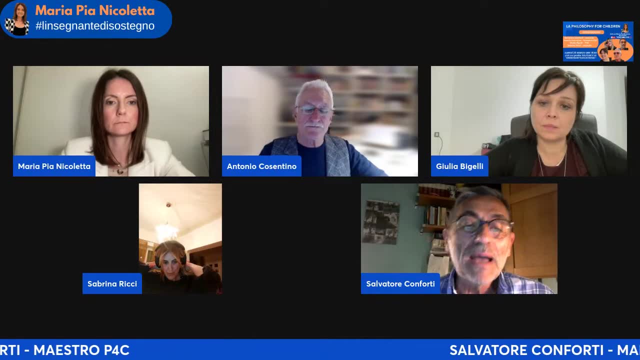 fare un po così ogni tanto a parlare di filosofia ragazzini. poi, con l'intervento di qualche signore esterno, qualche filosofo esterno che veniva un attimo a condividere con loro, diciamo questa, questa. 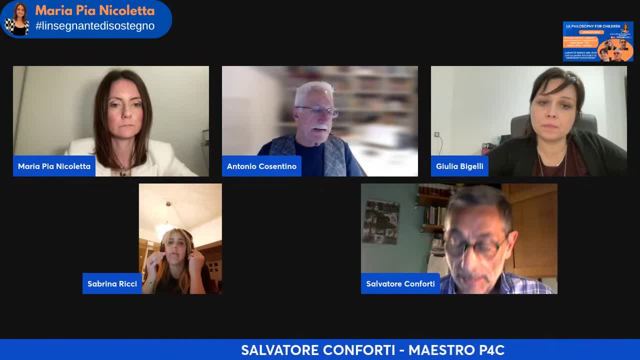 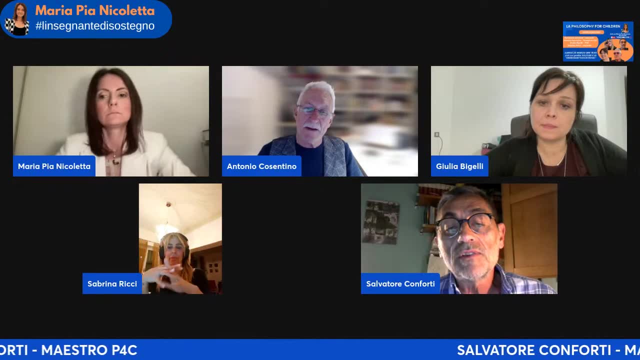 sì, di dialogo, di confronto, di divertimento, insomma, volevamo darci un po un tono. no, ma fu appunto nel cominciare. diciamo: questo gioco in effetti siamo accorti, anzi è incontrato sulla. 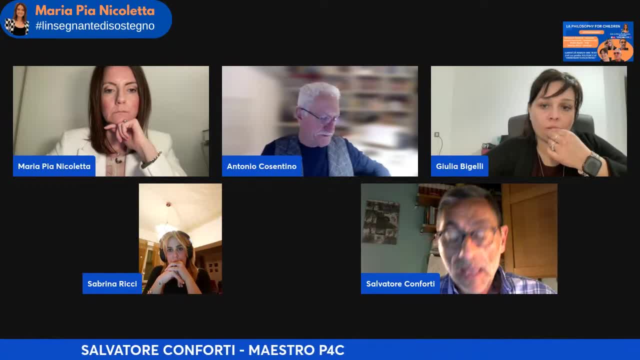 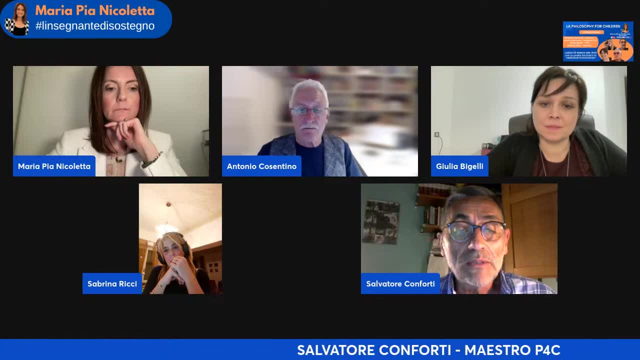 strada, grazie a qualcuno che ha avuto modo di presentarmelo, antonio, che appunto mi disse: ma guarda, per fare tutto questo esiste un metodo preciso, che non sia un metodo che funziona in un certo modo di come anche modo. ma guarda, tu come lo fai, io lo faccio. 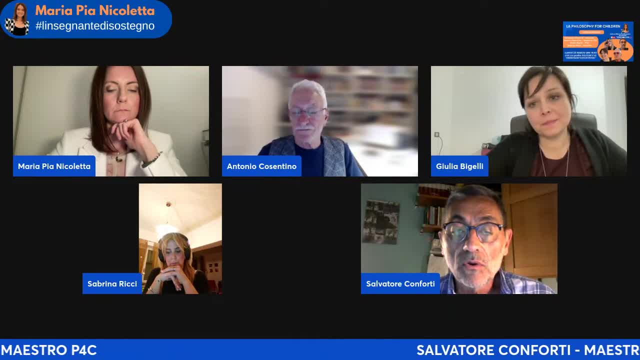 così noi lo facciamo con la. alla fine, insomma, troviamo un punto d'accordo che più o meno era quello che avevo pensato di adottare pure noi, solo che, appunto, non ha se non seguivamo quello che era. 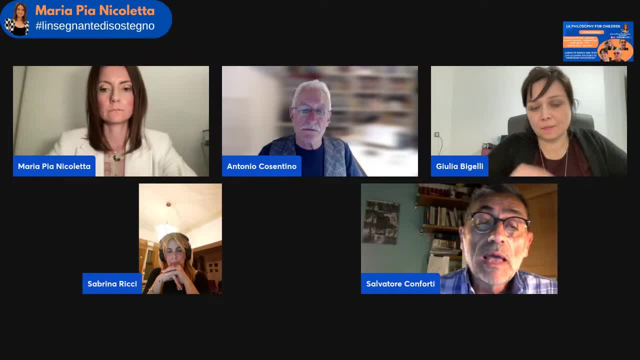 la metodologia di rickman. non eravamo assolutamente a conoscenza. insomma, senza farla lunga, dopo una settimana che ci, dopo che c'eravamo appena conosciuto telefonicamente adonio cosentino. 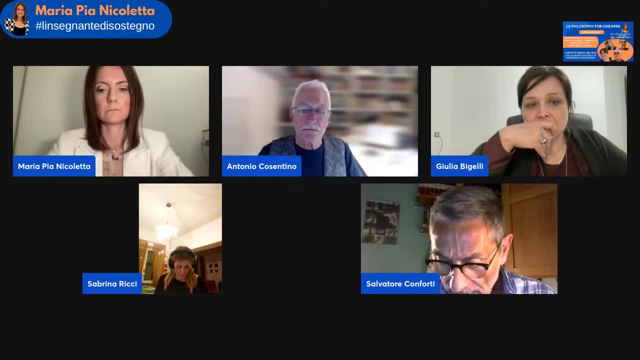 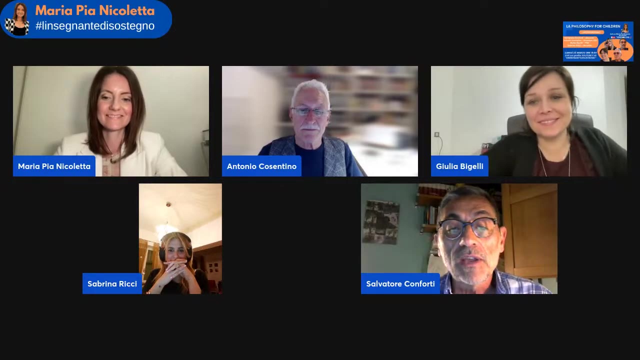 si presenta nella mia scuola, nella mia classe e in un anno, inaspettatamente, della serie di sai che figurate, se vengono in classe tua, sasano, hanno sempre un po rossi e nemico sia importanti, stanno sul loro piedistallo un filosofo, un filosofo. insomma, è invece antonio che appunto filosofo lo. 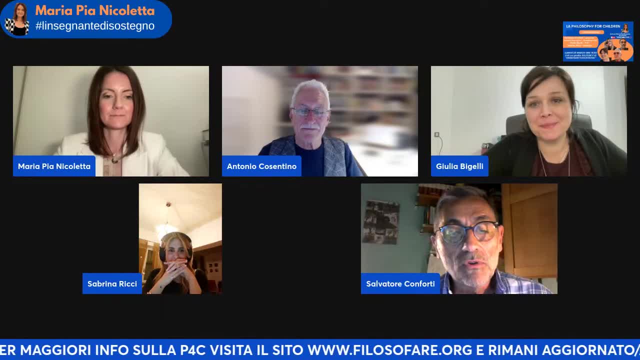 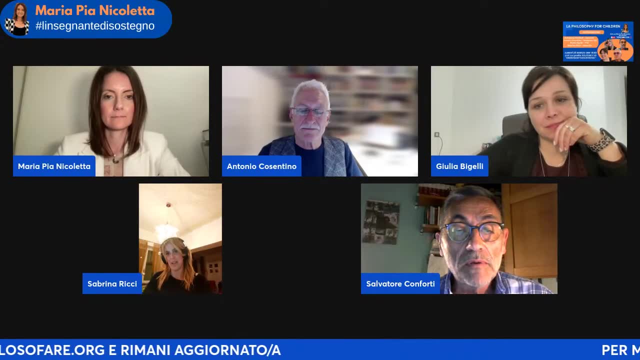 è, ma lo è praticamente. si è voluto confrontare subito su quello che era questa esperienza che stavamo portando avanti. e lì mi si è accesa, non ad amano una lampadina, magari un intero forno insomma, il quale ci siamo buttati a capofitto e devo essere singelo nel giro. 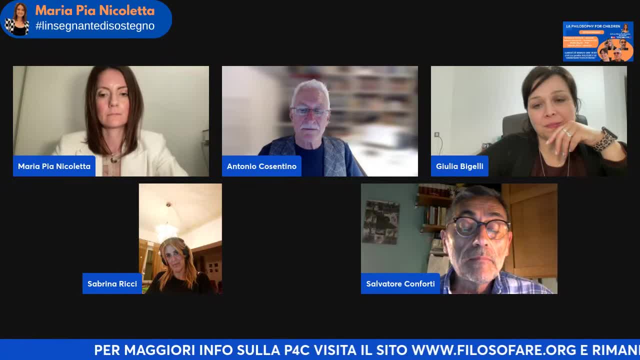 di non più di due o tre mesi, il mio atteggiamento rispetto all'insegnamento è totalmente cambiato, anzi, permettetemi di dire, e c'è stata una vera e propria rivoluzione. ma la rivoluzione non è. 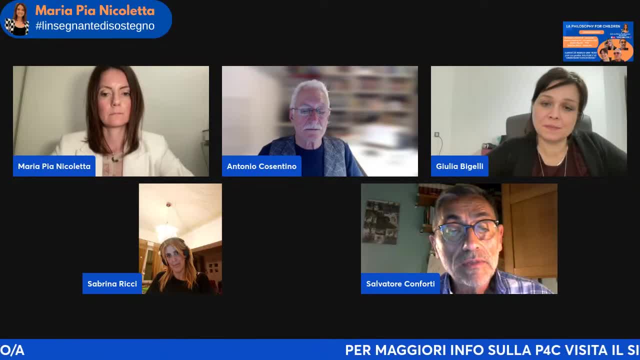 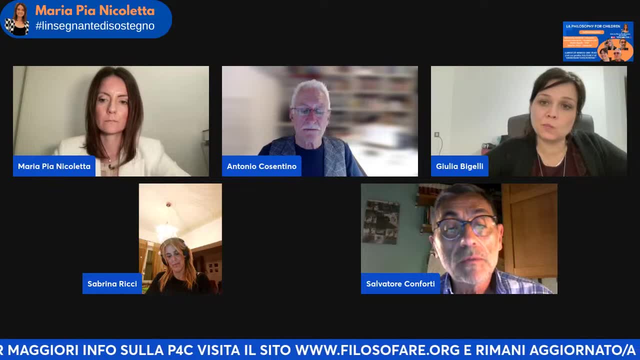 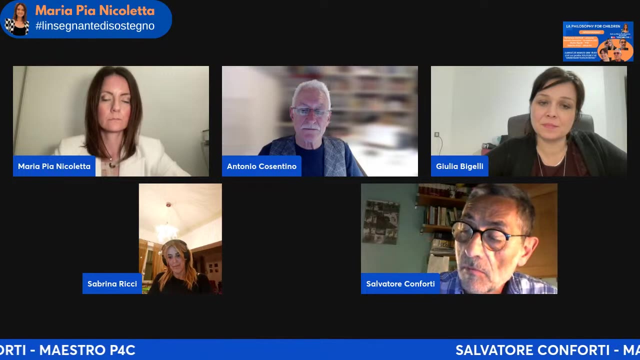 stata in me. la rivoluzione è stata nelle classi che io avevo, diciamo quelle quali facevo questa prima esperienza, tra l'altro in maniera pure del tutto nascosta rispetto alla dirigente scolastica perché, sa, a volte queste novità possono non piacere. ma siccome alla fine dell'anno qualcuno 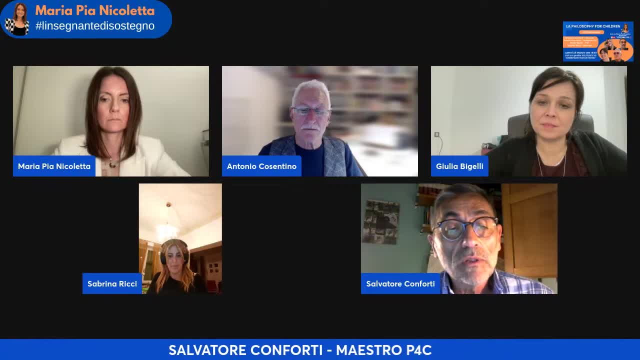 cominciò a sentire: no, fuori sa, se vuoi, dei corridoi, se ne parla, se ne discute, eccetera. qualcuno comincia a sentire degli effetti benefici, soprattutto i ragazzini, devo dire, e soprattutto 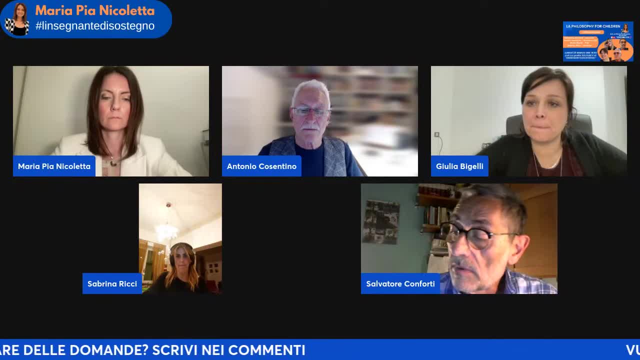 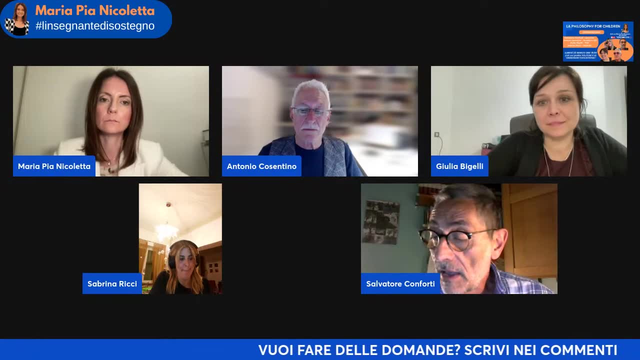 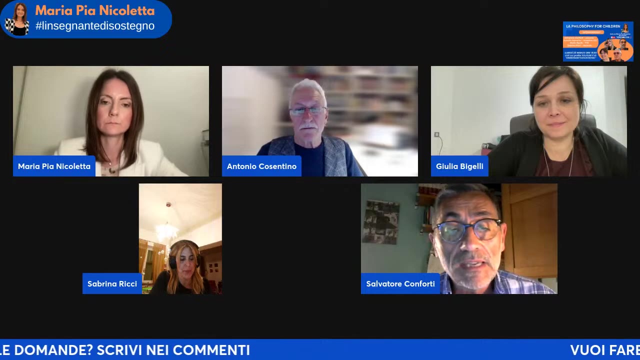 arrivò questa nome a questi interessi e pure ai genitori, i quali, in effetti, erano estremamente contenti di questa attività che si svolgeva. insomma, io cominciare con due classi e dopo di che, quando la preside capì che si trattava di qualcosa di significativo, me ne 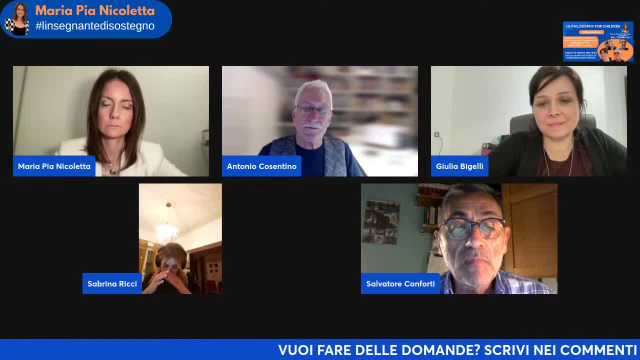 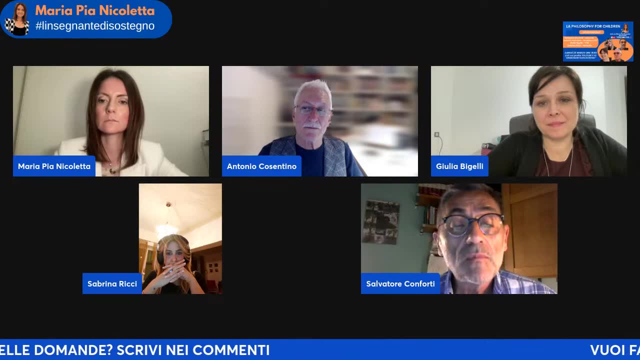 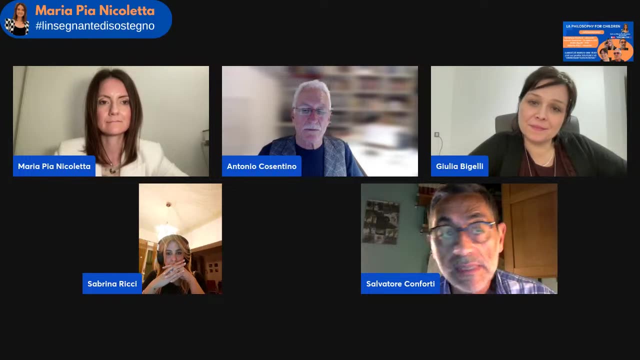 diede, me ne affidò cinque e insomma, nel corso degli anni. sono passate adesso sette, otto anni da quando io ottava attivato questo, questa educazione, diciamo così. all'interno della mia scuola siamo arrivati a dieci classi e oggi siamo all'undicesima. diciamo che più di queste 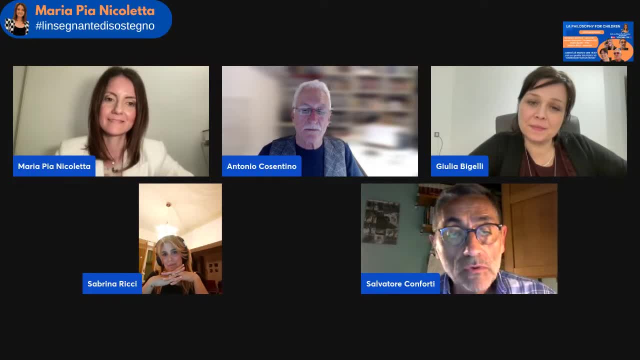 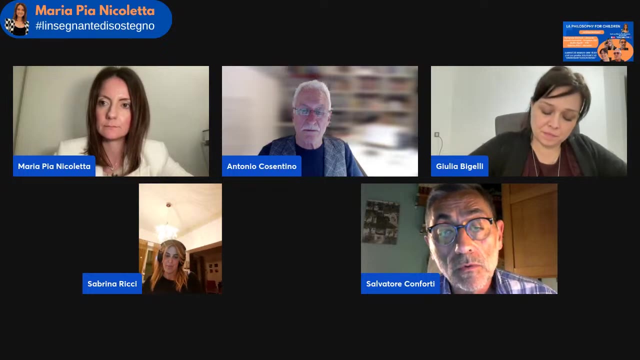 per me è impossibile, ha rivoluzionato la mia. ricordare forse ricordare, salvatore, a chi ci sta seguendo il nome della tua scuola. la mia scuola si chiama istituto borgoncini duca e sono tre plessi, tre plessi scolastici, uno se ne si chiama via manetti. 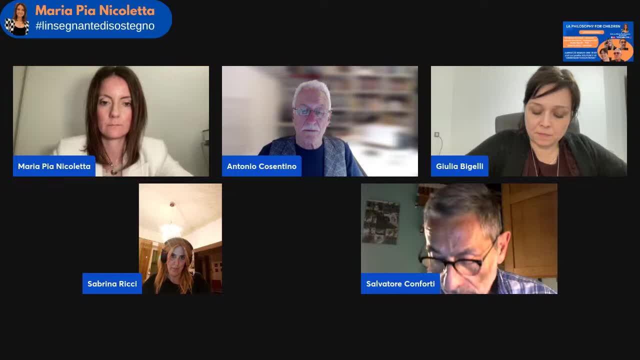 l'altra l'ottobre, l'altra appunto san francesco. insomma, in questa scuola, insomma, la preside a un certo punto ha capito, ci ha visto lungo, diciamo. hanno avuto anche un forte coraggio di quello di 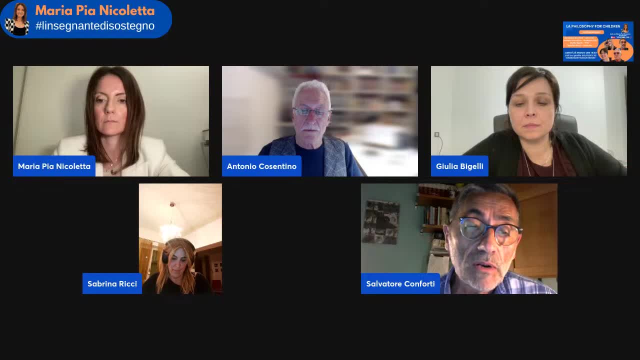 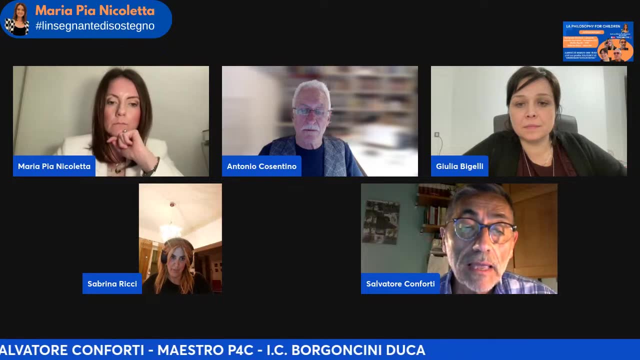 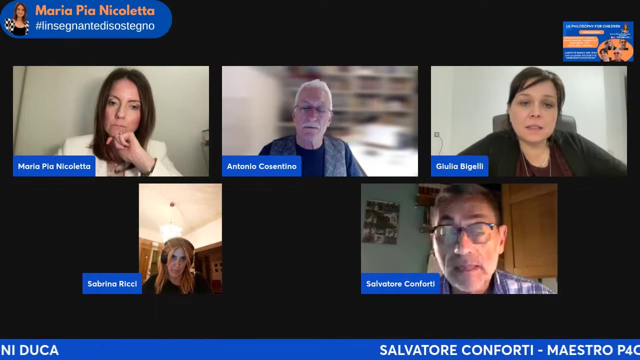 avermi assonerato dall'insegnamento di tutte le discipline, perché voglio dire una cosa: non è una questione così, né immediata e né facile da prendere, il che significa che qualche valore aveva da tipo di riconoscimento, tanto è vero che nel frattempo non fu neanche questo un caso. 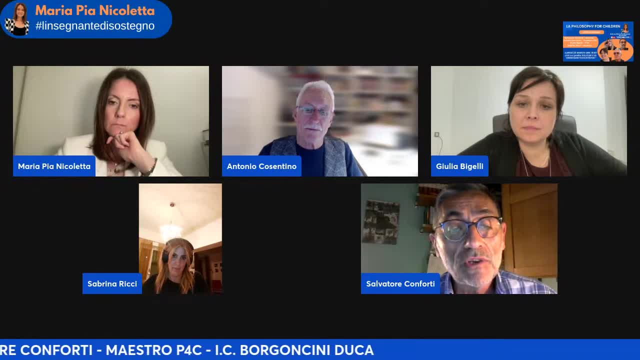 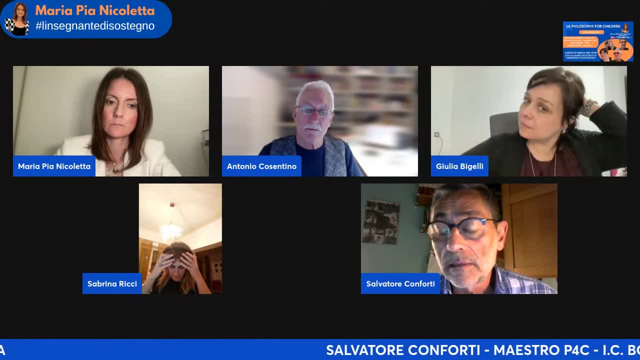 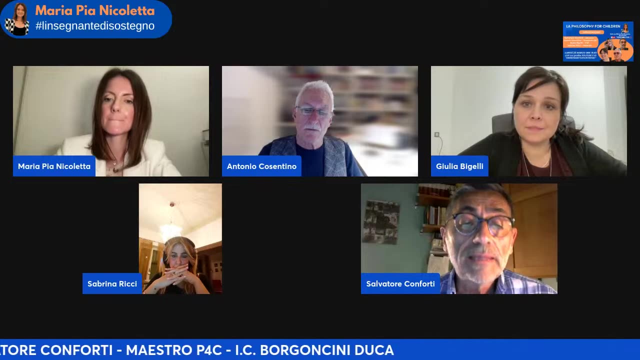 l'assessore della scuola di roma, in pratica ci offrì una vetrina importante nella, nella sala del campidoglio, per ben tre anni di seguito. ci invitò a testimoniare in pratica l'attività della. 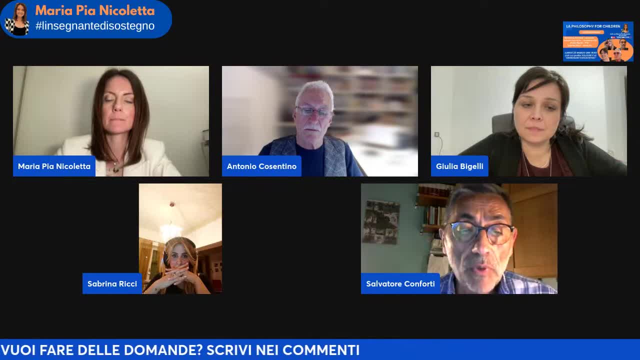 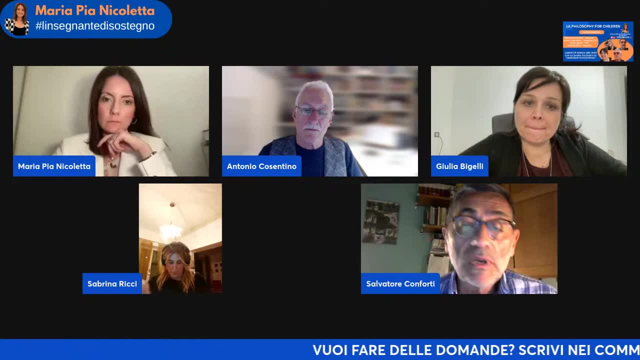 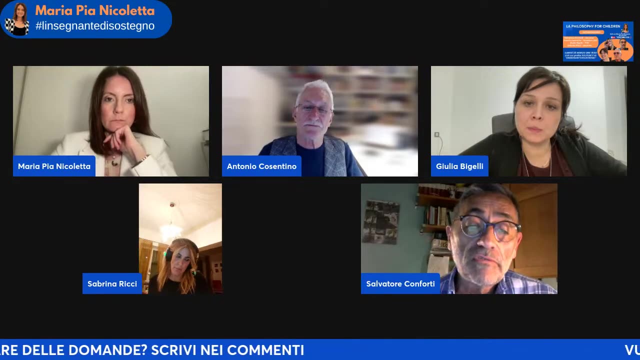 filosofia for children, quali tipo di risultati e porta. è chiaro che, per quanto riguarda noi, soltanto gli eventi- no, o appunto queste erano degli eventi- possono effettivamente testimoniare che cosa succede. perché valutare, come diceva prima giulia, il prodotto è facile: il 2 più 2 fa 4, 6 fa 5. 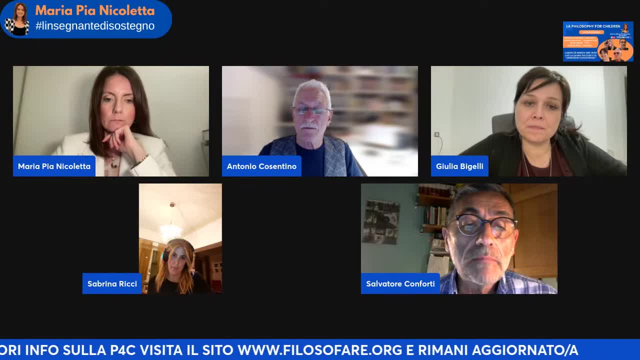 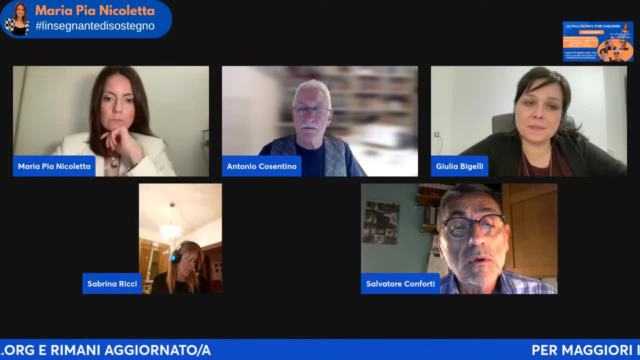 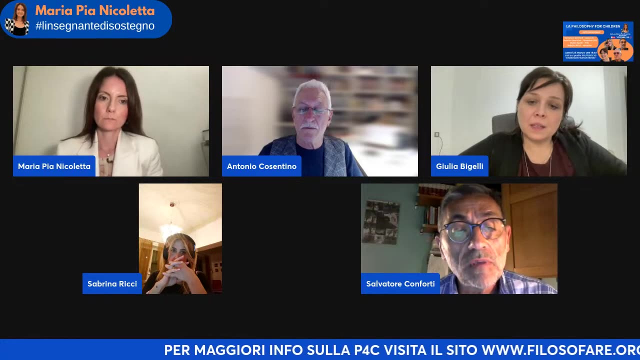 è difficile perché il processo si valuta soltanto a partire da un qualche cosa che fluisce. si parla prima di un flusso per poter arrivare poi dopo a un qualche cosa, anche non che tutto determinato, ma che comunque un flusso che si si rende conto che ha un suo principio, una sua partenza, un punto. 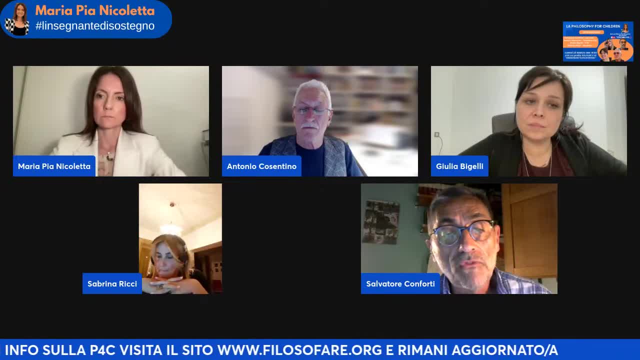 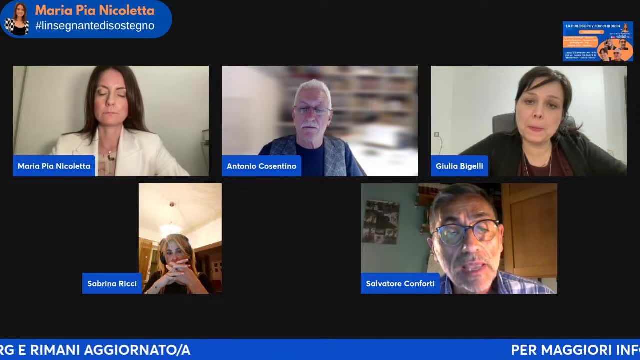 di arrivo e quello interessante perché offre la possibilità a chi viene dopo, quindi alle scuole medie e superiori, volendosi, di incamminarsi in quel flusso e capire finché la scuola di roma è. 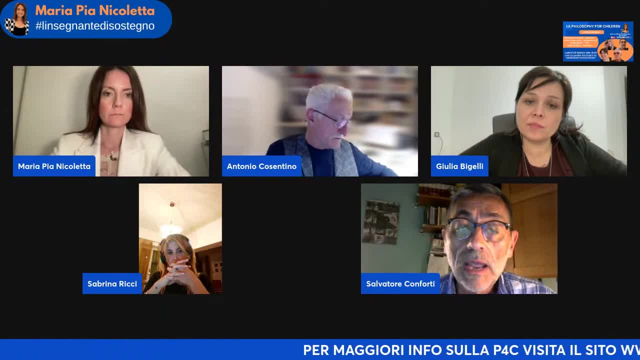 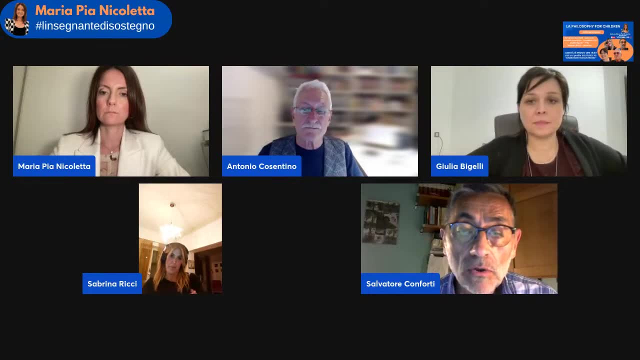 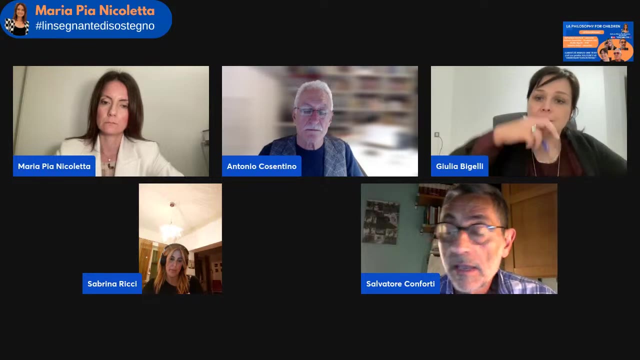 effettivamente, qual è una valutazione di questo genere? una valutazione di questo genere, diceva prima giulia, e quella efficace con, l'effettiva, quella che ha valore. le nostre valutazioni di oggi, permettetelo di dire, anche se so che posso farmi dei nemici, in questo sono assolutamente. 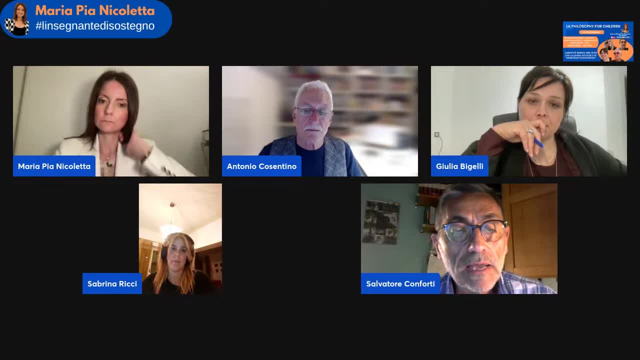 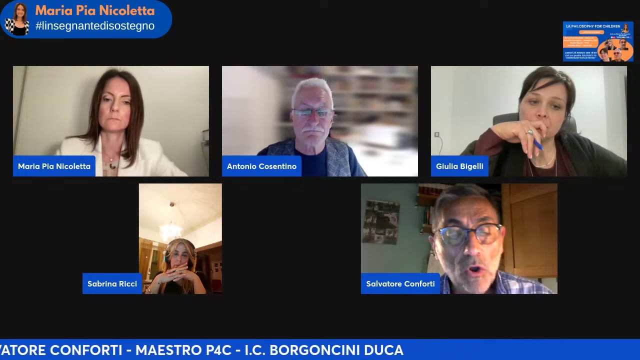 insignificanti. che cosa significa valutare un bambino, una bambina, un ragazzo con un numero, ma che siamo numeri noi, cioè importanti, poter dire effettivamente che cosa sono in grado di saper proporre loro, a noi, e quindi valutarli. 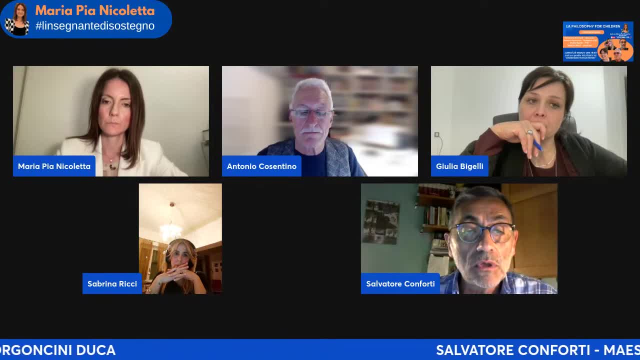 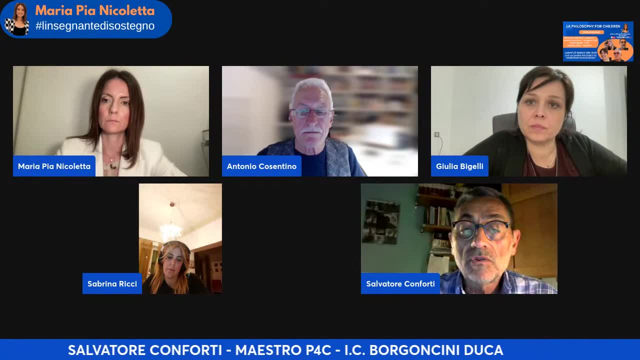 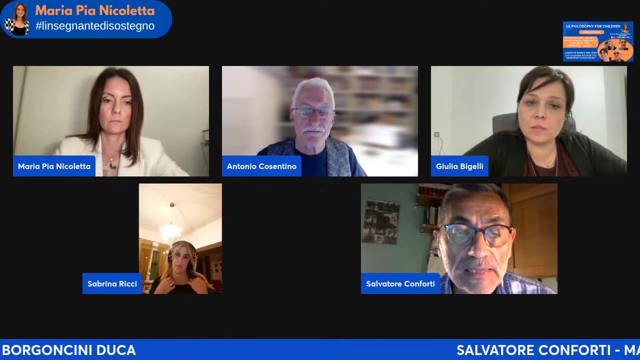 in base, diciamo qua, lo spostamento che è avvenuto da parte loro, partendo da un qualche cosa di che avevano già addosso, portandolo, diciamo, a un risultato differente, diverso, che noi in qualche modo possiamo soltanto che testimoniare. cioè, io avrei degli esempi qua molto pratici da dire. 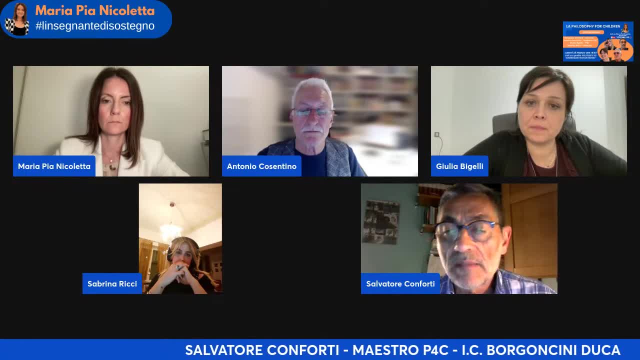 insomma, però non voglio limitarmi a quelli che sono stati presenti, e che sono stati presenti, perché sembra quasi che siano queste poi delle fotografie di quello che succede in classe. magari poi dopo, se c'era un secondo passaggio, dirò qualche cosa che succede in. 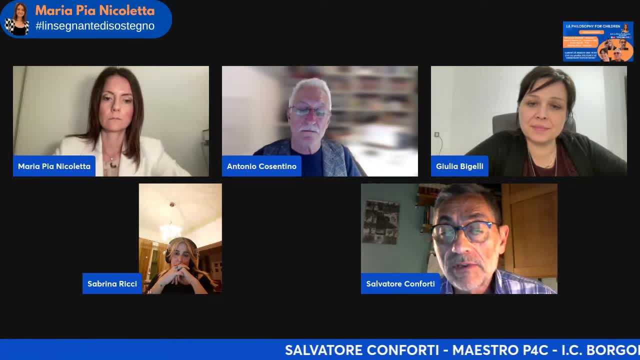 classe in maniera più specifica, anche per far capire a chi ci ascolta di che cosa stiamo discutendo e parlando. ma soprattutto direi che la cosa più importante è venire assistere e di conseguenza cercare appunto all'interno no di quella, di quella, quella sessione, quell'attività. 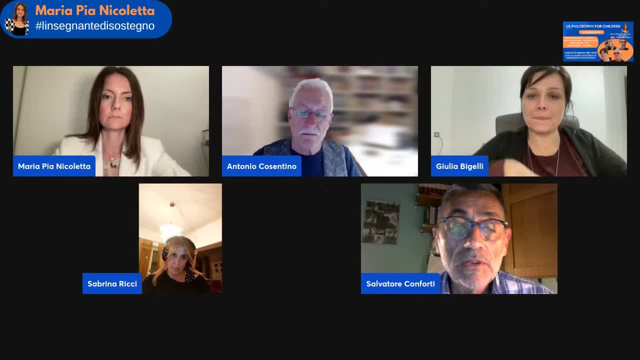 ossessione filosofica: percepire, recepire quali sono effettivamente i risultati e che si toccano con mano. insomma, io, in questo contesto è inutile dirlo perché un po tutti quanti conosciamo quali sono, forse compresa la, la collega sabrina. insomma, mi fermerei qui. grazie mille, salvatore. tra l'altro, 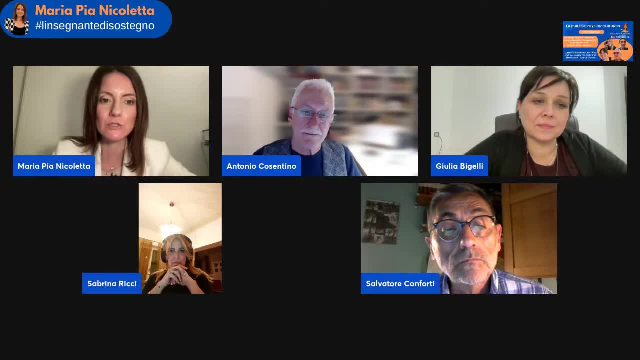 con antonio e salvatore condividiamo le stesse origini del sud. siamo calabresi. io sono veramente orgogliosa di questo ed è un vero onore per me oggi parlare di filosofi for children con esperti come tutti voi adesso. 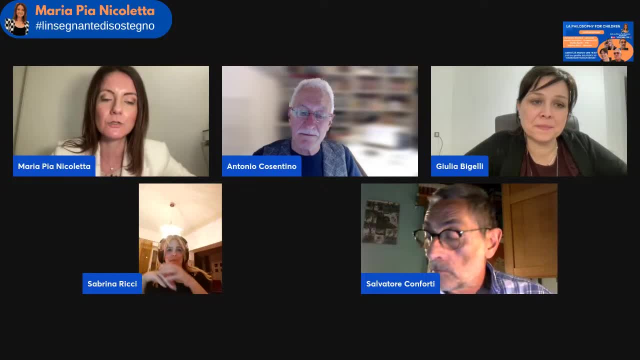 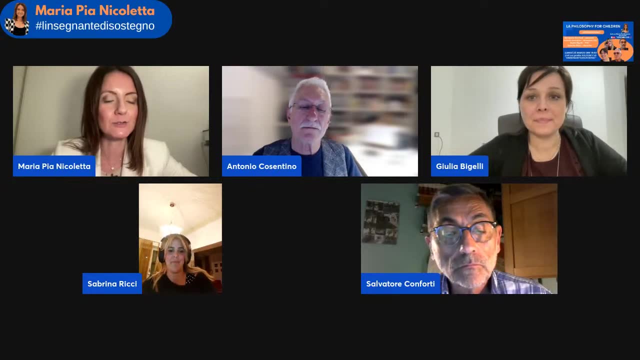 lascerei la parola alla collega sabrina ricci, docente di scuola primaria, testimone oculare di quella che è stata l'attività del maestro salvatore conforti, maestro di filosofi for children. ecco, sabrina, intanto, grazie per essere con noi, grazie a te, anche con te. 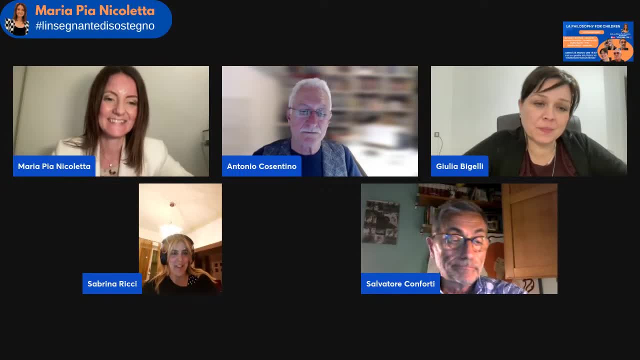 i miei amici che vi sono scattati e che a un certo punto dovete avere una città al suo proprio posto. è nato questo scambio su instagram. casualmente si ho risposto ad un post. da qui è nato tutto. io ti ringrazio, sono veramente onorata di stare qui con voi, con di rivedere salvatore. 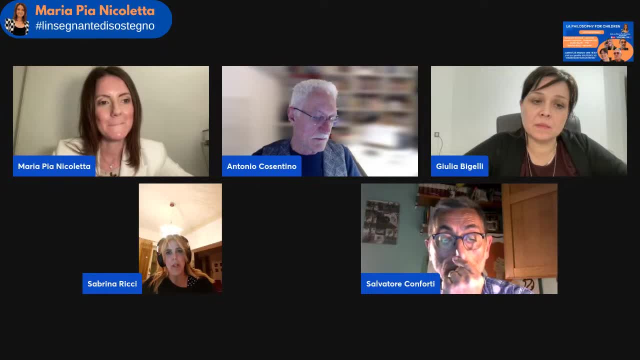 perché ho condiviso l'anno scorso a roma nella scuola borgoncini duca- io stavo nella nel plesso on support- because for me the key word in this is inclusion and I refer to everything Giulia said on metacognition, on the development of critical thinking, because I touched 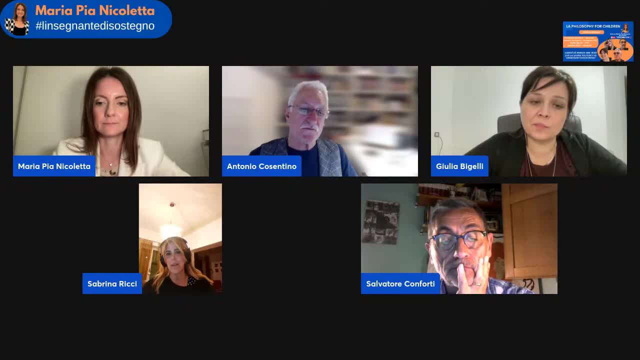 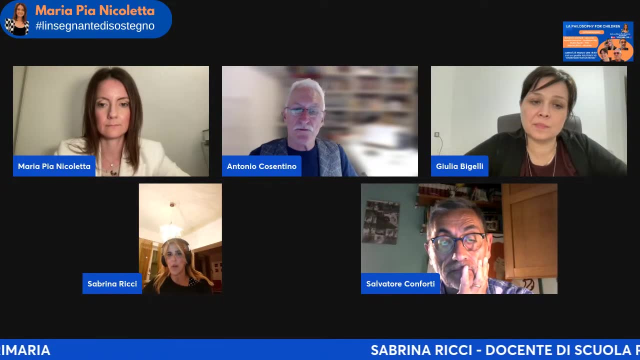 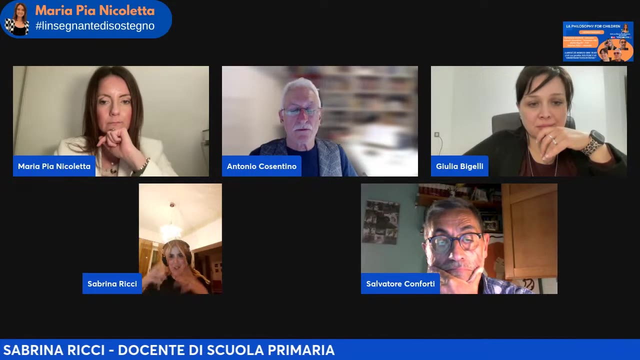 with my hand, that is. I was practically already a teacher of disciplines. I did activities with children who did not limit themselves only to the front lesson. I was looking for various channels. so many times, even with the teacher, we discussed the digital and let's say that not a little to bring out those famous 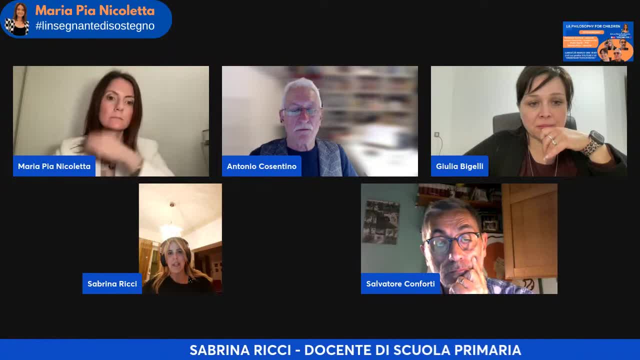 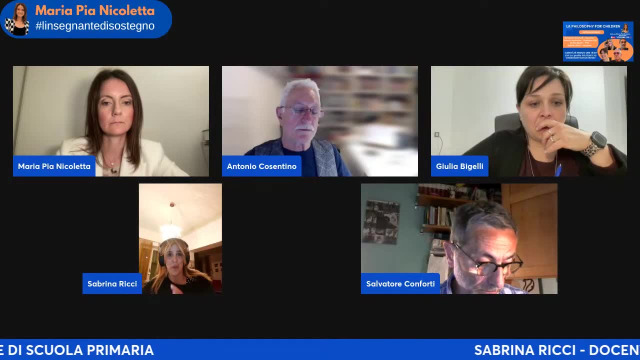 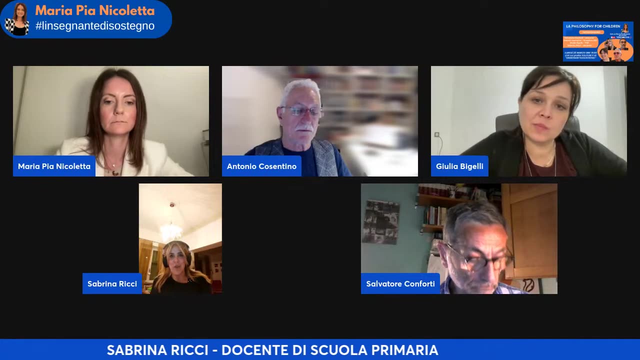 talents, those potentialities in children, and I found a huge support with the didactics, because then, as Giulia said, there is still a link with philosophy, and then didactics, because I touched with my hand and therefore for me Salvatore was a 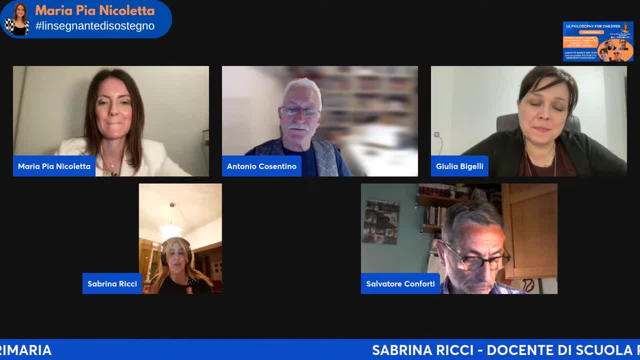 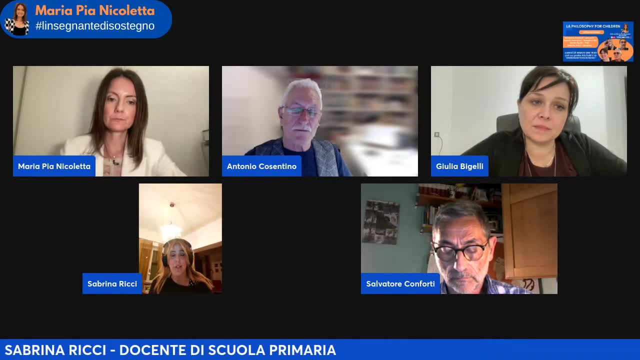 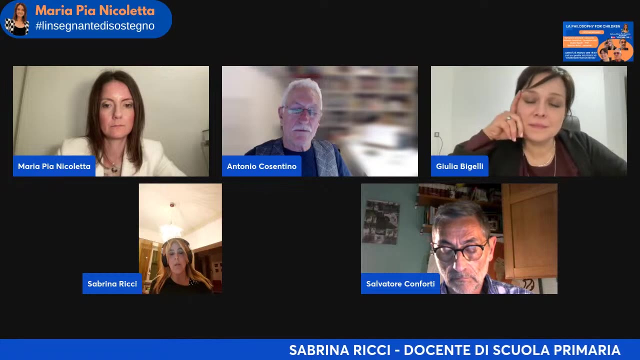 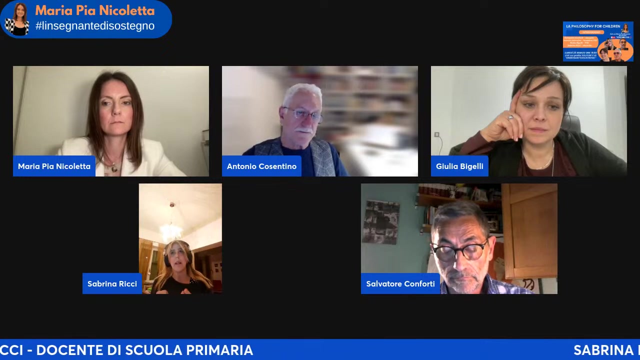 reason of solitude. I immediately got close to this methodology, to this fantastic approach. I was just a witness of this in this circle, in this circle where children are really free, free even to make mistakes, to say what they think. so both absolutely metacognition, but also the relationship, let's say also the consciousness of the self and of the self. 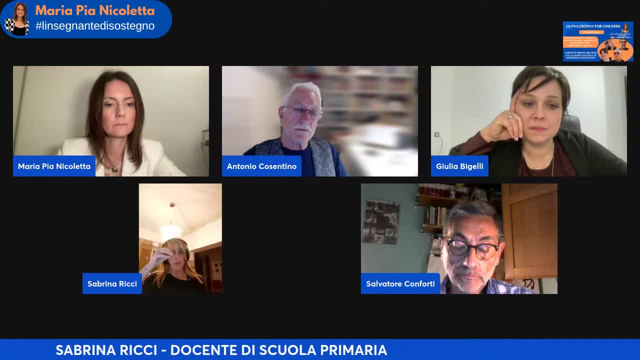 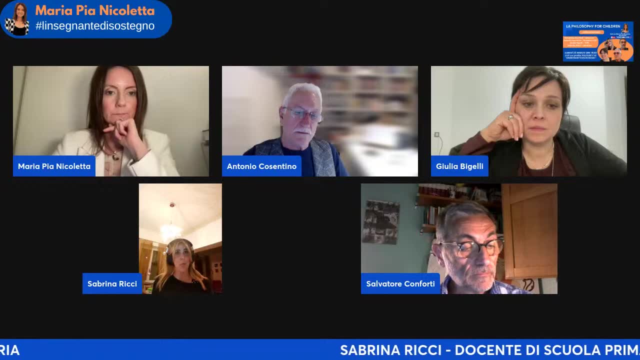 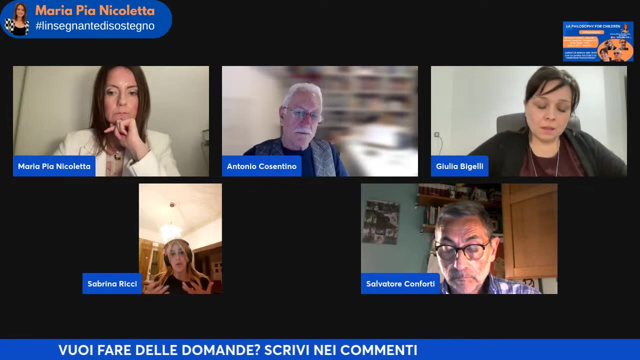 of the other and therefore perhaps the children who had some difficulties in some way in the classroom didactics. I speak for myself in class, when, yes, I tried to adapt the activities, came out with Salvatore even more because maybe he valued what was a natural predisposition. 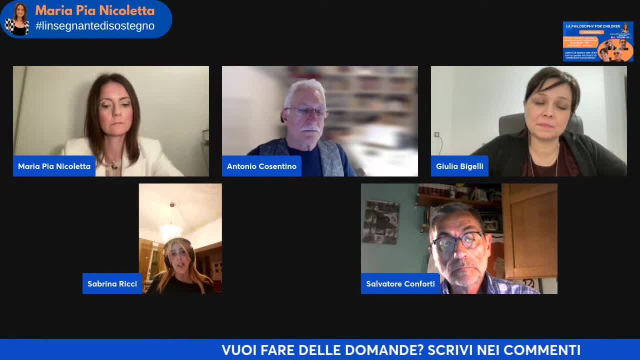 of that child who instead, in other circumstances, did not come out at all, because it is also a natural predisposition of the child who instead, in other circumstances, did not come out at all. however, it was a tool that I used to learn something new, because I could somehow create. 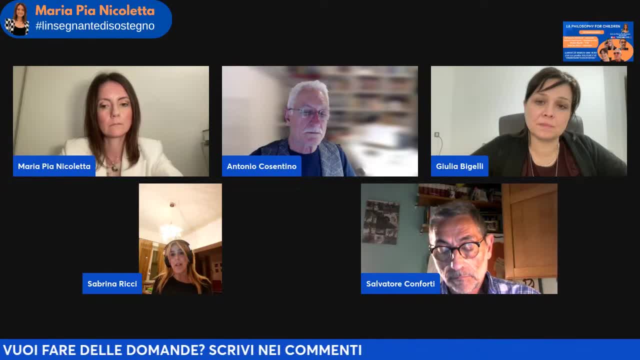 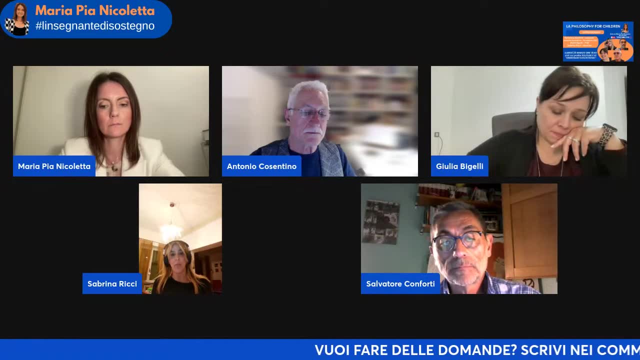 again, what would be soup with the children who were looking for a better education, a creative, from the outside. that's why I really say this is the school of talents. that is, with philosophy I have really seen what a didactics can do, because for me it is innovative didactics. 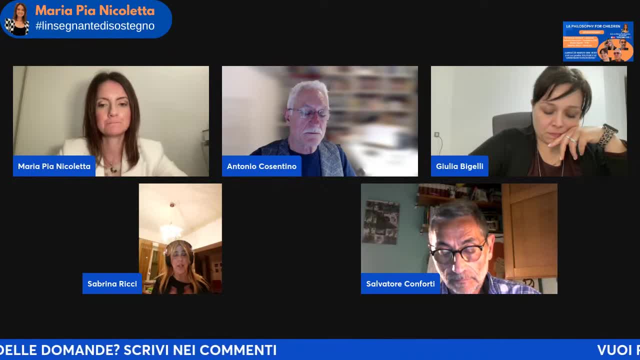 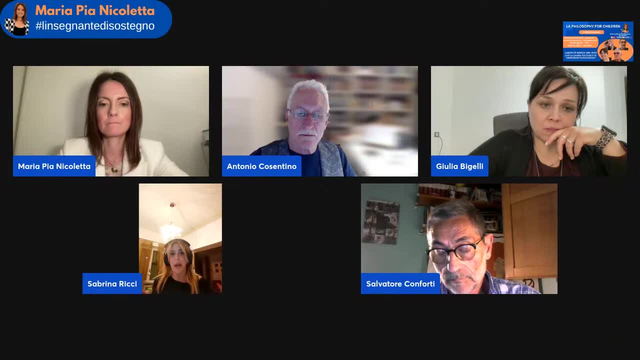 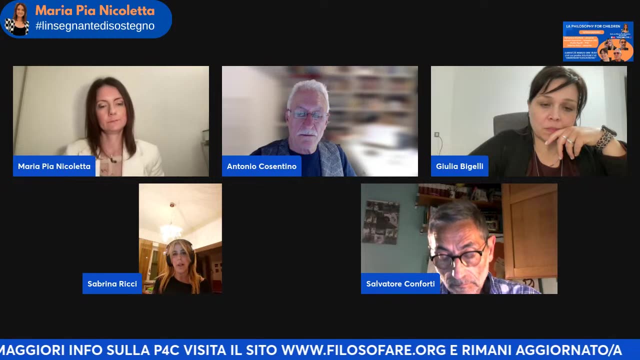 also this is inclusion at 360 degrees, because a child who has relational difficulties in the group, normally in the garden or in the classroom, because maybe he has a different predisposition there in that circle, came out of the incredible abilities, think phenomenon, critical reasoning. 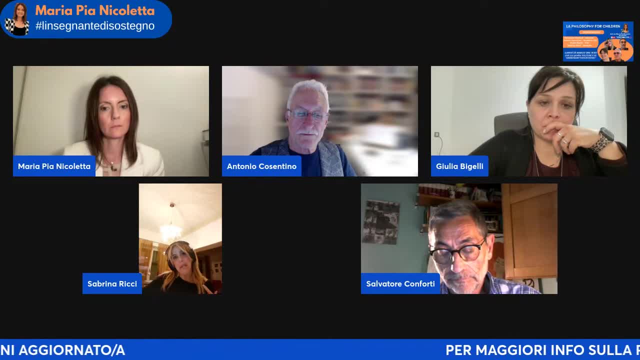 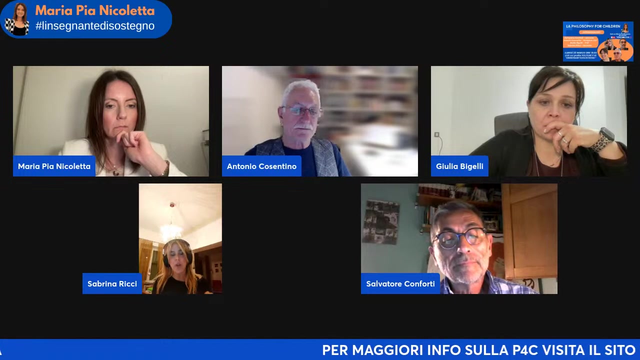 even understanding the different point of view from the other and therefore the acceptance of others, because in another context this child was not understood, even taken up around- is at that moment the child reflects and says he is saying really an important thing and therefore we have. 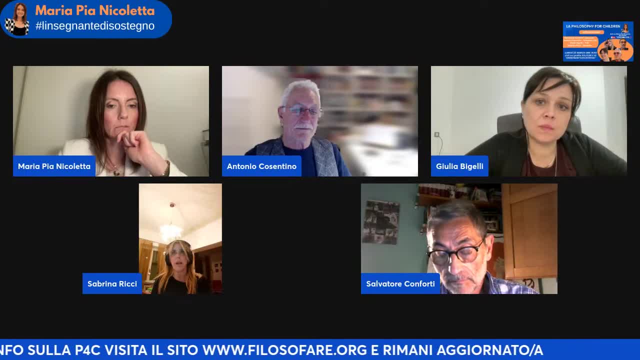 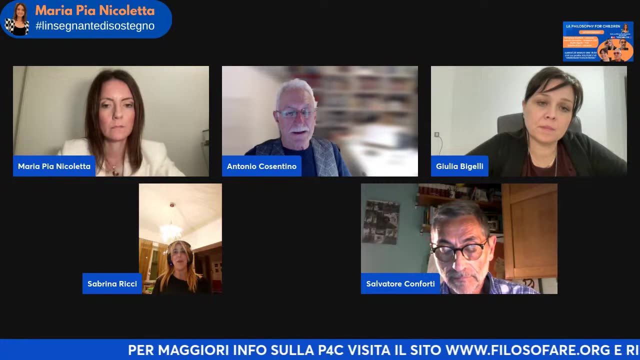 just experienced this aspect in a way, that is, I got really close in curiosity and Salvatore then wanted me one day in a live broadcast. they came to the television to record us and I was really amazed not only by the freedom but also by the way of not having 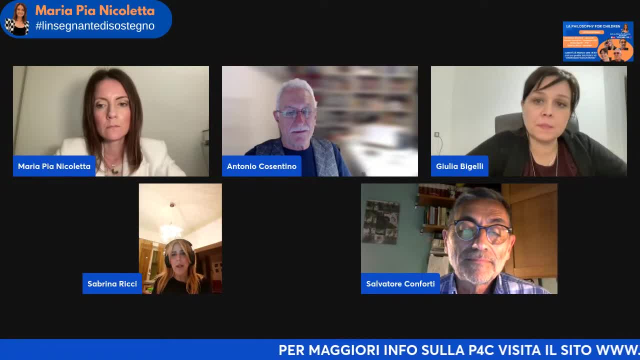 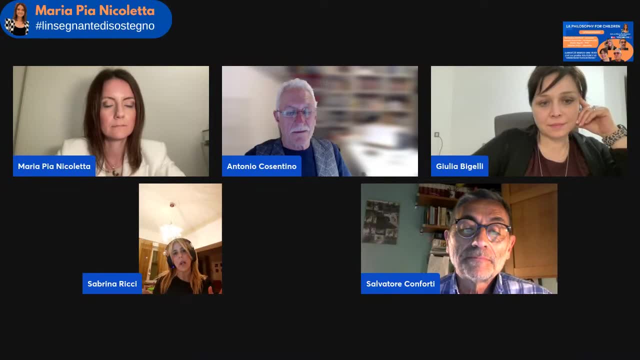 to dance does nothing, so much I am in an environment in which the other accepts me, because I can say anything. you go back to that topic that the master, because the master was absolutely a facilitator who was able to guide the children in an excellent way, and therefore this: 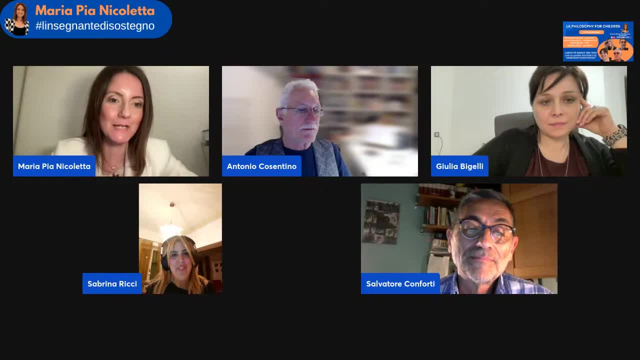 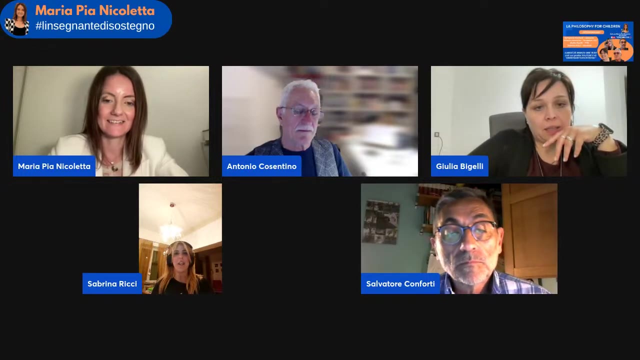 teacher Daniela Lucangeli and moral brother, is fast in good. you in fact now reading every test, the last I'm reading the time first baked of the error and therefore the roll afraid ball. but all the efforts that come back are wrong if everything is wrong. 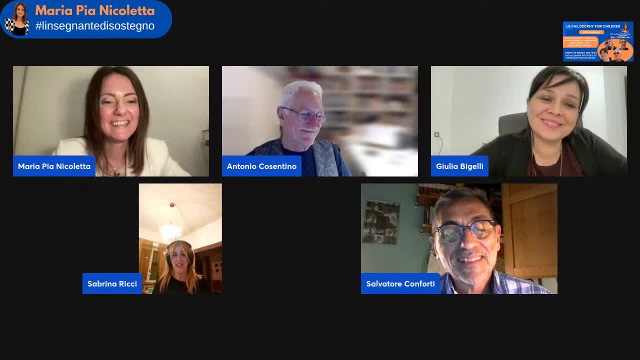 does nothing. see, I was wrong. If you make mistakes, you don't do anything. it's true, and therefore also let's say a way of putting yourself. that is empathy. here it comes back with everything that is. we can talk about Morin, we can talk about Brunner, about Goleman's empathy. really, there are a whole series of ingredients that have really made everything easier for me too. 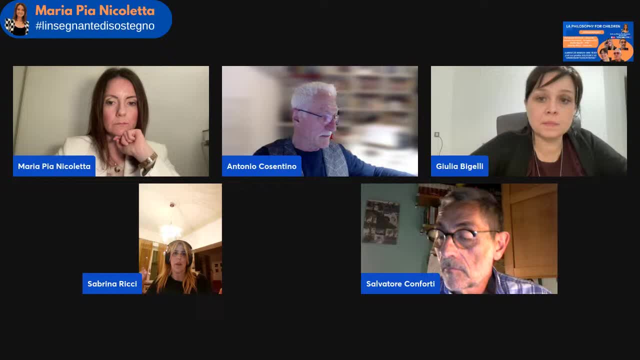 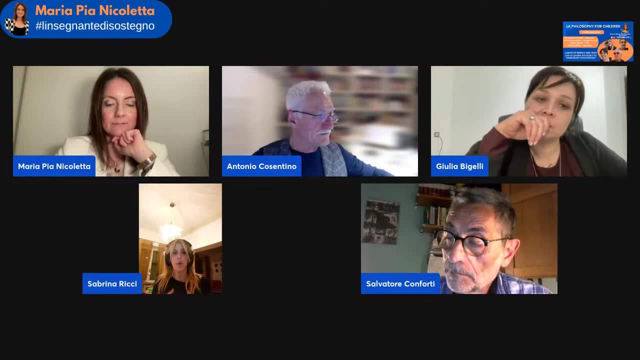 and then I would go back to class and still say, okay, these children are used to reasoning, they are used to it and this way of reasoning also led them to be autonomous anyway, because they developed other abilities. that is, it's all completely connected and it's really made a world. I am happy to have met Salvatore in this tiring year. 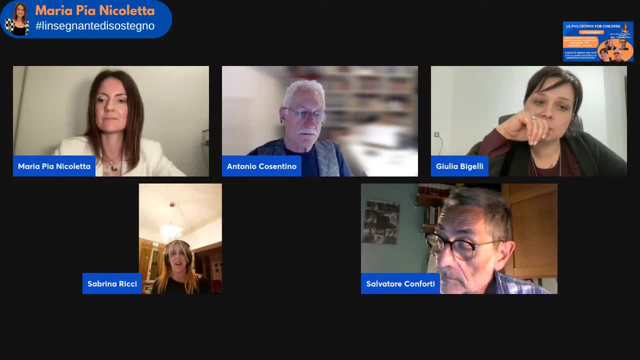 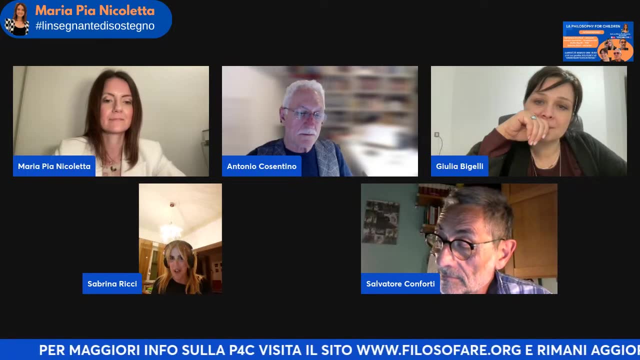 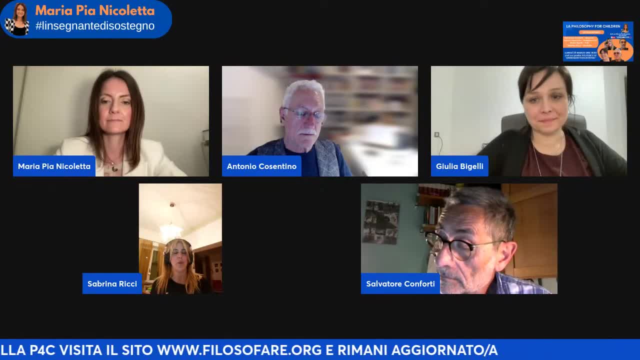 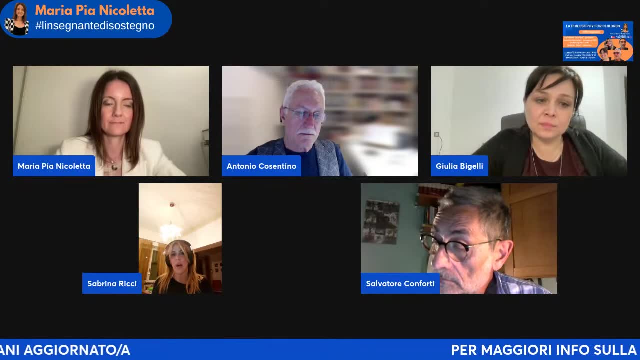 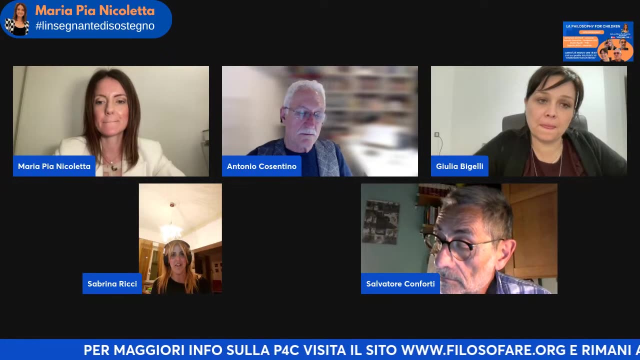 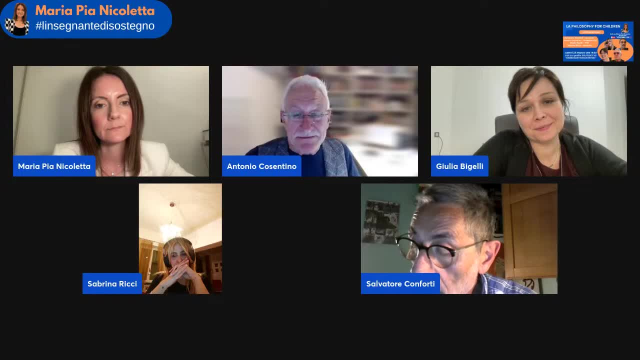 and I saw, in short, I touched with my hands how much the Philosophy for Children can be a great opportunity for children fermarsi, ma non del tutto. no, è un camminare lento. vogliamo chiamarlo così: è un camminare lento è un. 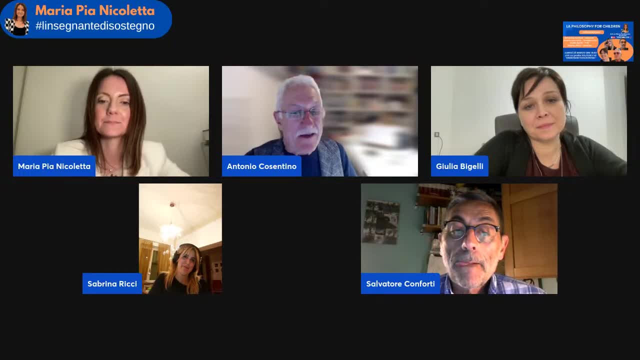 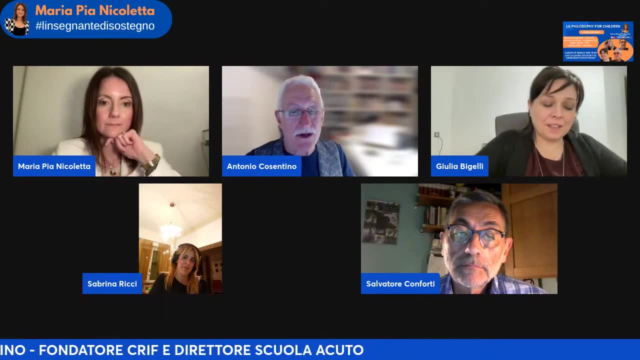 stare nei processi anziché inseguire i prodotti. la scuola di oggi è una scuola funzionalista. possiamo chiamarla no, è una scuola dove gli obiettivi vengono. vengono hanno matrici che 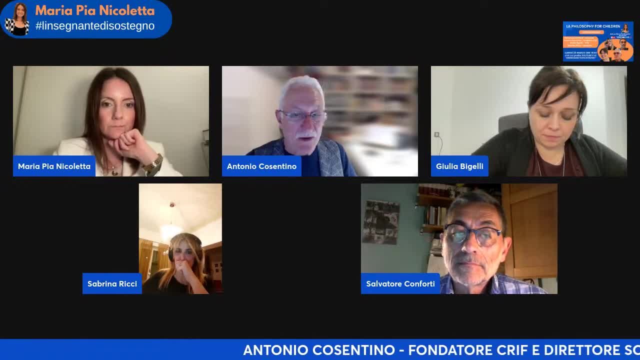 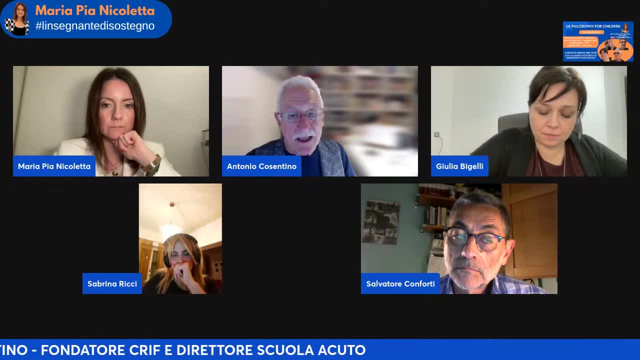 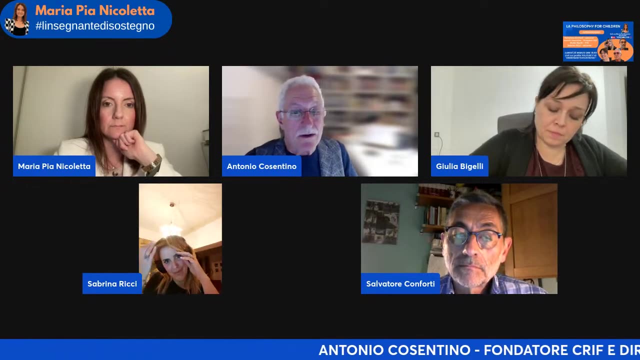 non sono pedagogiche e culturali. sono matrici esterne, non la politica, ma soprattutto, oggi, i mezzi di comunicazione di massa. e che mezzi comunicazione di massa? adesso le piccole chiamano le tecnologie, l'informatica. viviamo in un mondo, in due mondi: quello quotidiano, quello. 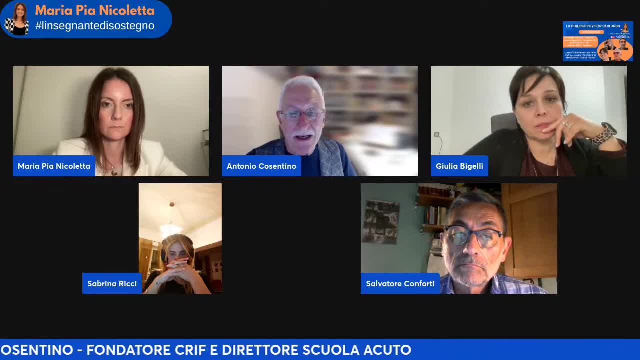 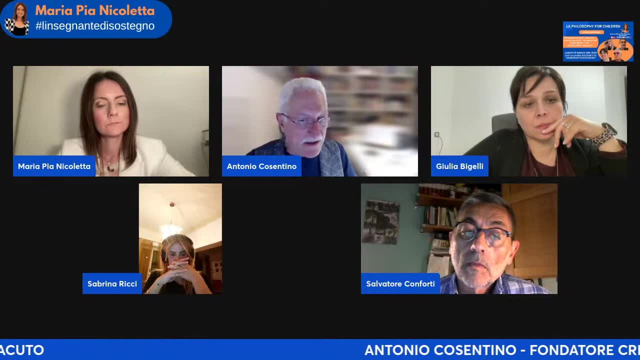 dove i bambini si incontrano, nella scuola, classe. però viviamo anche nell'infosfera e questo naturalmente comportano molte, molte implicazioni. direi che la filosofia ci serve a consolidare, rinforzare, a tenere vivo il legame. 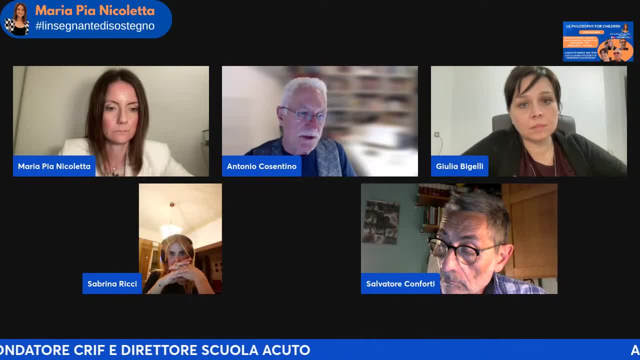 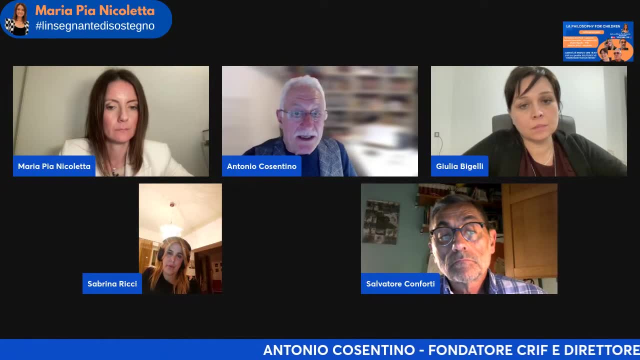 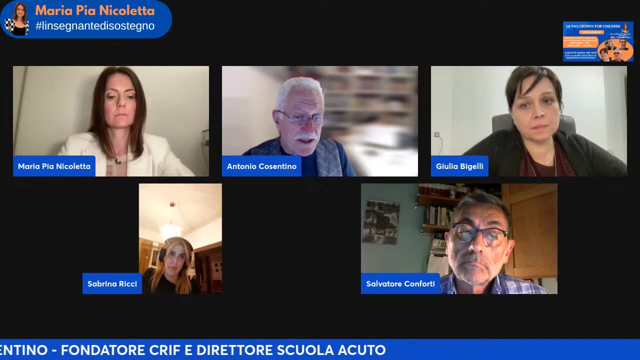 col mondo del corpo, col mondo delle emozioni, con molto delle relazioni col mondo del l'esserci. no, perché credo che sia importante da via valore. per esempio, pensiamo semplicemente all'educazione civica. o l'educazione civica la puoi fare anche su, su wikipedia, se la intendi come una serie di. 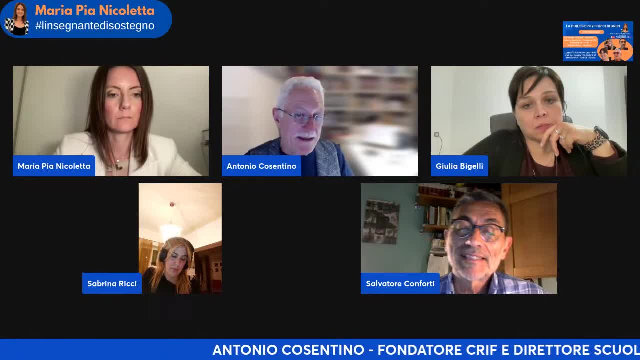 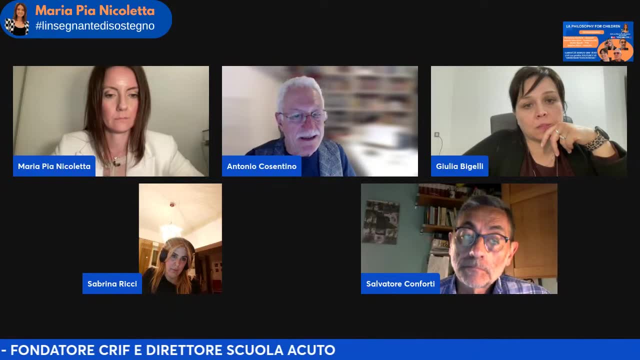 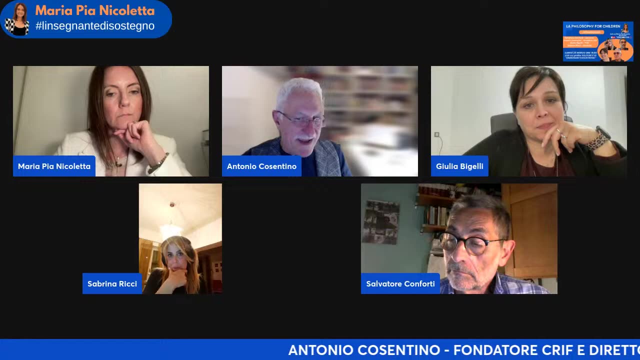 nozioni su come vivere in democrazia, leggere gli articoli della costituzione. ma se vuole essere invece un esercizio di cittadinanza attiva, partecipata e responsabile, la puoi fare soltanto in un ambiente che socialmente è presente e ti chiede. 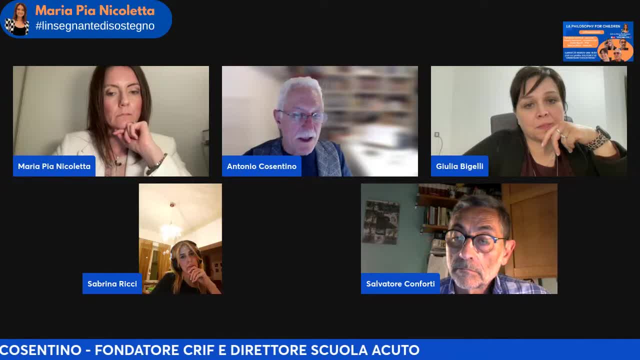 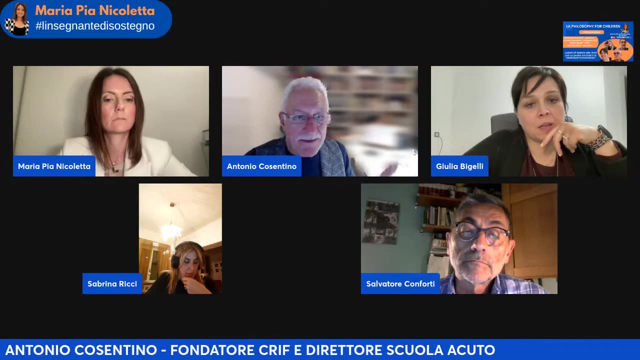 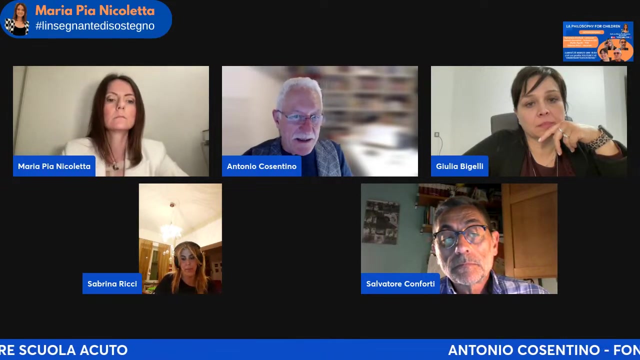 responsabilità quando tu vai su internet, su un social media, social medium, ti presenti come un avatar. un avatar è e non è responsabile, perché io l'avatar, sappiamo, non significava nella filosofia indiana, era il dio che si incarnava in tante forme, prendeva tante forme e questo 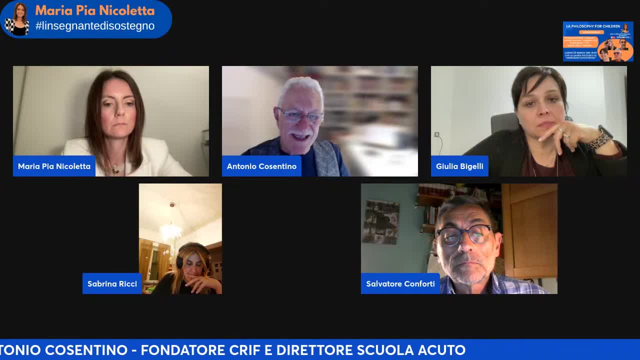 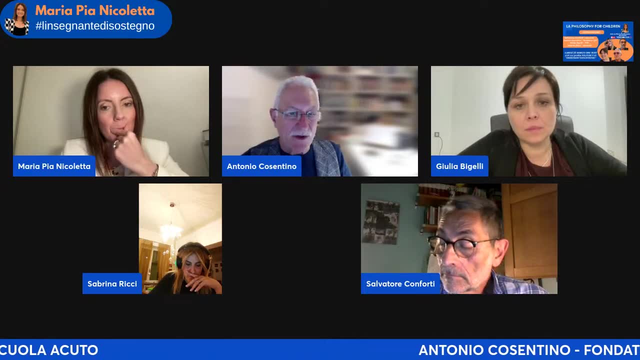 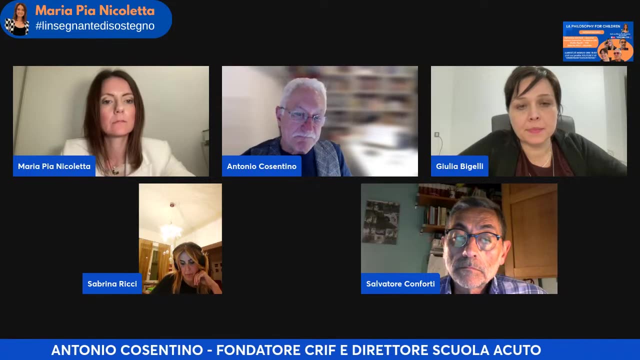 social media ci permettono di essere dei dei che si costruiscono le volte in volta delle identità differenti, ma in quanto avatar non sono responsabili e sappiamo cosa succede, infatti. da questo punto di vista, quindi, allora, la, il fermarsi, la presenza, l'abitare un contesto è 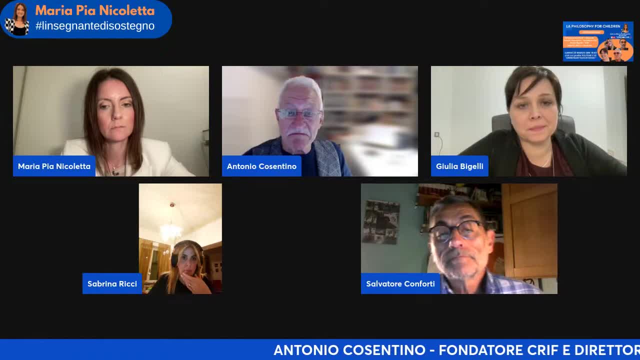 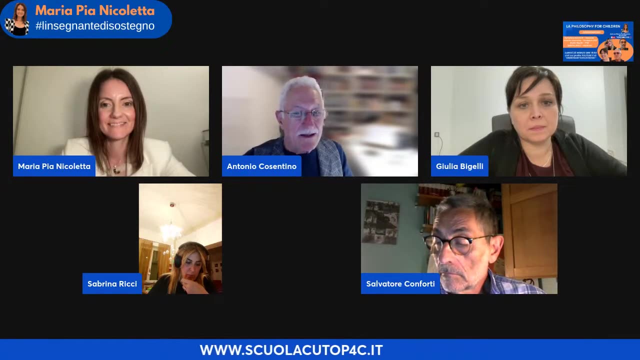 fondamentale nella filosofia cittadina e credo che sia un contributo importante anche, appunto, di compensazione, nella formazione dei ragazzi che vivono in un mondo che invece li trascina più nell'altra direzione. volevo aggiungere soltanto una cosa: che tutto quello che 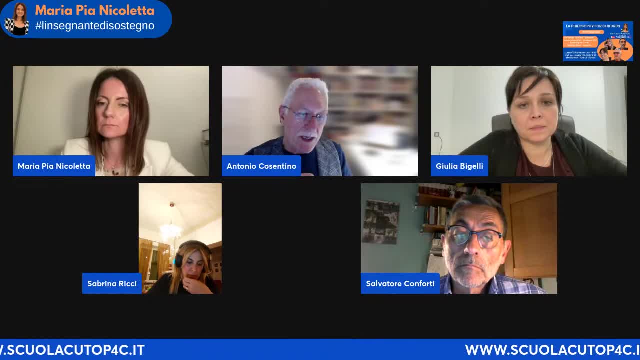 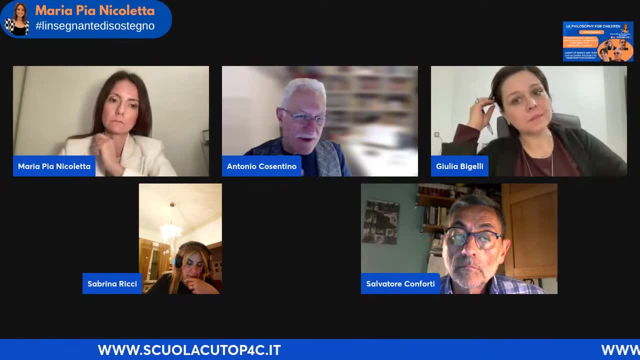 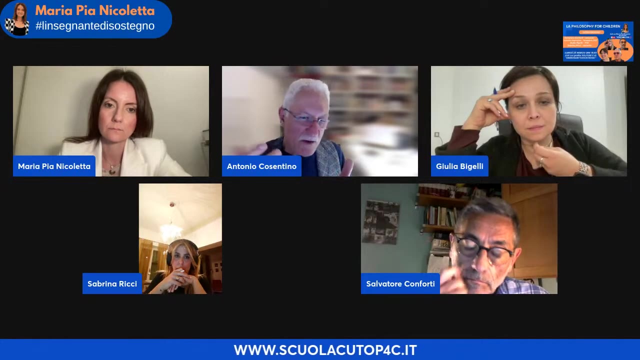 si può fare con la filosofia cittadina e si può fare in modo armonioso, mettendo insieme, appunto, richiami che, come diceva Sabrina, possono andare da diui a Brunner, a Freire. a dominare. ci troviamo tanti ingredienti, ma perché come possono stare insieme? perché non 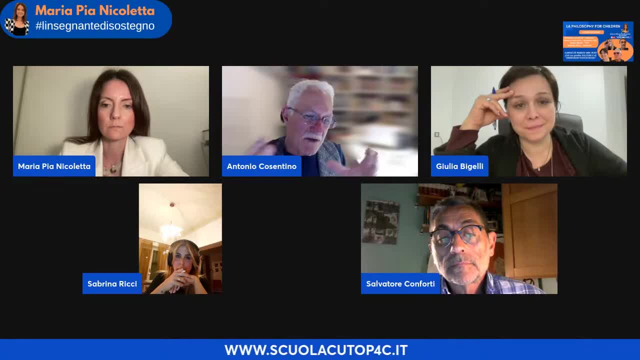 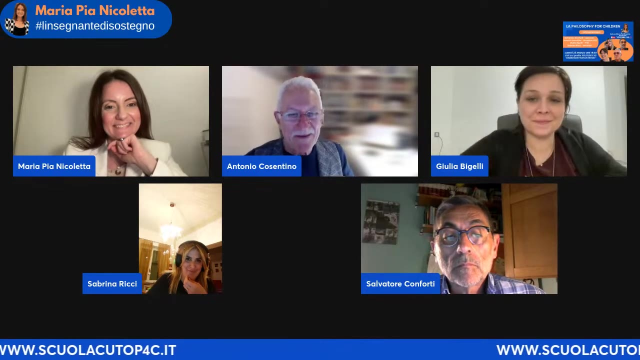 sono teorie, perché non è una teoria. è una teoria molto possibile, vaga. è una pratica, fondamentalmente è una pratica. è una pratica che ecco. P4C forse mi piace più di filosofo cittadino perché filosofo. 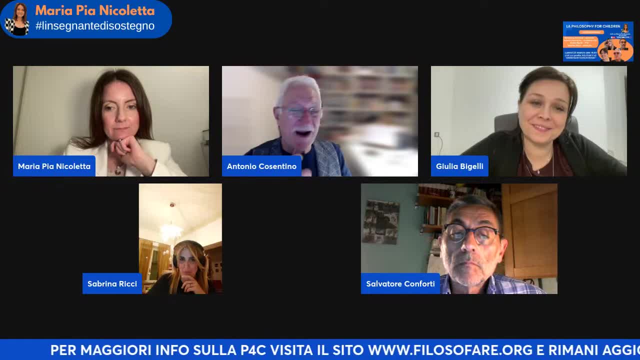 per i bambini il giocattolino: no, oppure la banalizzazione della grande filosofia per i bambini: no. non è questo, l'abbiamo già detto prima. però P4C è una, è un acronimo, ma può essere anche. 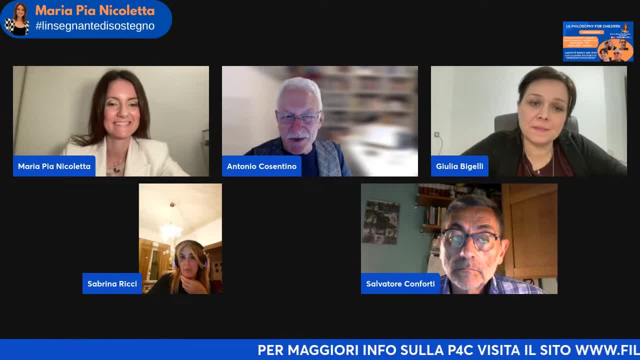 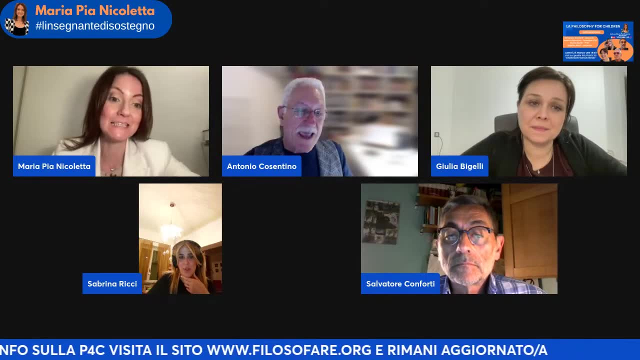 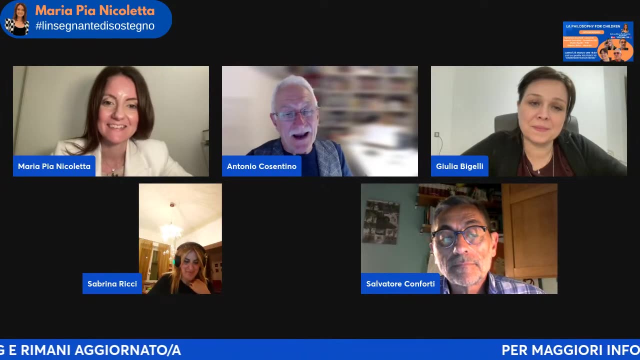 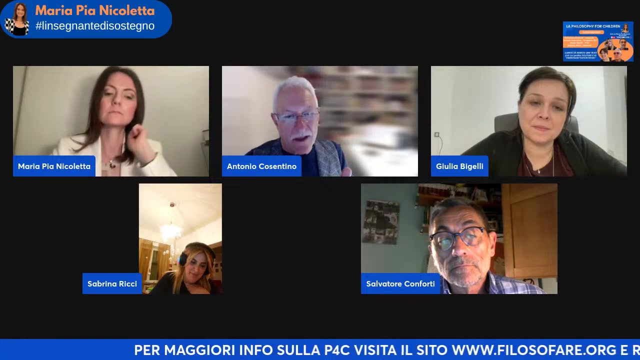 praticare le 4C, per esempio. e le 4C possono essere la comunità, la cura, la comprensione, la creatività, ma anche qualche altra cosa ancora, bello, bellissimo. questa definizione mi piace, tanto è una pratica. allora aggiungo, e finisco dove l'insegnante che noi chiamiamo facilitatore: 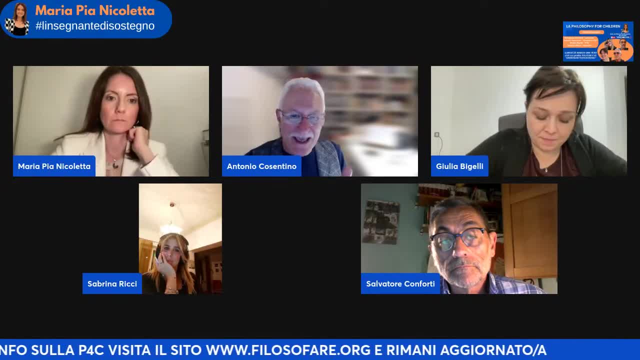 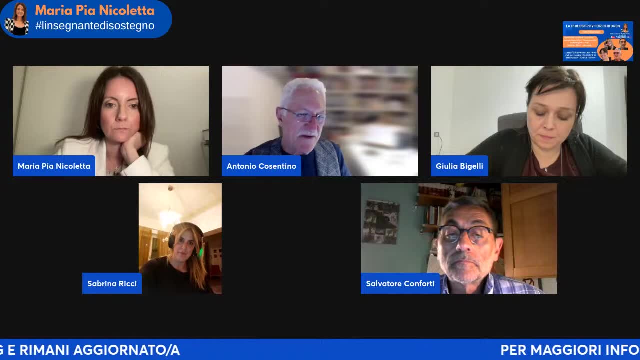 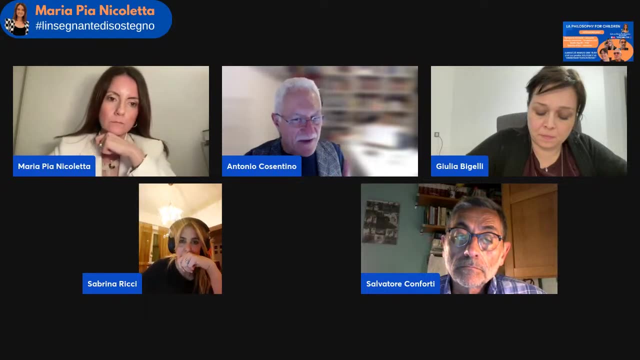 facilitatrice gioca un ruolo che è tutto diverso. quindi la formazione degli insegnanti è molto importante per farla bene. farla bene significa fargli consentire che dia i suoi frutti migliori, ed è un lavoro, quello che si fa all'acuto, quello che si fa nei corsi di formazione. 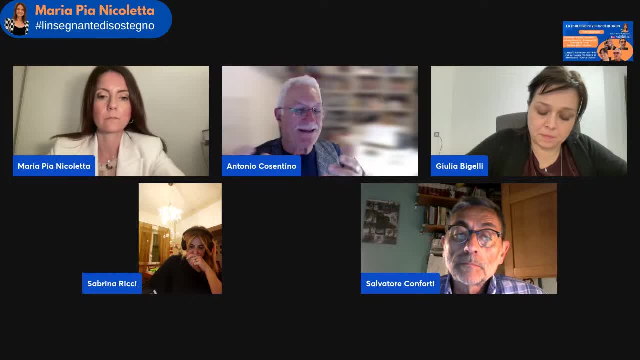 dove non c'è da apprendere grandi cose nuove, c'è da lavorare su se stessi per liberarsi di tutte quelle incrostazioni che la scuola tradizionale ci ha dato come insegnante, perché ci ha voluto. 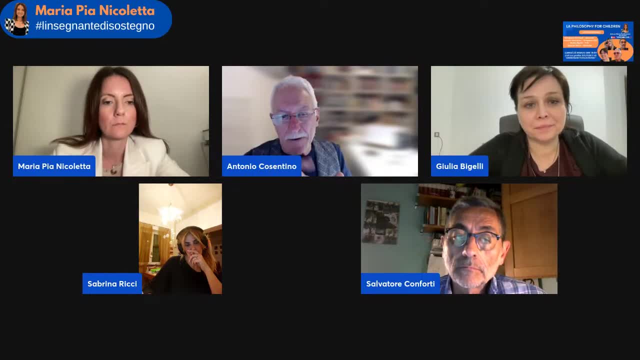 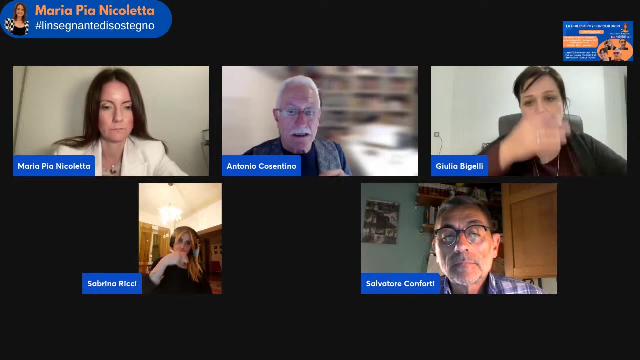 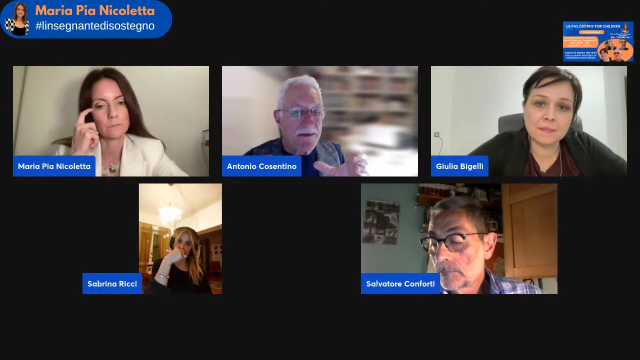 formare come trasmettitori, come controllori, valutatori, sacerdoti di qualche disciplina, questa scuola, che è nata nel settecento, insomma, che ancora continua a far sentire i suoi effetti su molte persone, bastano questa scuola. la scuola è un ambiente, un setting che è progettato ed è. 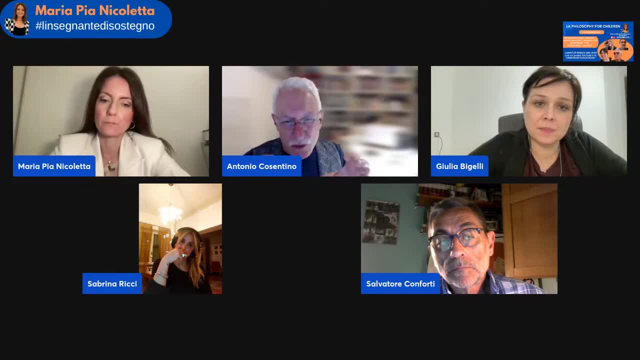 tenuto vivo, custodito in maniera consapevole da quello che è la figura, appunto, del facilitatore, della facilitatrice che non deve insegnare ma deve creare e saper tenere in vita, consolidare, tenere attivo, animare un ambiente che permette. è uno scaffolding, un. 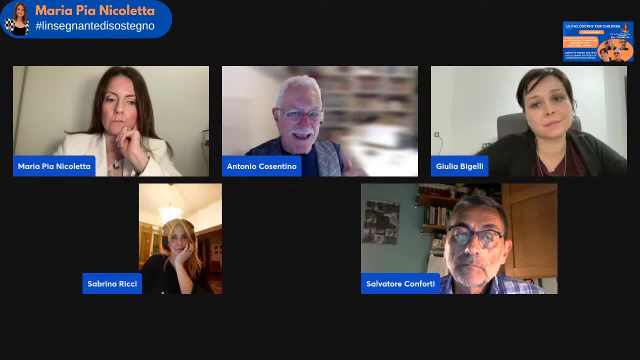 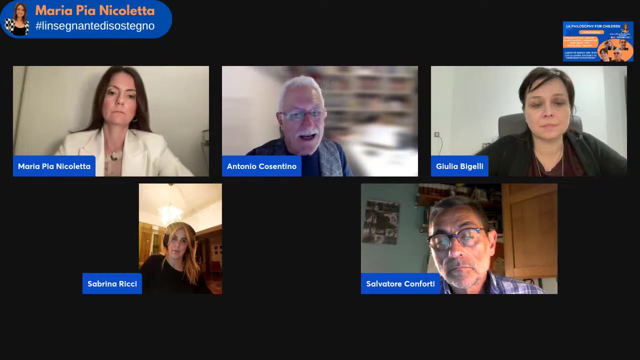 supporto, poi tu fai l'impalcatura, ma chi sale sull'impalcatura dovrà costruire autonomamente i suoi guadagni informativi, la sua, costruire la sua identità, la sua, la cura di sé nel confronto con gli altri. e questo è, e questa è un'educazione, secondo me, della scuola. 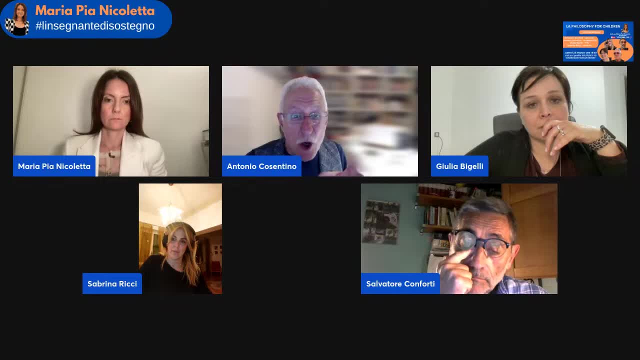 del futuro, dove le nozioni devono sparire dalla scuola. ingombrano, stanno fuori stanno. ci sono mille fonti, quindi la scuola o chiude o fa qualche altra cosa, che può essere qualcosa del genere. 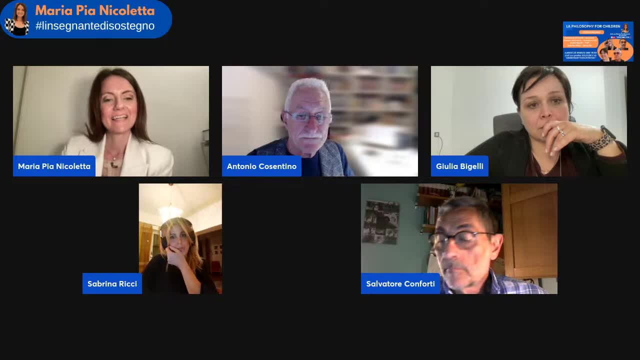 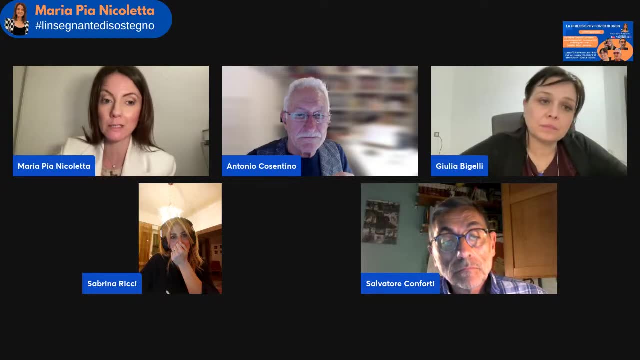 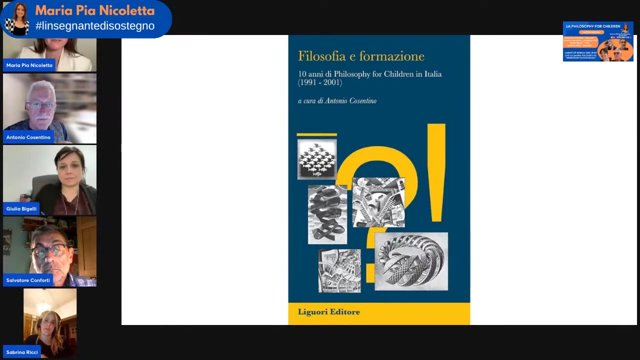 grazie, antonio. mi piacerà lanciare qui in grafica alcune delle tue pubblicazioni. sono tante. eccola qui. filosofia e formazione. dieci anni di philosophy for children in italia. ecco questa cura di antonio cosentino. 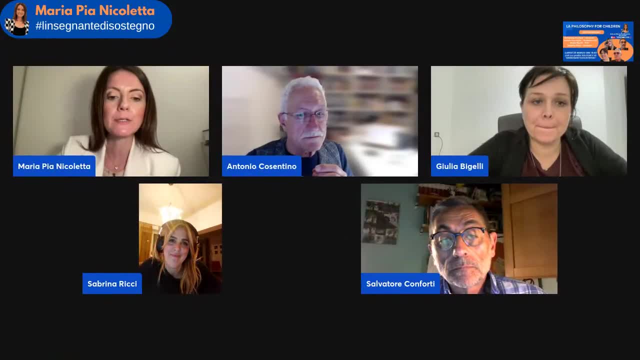 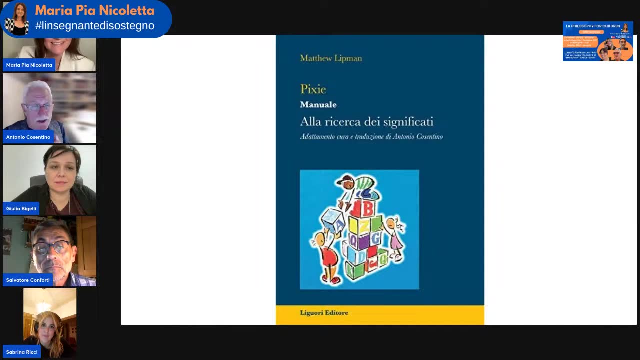 punto liguori editore. poi ne lancio un altro. eccolo qui, pixi, è un manuale, no e curriculum. dove si volesse potesse consigliare una lettura introduttiva ma anche sintetica. tra le cose che ho, 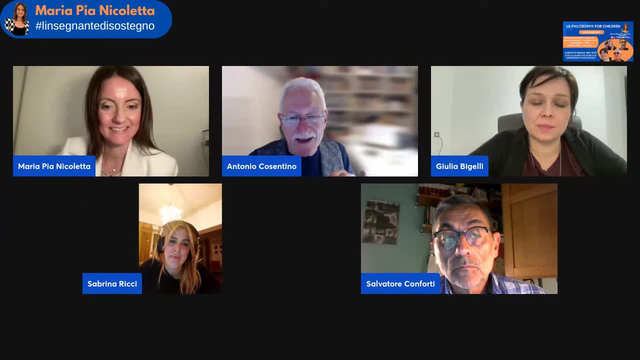 scritto. io vi consigli, consiglierei a chi ci ascolta questo libricino pubblicato da anice, che si chiama didattica della comunità di ricerca, perché racconta un percorso, quindi è una narrazione. 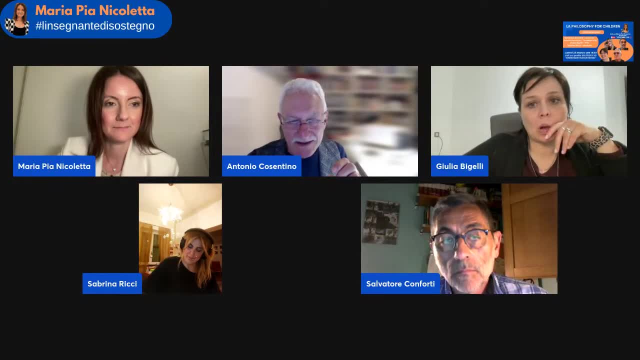 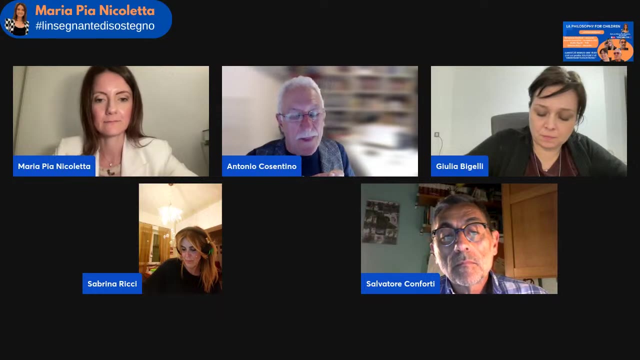 la storia. la storia l'abbiamo vissuta e costruite, salvatore, quello raccontate io, insieme a maria, contributed with a part of the book and therefore there is the story and the teacher who wants to understand maybe understands better through the narration of meeting, by meeting what happened. 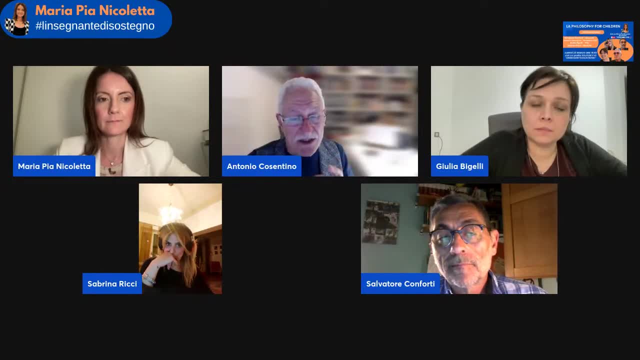 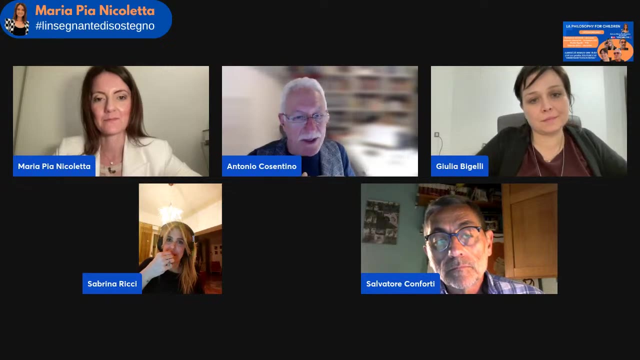 what was the difficulty, what we did? and then there is this theoretical framework that takes up a little the things that have been written on the other books. socrates, after all, is one of the most recent texts where I turned more to philosophers in the academic world to say that the philosophical practice 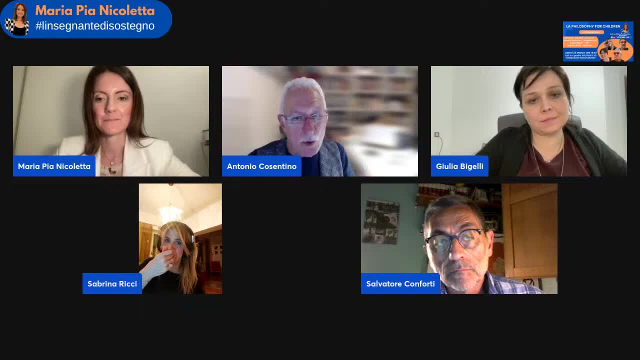 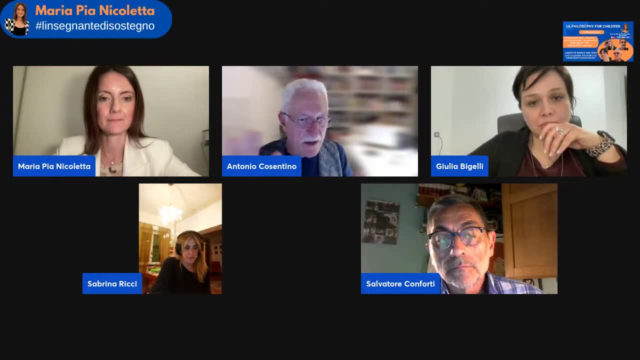 was the way in which philosophy was born, in a theme with socrates, who did something like that we do not want to do as soon as another, but he spoke, he confronted people, he asked the person to assume the responsibility of what they said. then philosophy took another. 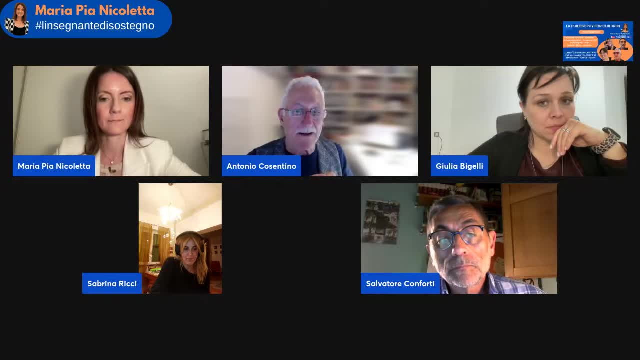 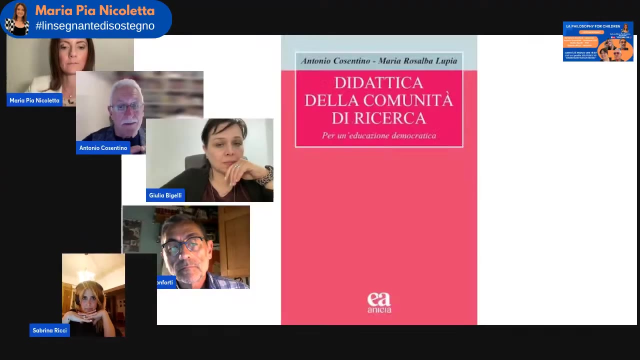 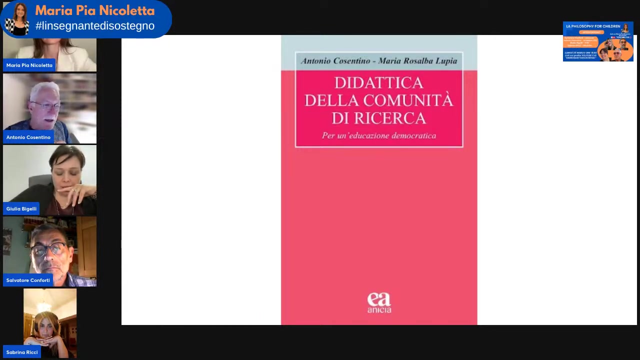 path which was dictated by the first act of writing and that has become books, has become a discipline, their language, their complicated lexicon, etc. etc. but the why is it forced? it wants to bring back in life the Socratic evidence where the dialogue is not more than two, polyphonic, etc. etc. there are various differences, but 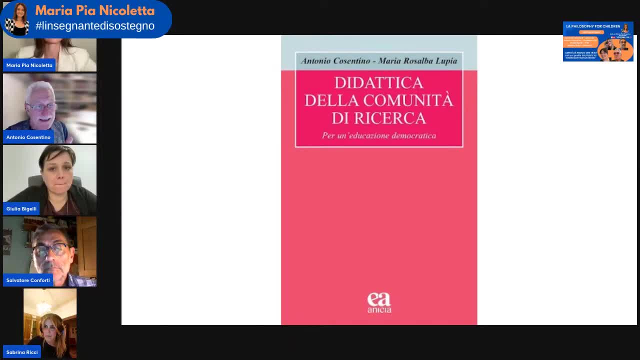 fundamentally, this is the philosophy before being written- is a practice of dialogue between people, where you confront yourself not on your own opinions, but on the reasons of your opinion. on the reasons of your opinion. so it requires arguments, that requires the use of discursiveness against what we see today in the talk show. I tell you the truth, which is: 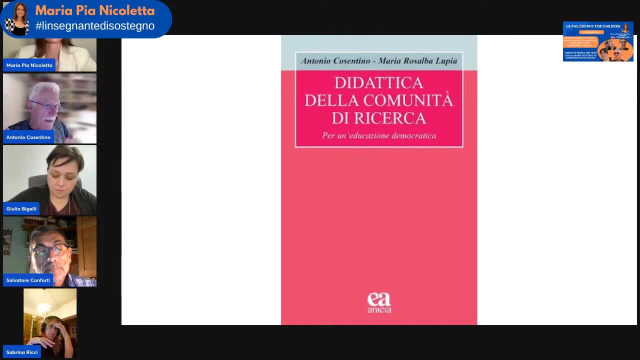 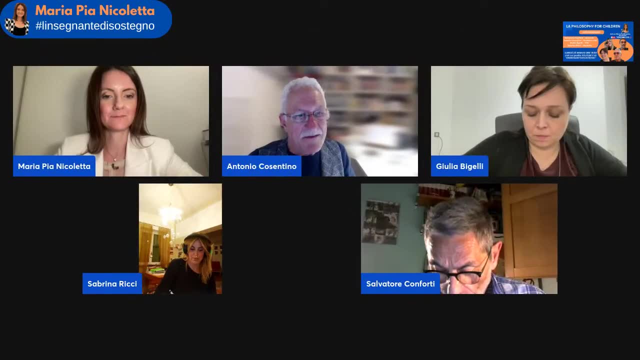 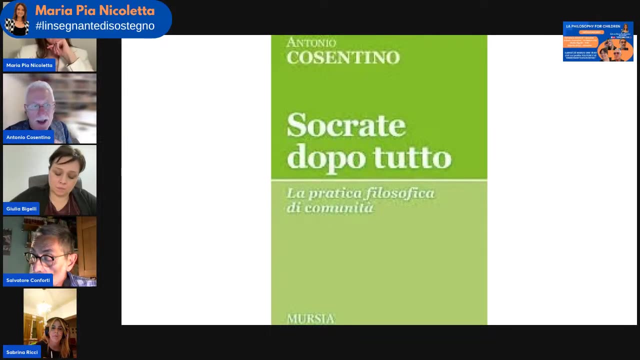 and if you do not understand it, you are an idiot. this aggressive way of confronting yourself that never requires an argumentation. this is, in short: it brings wars and we have it perfect thanks, antonio. in the meantime, I let the texts that you recommended here in the graphic flow and I would pass the 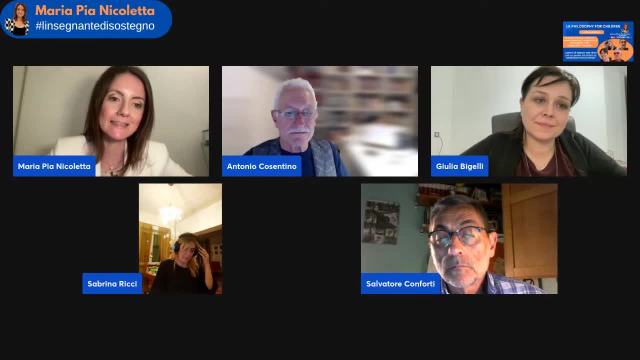 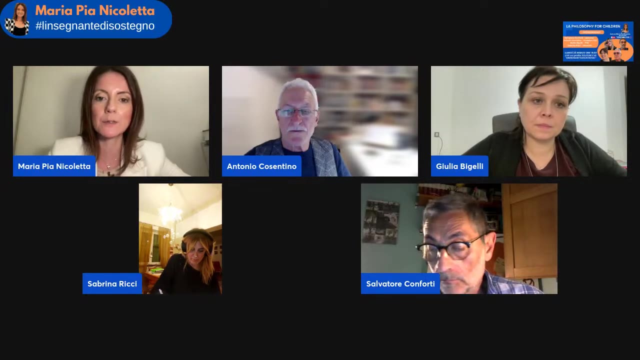 word again to the doctor, giulia bigelli. we talked about it a little earlier. here is how important it is to apply the philosophy with children for a better environment, to make schools in a new and different way. so, giulia, the philosophy for children, we do not have to study it only for competition tests, and keep it only. 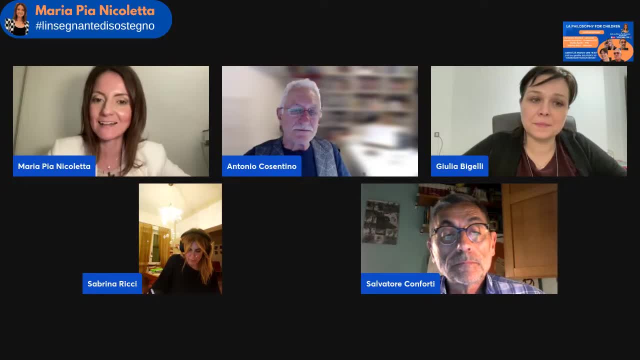 as a theory, but it is possible to practice it, it is possible to apply it. but I agree with antonio, the training is essential. but precisely because, among other things, today there is so much literature, there are so many initiatives of philosophy for children, with children, of children, and 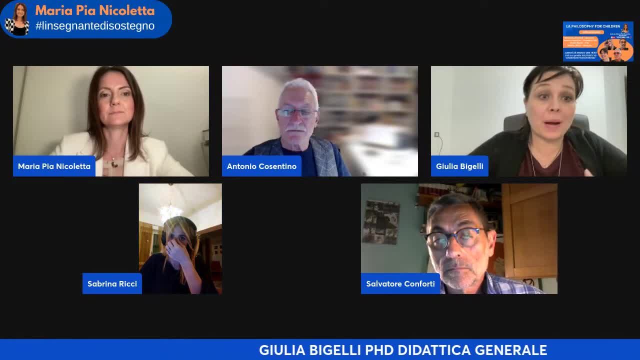 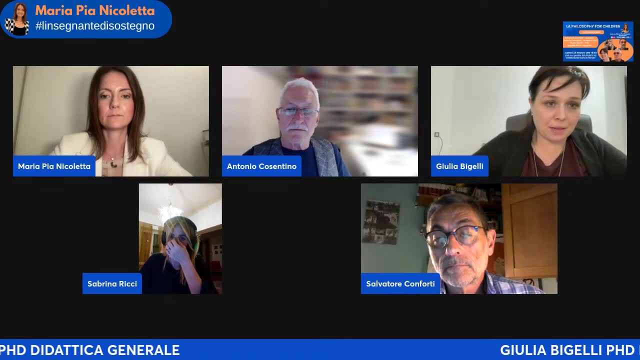 therefore, you have to say how to say: have a good baggage and, above all, a good awareness of yourself, because, because it is true, everyone can do philosophical practice, everyone can do philosophy for children, but I would add, however, all those who actually put their own style of thinking into discussion. but the 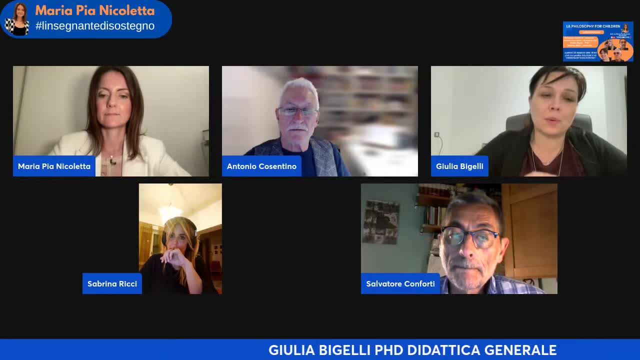 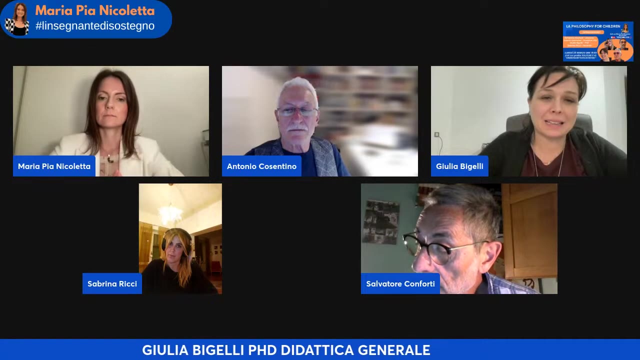 classroom of teaching and put it into discussion, but really the provost, how to say? being a teacher, I am very convinced of this because, because there is still a decentralization of the teacher in the van in the philosophy for children. we must be a little in the time of the for their children. it discards not what. 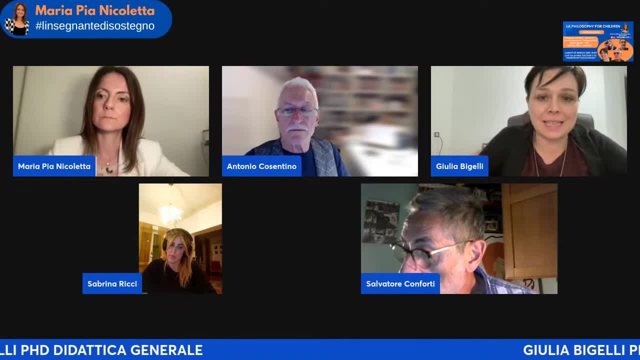 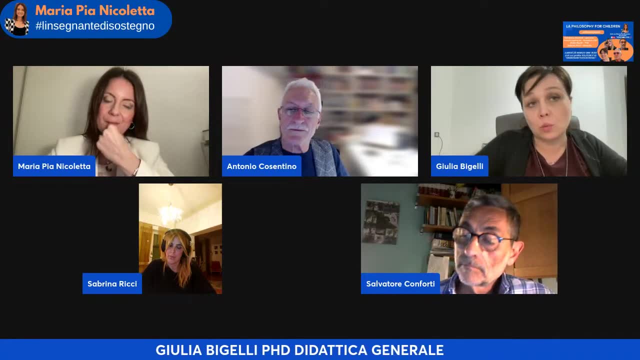 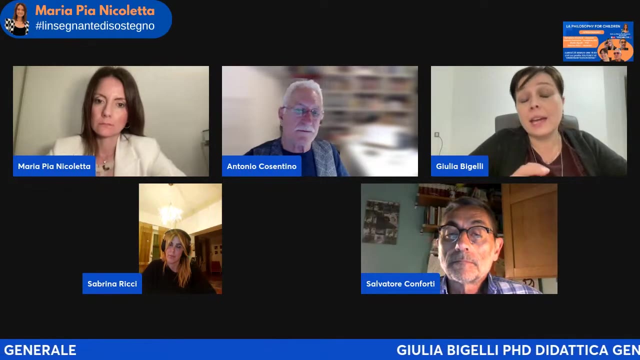 the traditional school is. it is flipped over the classroom in what sense that in reality there is no more a classroom, because the teacher becomes a facilitator and becomes them also a builder, a constructor of conoscenze, di flusso di pensiero, insieme ai membri della comunità di ricerca. e questa non è una cosa. 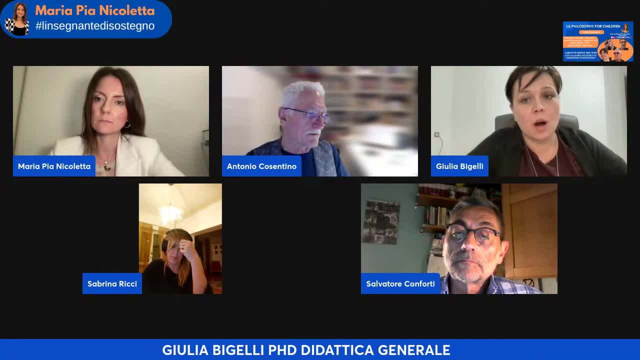 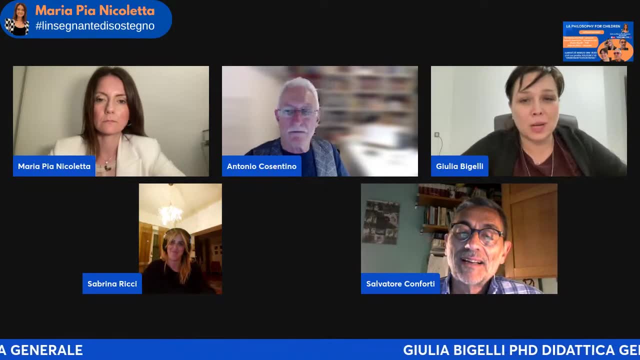 scontata, secondo me, oggi come oggi, non nelle scuole, dove dove realtà ancora ci viene richiesto di finire il programma, di compilare registri, soprattutto nella scuola primaria. io ho l'esperienza sia nella secondaria che nella primaria. la scuola primaria è piena di burocrazia. 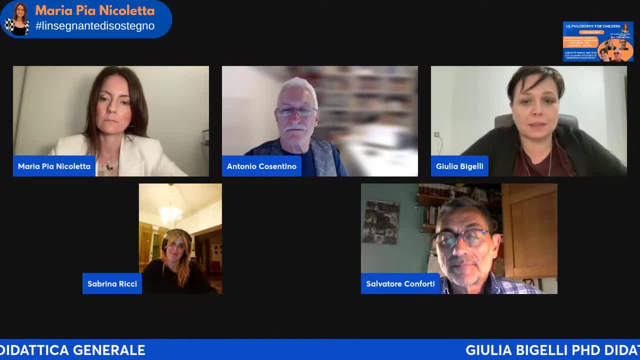 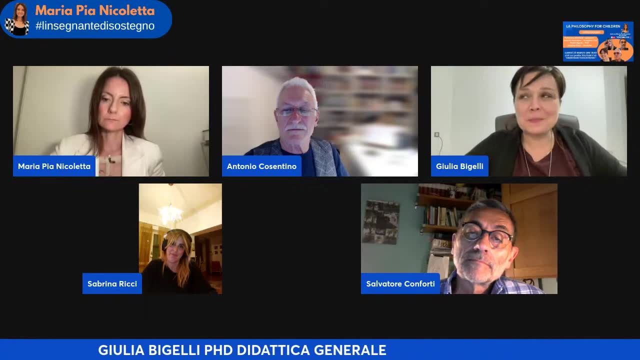 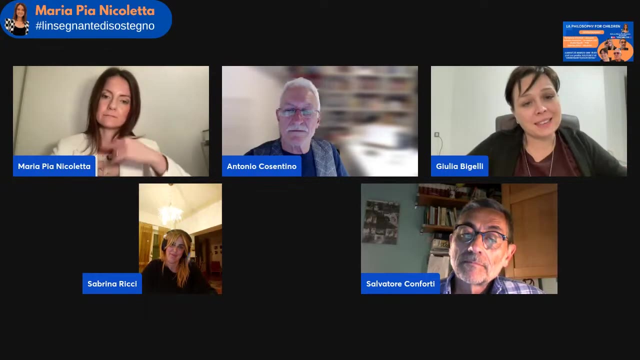 e ci sono i registri, c'è di tutto. veramente tanta programmazione lente, quindi è come dire difficile, no, anche riuscire però a mantenere, o meglio a coltivare un essere docente che non venga risucchiato da tutto questo. prima non toglie, diceva la filosofia, richiede presenza. 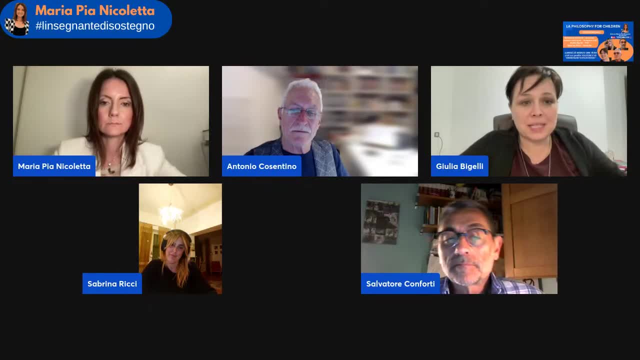 no, io sono molto convinta di questo. richiede presenza ai bambini che ne abbiamo in classe, che ogni giorno arrivano. no, sono lì con loro la loro vivacità, con tutte le loro differenze, con tutte le loro caratteristiche, i loro talenti. noi delle 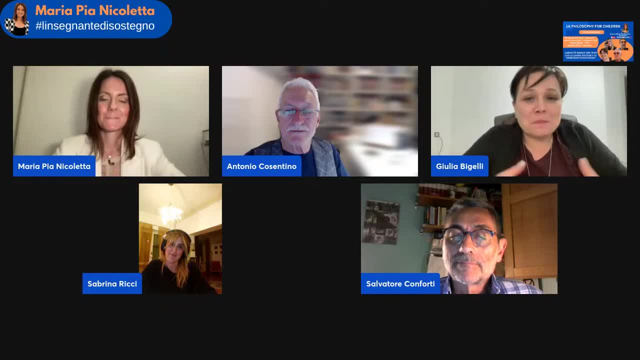 volte riguardo e dico chissà? no, tra di loro veramente ci sarà un futuro? non so medico, un futuro di tutto no. e e allo stesso tempo richiede la presenza del docente heidegger ci dice: diceva che cosa? no, che essenziale è l'essere. 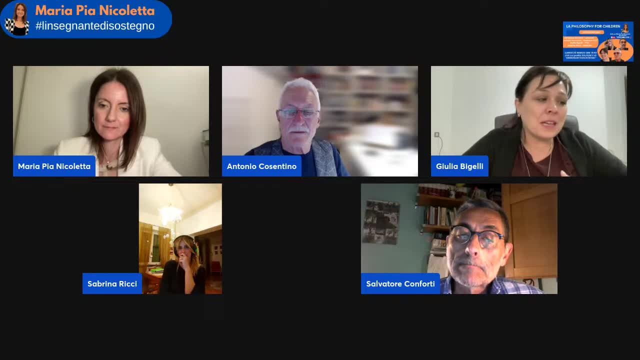 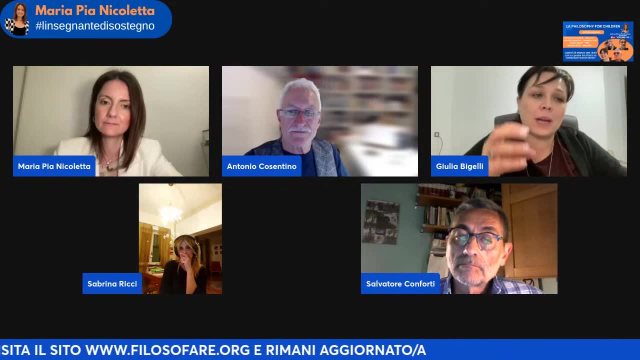 c l'essere c inteso proprio come quel quell'essere gettato no, nel qui e ora. e io credo che la, la filosofia for children recupera proprio quel, quella particella no, quel c che poi la progettualità, cioè 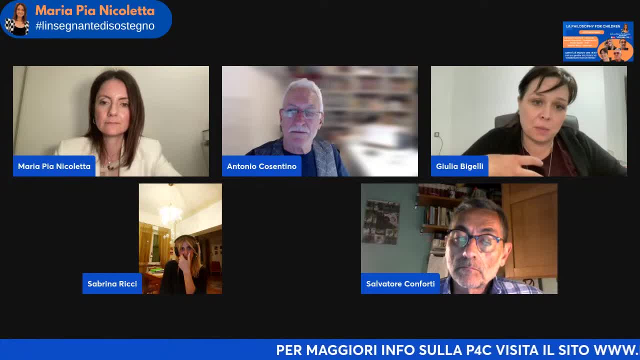 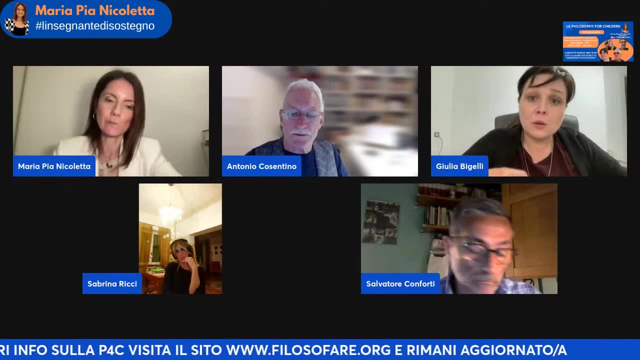 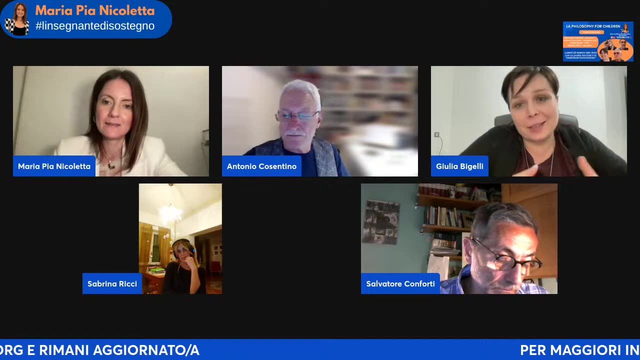 io sono nel qui e nell'ora e sono consapevole di me, dei miei pensieri, sono consapevole delle mie emozioni, del mio corpo e solo quindi, lavorando su questo, posso davvero costruire ad un altro come docente e e quindi, anzi non e, ma con i bambini che comunque io in classe, 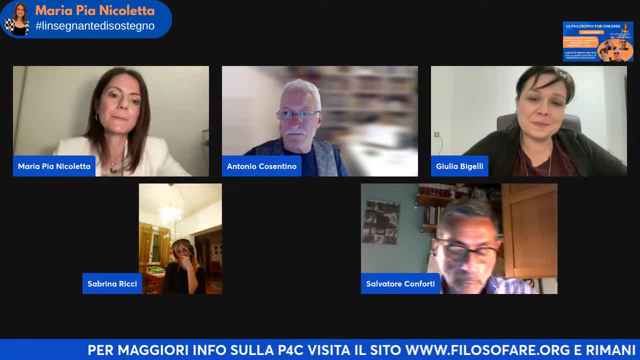 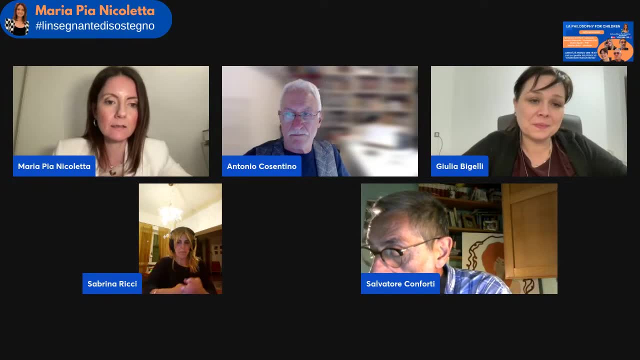 grazie giulia. ci apri gli occhi su delle realtà che sono possibili. batterebbe davvero mettersi di un buon impegno, entrare in classe con un'ottica diversi, ma non quella di completare le scartoffia. che se passatemi il termine, ma quella di mettere in classe certissimi e altri cambiamenti, peretera scatologia che se passatemi termine, ma quella di completare le scartofie che se passatemi il termine. 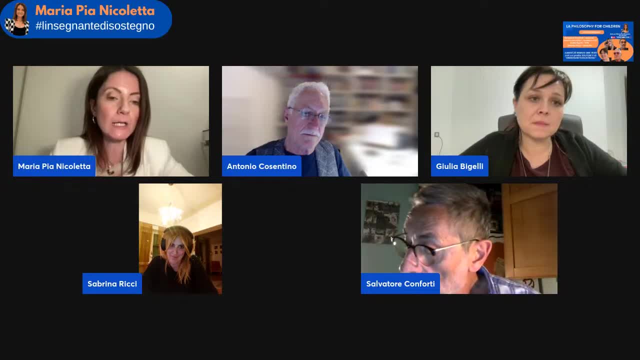 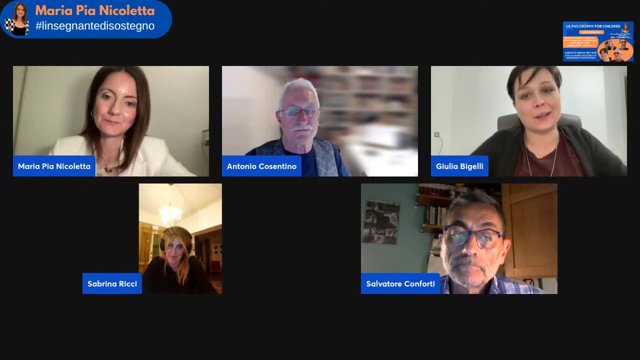 consapevolezza che davanti abbiamo dei futuri, il futuro della nostra società, dei futuri specialisti e magari attraverso la philosophy for children avranno anche maggiore consapevolezza di sé, di cosa vorranno essere Assolutamente, proprio perché si lavora sull'identità anche. 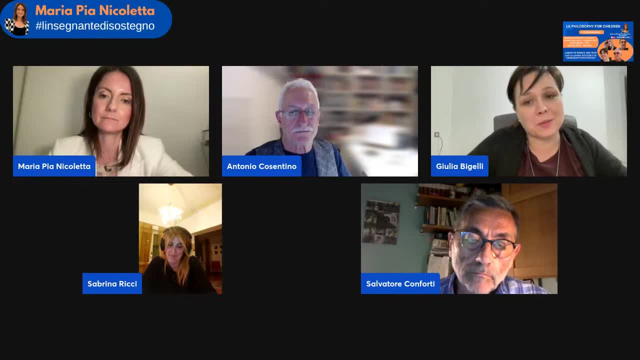 sulle proprie competenze, sulle proprie abilità. come diciamo prima: il mio pensiero vale io algo? no, Anche io ci sono. Grazie davvero alla nostra ricercatrice Giulia Bigelli Salvatore. 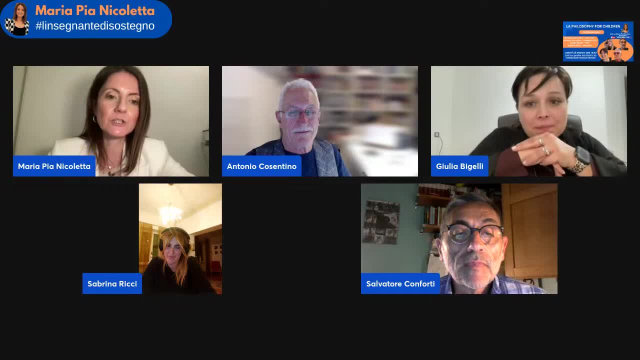 torno da te. Avevi lasciato in sospeso un discorso che volevi terminare. ecco a te adesso Il discorso a terminare. volevo soltanto lasciarvi con degli esempi concreti, perché Giulia e Antonio, 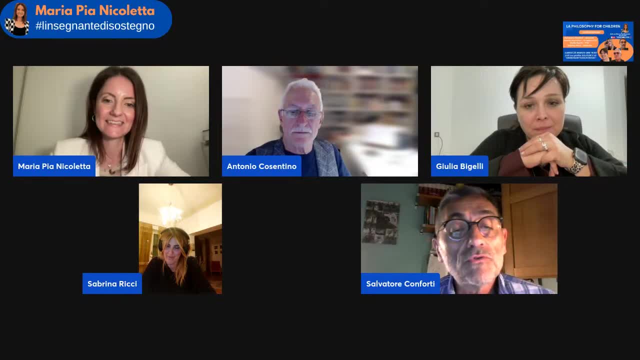 sono due teorici ai quali bisogna aggiungere poco. Sono chiaro che, come dicevo prima, sono due teorici ai quali bisogna aggiungere poco. Sono chiaro che perché Giulia e Antonio sono due teorici ai quali bisogna aggiungere poco. Sono chiaro che 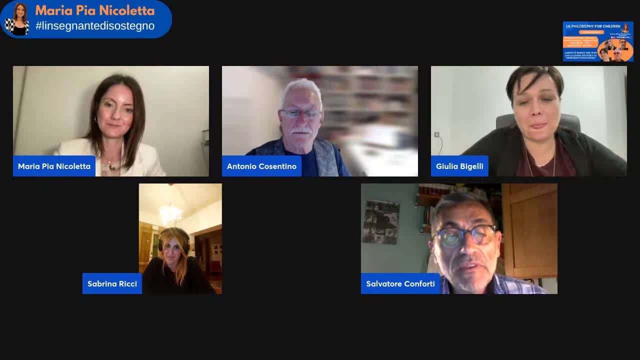 perché Giulia e Antonio sono due teorici ai quali bisogna aggiungere poco. Sono chiaro che diciamo che sono, come dire, esemplificano quanto più possibile per far capire a un pubblico che magari si occupa di scuola, ma pure per chi non si occupa di scuola, no, Nel senso della philosophy. 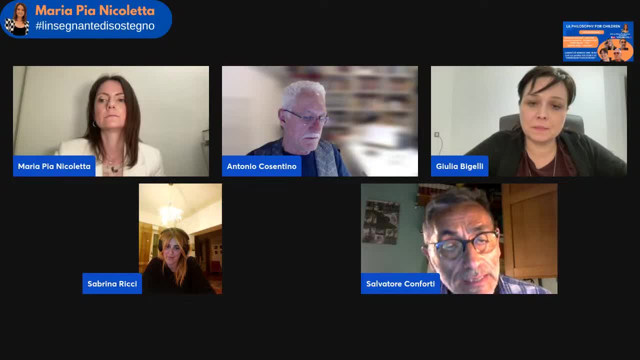 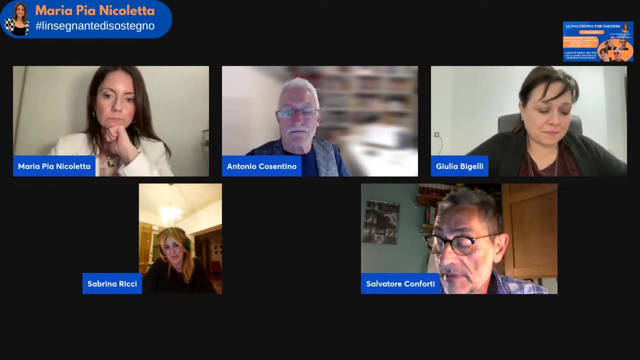 Invece voglio lasciare qualche perla proprio dei ragazzini, perché sono quelli che poi alla fine lasciano capire che cosa succede durante una sessione, all'interno di un cerchio. Queste perle sono quelle che poi mi danno la voglia di andare, proseguire, andare avanti in maniera sempre più. 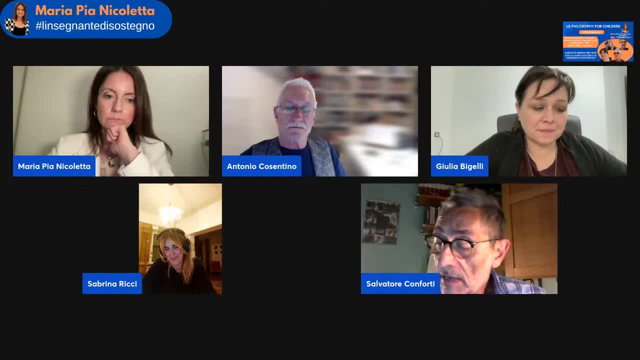 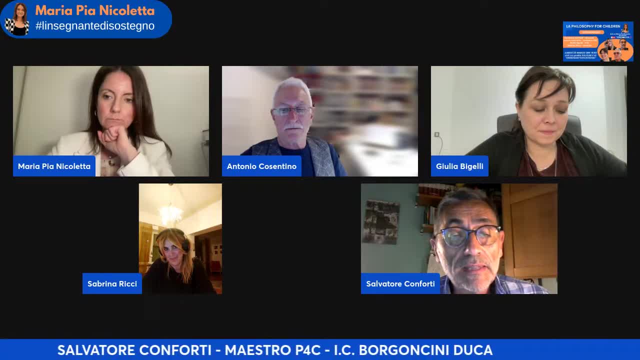 con questa affermazione qui, e ho cominciato chiaramente a mentire, un po' in crisi, nel senso che, insomma, certe cose diciamo, ma come è possibile che possano dirle bambini di otto? 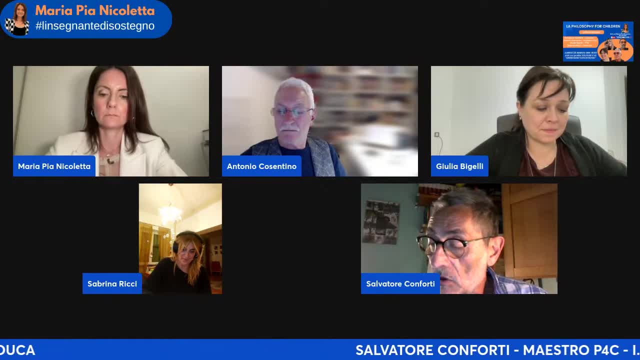 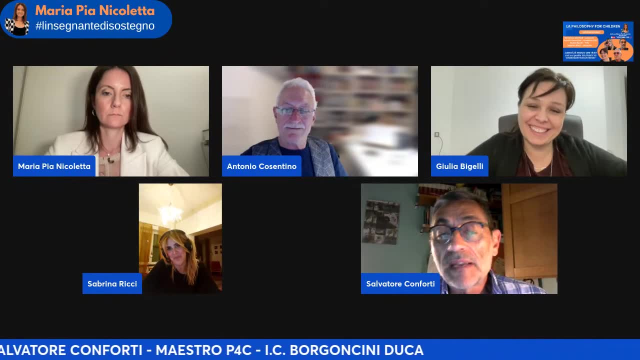 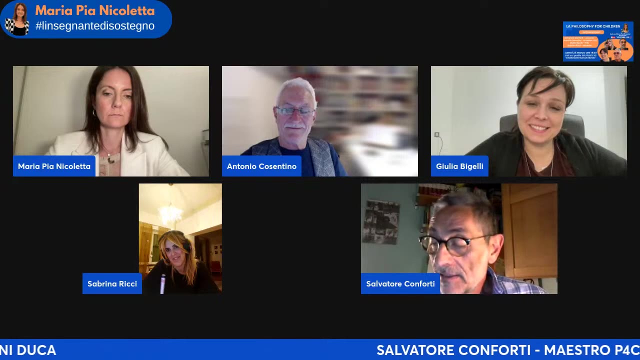 nove anni E lei risposa che il tempo è come un amico egoista che uccide tutti, ma lui non si scalfisce mai. Questa era Maria Vittoria, di nove anni e invece eleonora di sette anni. sembrava praticamente socrates in gonnella. a un certo punto disse: 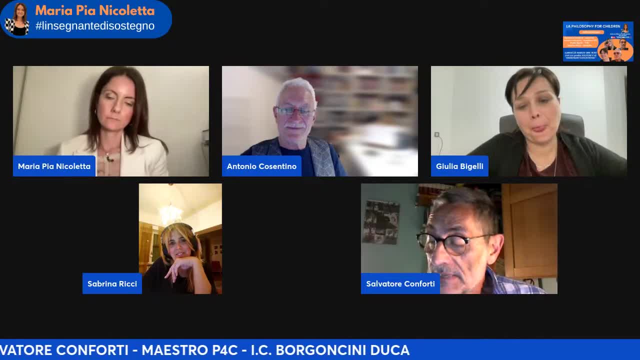 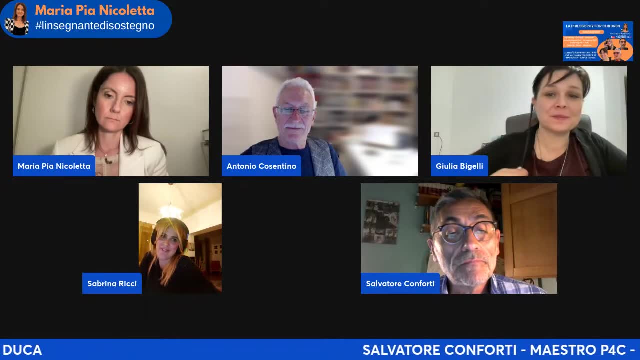 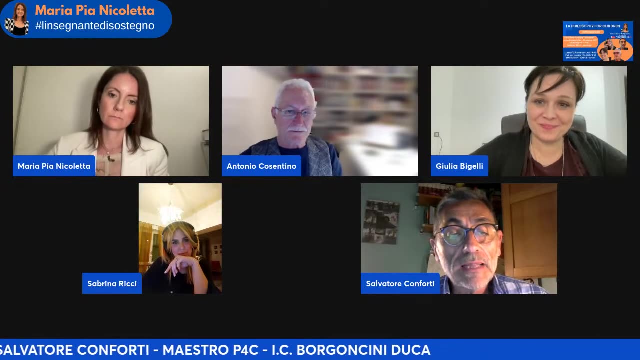 riconoscere di essere stupida rappresenta un punto di forza, perché ti permette di trovare il tuo punto debole e di sconfiggerlo. dunque io dico che a queste perle non bisogna aggiungere nient'altro per capire di cosa si tratta, se non invitare chiunque voglia. 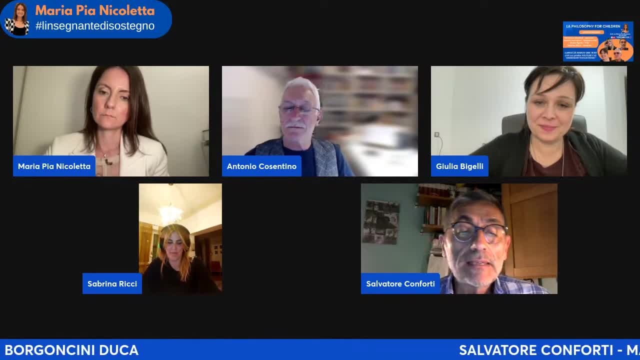 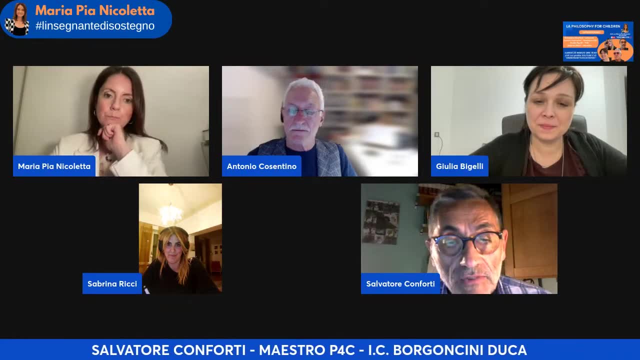 fin da domani, in pratica ad assistere alle sessioni che si fanno da noi in classe. io sono molto commendo quando qualcuno viene, apprezza, capisce, si rende conto, ci mette, diciamo, la faccia, in qualche modo si confronta su quello che noi possiamo raccontare teoricamente adesso per ore. 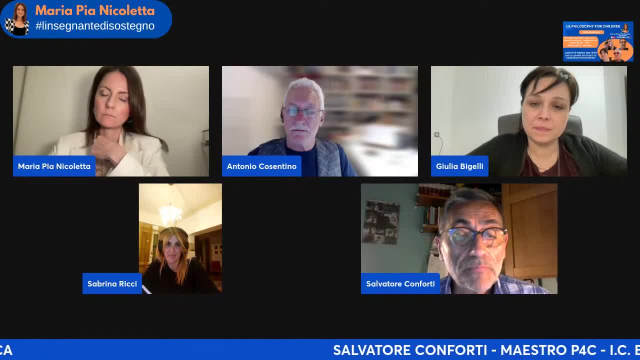 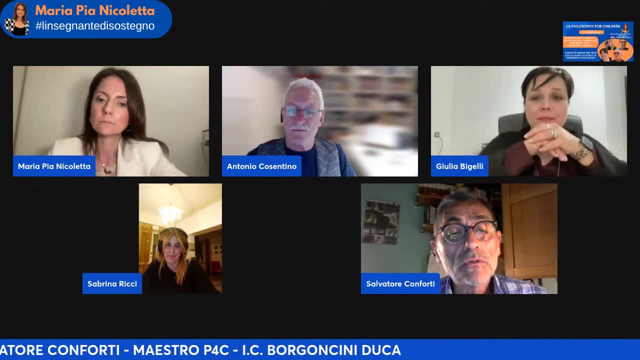 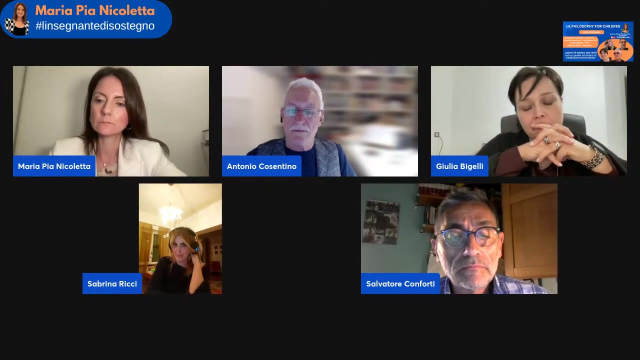 ore, ma non si capisce bene fin quando non si assiste. e prima di chiudere voleva lasciare, diciamo, con due informazioni di significativa. intanto, sabato scorso e nasce la settimana del crif laziale, che si è costituita proprio da poco e più fraziale significa in pratica che 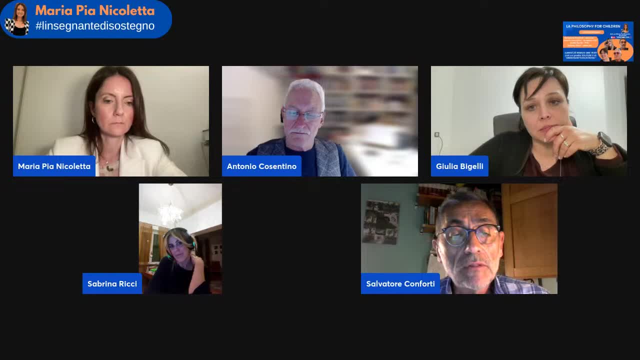 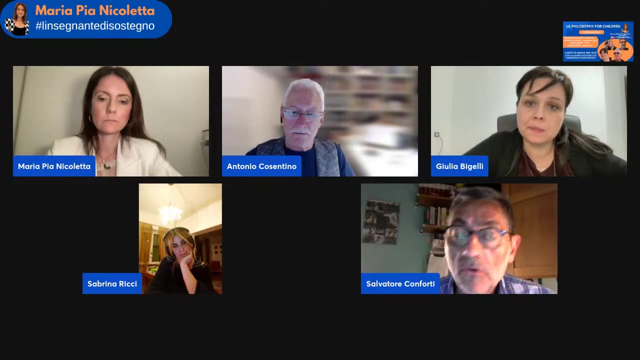 noi adesso abbiamo una certa diffusione, un po ci stiamo allargando in tutto il lazio, nelle province del lazio, dove abbiamo delle collaboratrici e delle professoresse e colleghe di scuola primaria che si sono formate presso il crif e che adesso 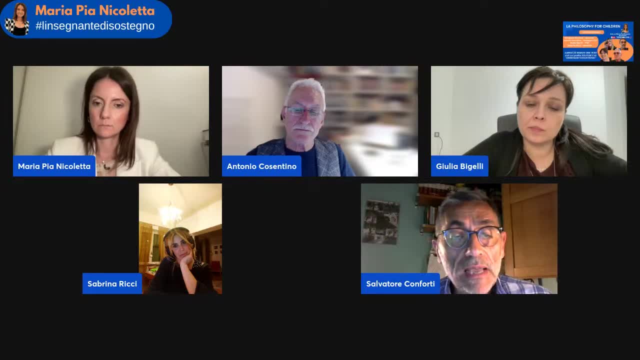 cominciano ad agire in autonomia, essendo una necessità, il bisogno pure loro, dopo aver sperimentato appunto il potere della filosofia di allargare quanto più possibile questa didattica, perché appunto ce n'è bisogno. e poi lascio. 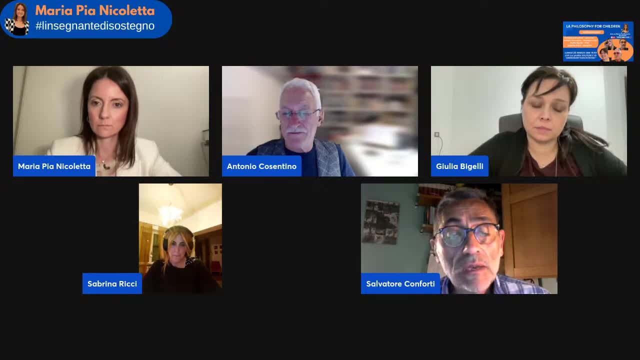 la parola a sabrina dicendo che il 24 e 25 di maggio, presso la scuola di anzio- quindi siamo in provincia- noi abbiamo organizzato il festival nazionale della filosofia, città dove possono in pratica partecipare tutti i giorni che ci sono, in particolare tutti i giorni che ci sono tutti i giorni. 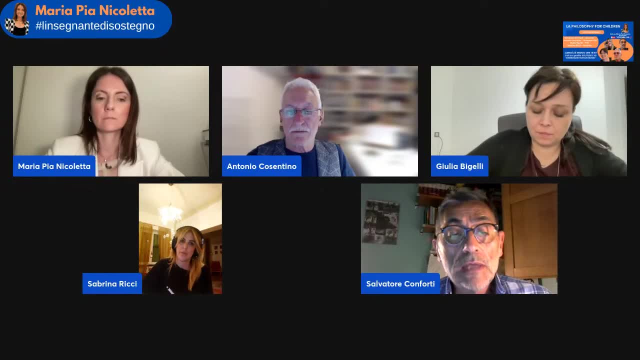 nelle scuole d italia che mi manano richiesta. sul sito della scuola culto avranno possibilità di trovare tutte le informazioni, ma soprattutto sulla locandina si sta circolando un bel po. poi magari te ne mandiamo una dellaடa maglia via così entrati, vedo che anche ho trovo il line. 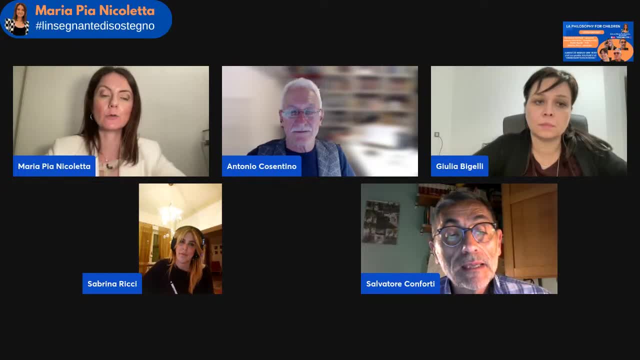 adesso lo pubblico sul banner, così lo possono vedere e lo condividerò anche sui miei social, nelle storie sono volentieri e grazie. e quindi diciamo: questa iniziativa ed Buy chama, ci monito, e molto interessante, perché la prima giornata vedrà appunto 3, 400, forse addirittura 500 ragazzi. 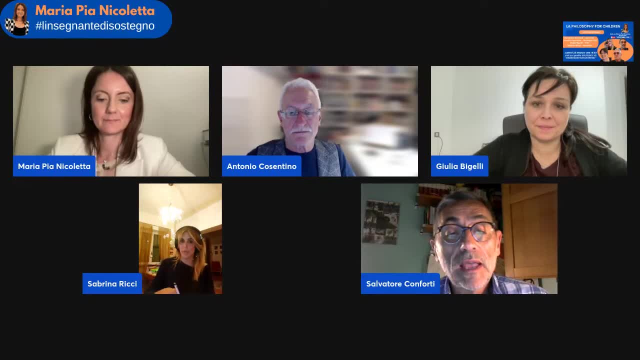 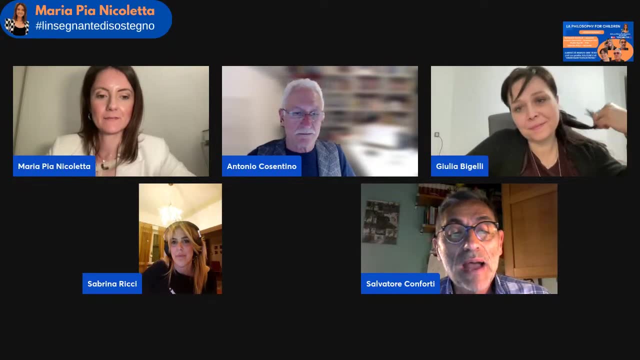 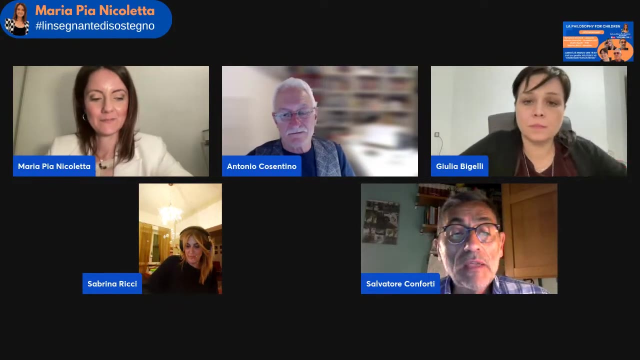 confrontarsi appunto nelle sessioni filosofiche in riva al mare, perché siamo ospiti di questa scuola che ha un, come dire, una terrazza verde sul mare, bellissima tra l'altro. e poi seguirà il giorno successivo. faremo invece un convegno apposito su tutto quello che è successo il giorno. 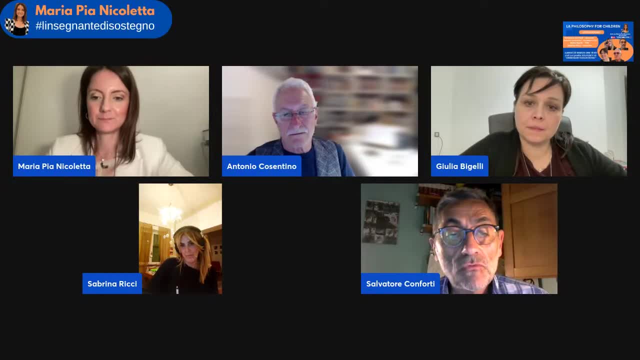 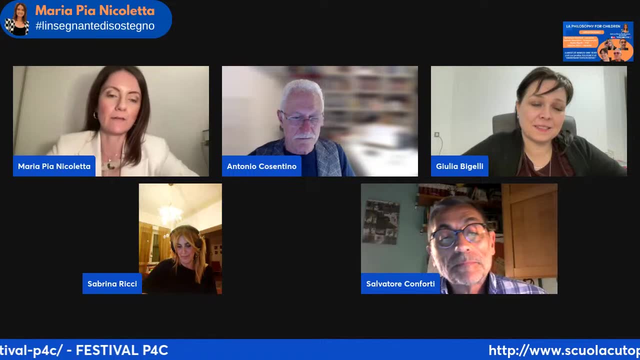 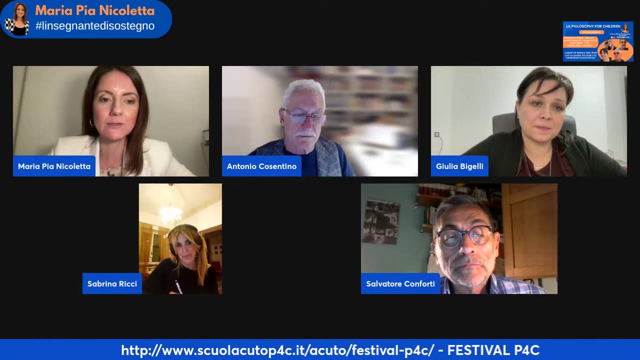 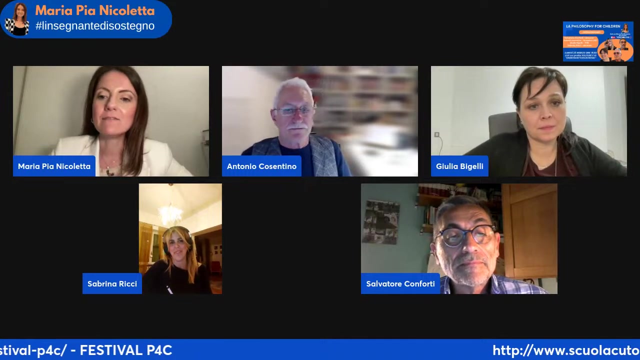 prima, ma soprattutto su quello che intendiamo organizzare per il futuro. grazie ancora a te, grazie grazie, salvatore, per averci, a averci insomma deliziato delle tue informazioni. io passo la parola alla docente sabrina ricci, che va a chiudere questa diretta. ecco, sabrina, visto. 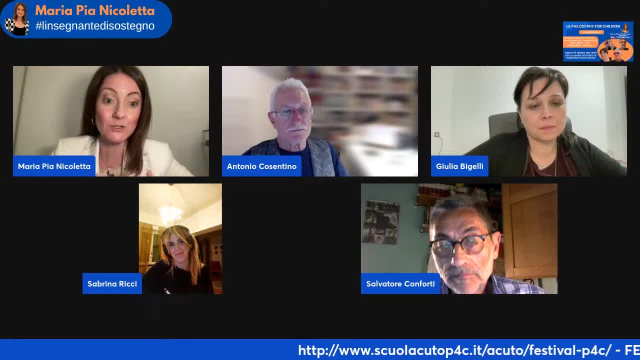 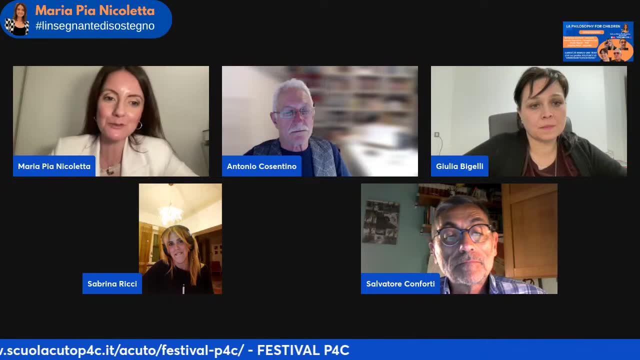 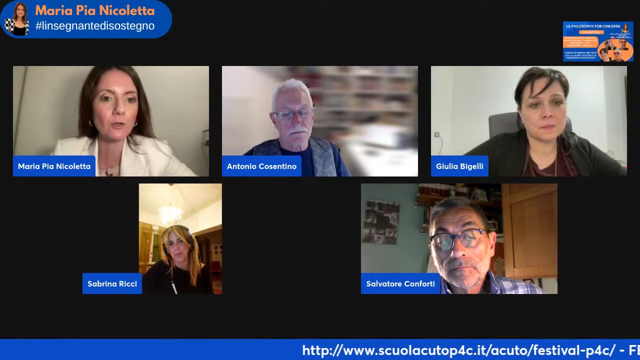 che adesso dobbiamo invitare tutti chi ci segue, che ci iscrive tra questa diretta indifferita al festival, a darci almeno due motivi per prendere informazioni: magari formarci sulla filosofi forci del, visto che hai visto degli ottimi risultati all'interno. 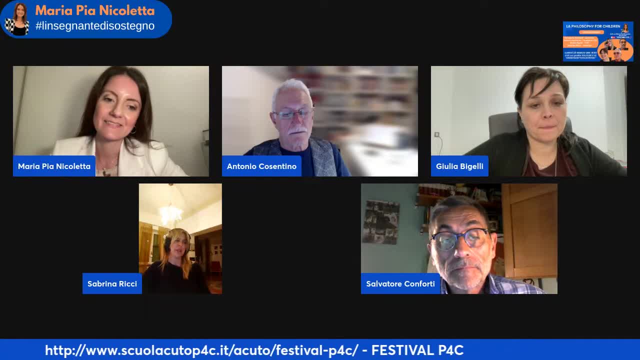 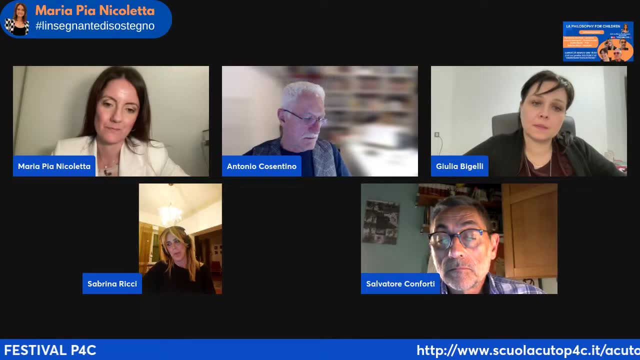 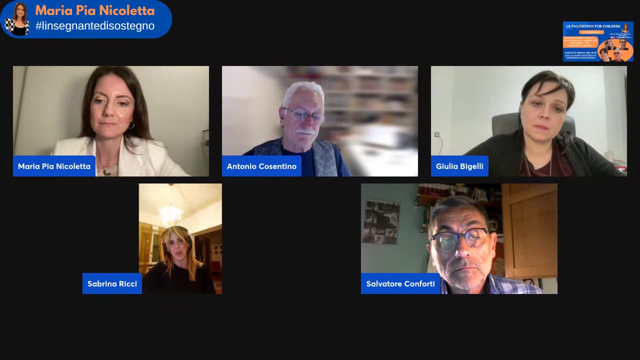 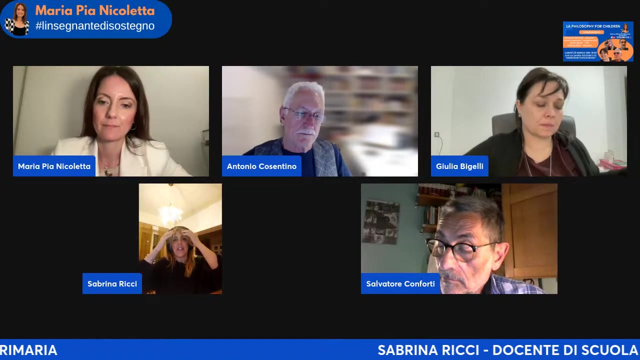 delle classi. certo, secondo me, chi ha voglia di mettersi in gioco, comunque, di di fare, di mettere al centro i bambini, ecco, io dico sempre che il nostro centro sono loro, loro devono, devono essere al centro della nostra didattica. quindi, 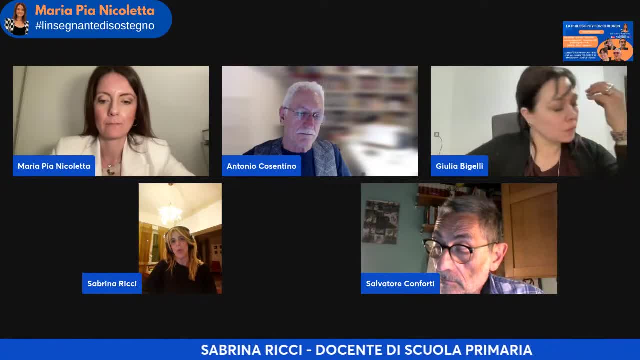 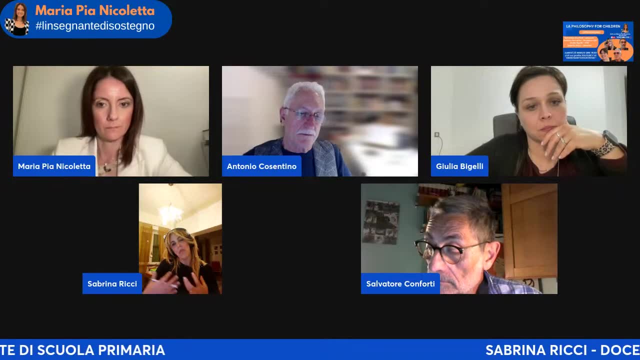 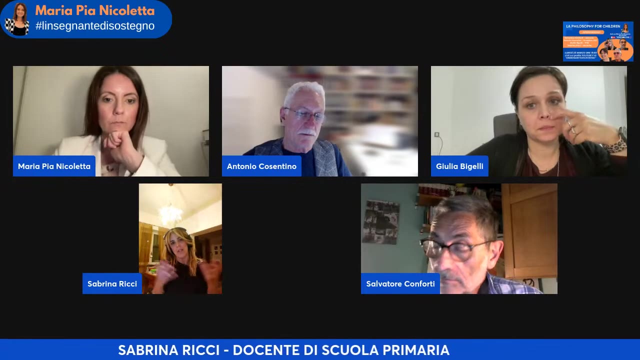 progettare delle elezioni che siano, appunto, coinvolgano, che di, che favoriscano il loro, tutto quello che fa uscire il loro mondo, uscire se stessi. ecco, per me questo è uno dei motivi centrali. 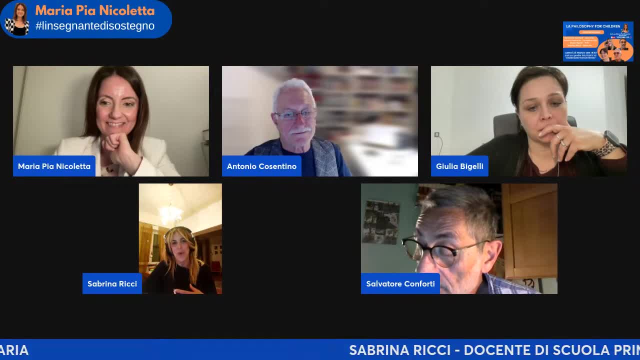 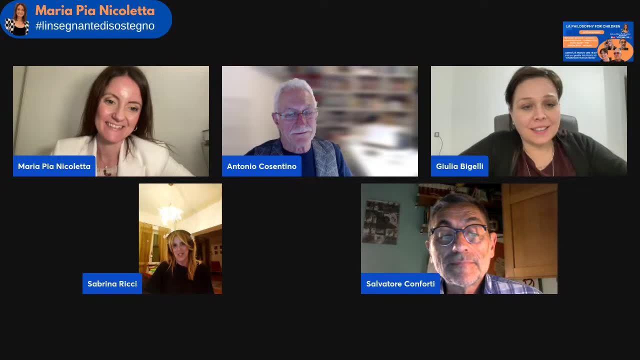 per per conoscere comunque la filosofi e attuar la scuola e presso. anch'io sarò allieva di salvatore, quindi conterà in cori corso. no, dovrò frequentare io. sì, sì, sì, scusami, ti sento un po attratti. sì, sì. 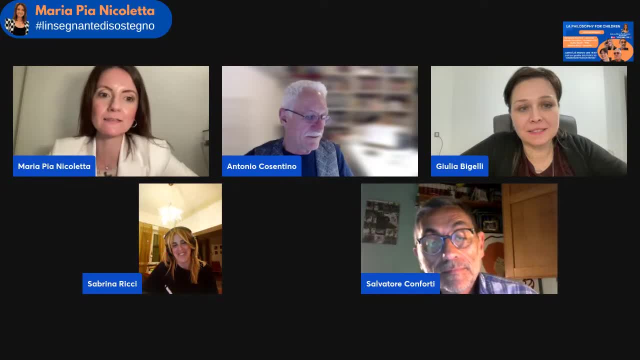 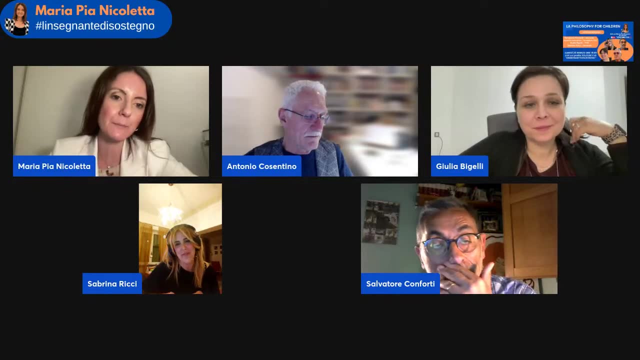 grazie, grazie, sabrina. allora interagiremo informazioni su quella che sarà la tua esperienza. ti w, a me piacerebbe molto invitarvi nuove menti per approfondire ancora più nel dettaglio, essere ancora più specifici. antonio, se ce la facciamo, organizziamo qualcosa proprio per approfondire, per informare chi ci segue, per chi ancora non conosce, a curiosità, magari prima del festival, se riusciamo, così da ricordare l'appuntamento- ed era possibilità- alle persone che vogliono partecipare- di iso e la sua vita su questo live. 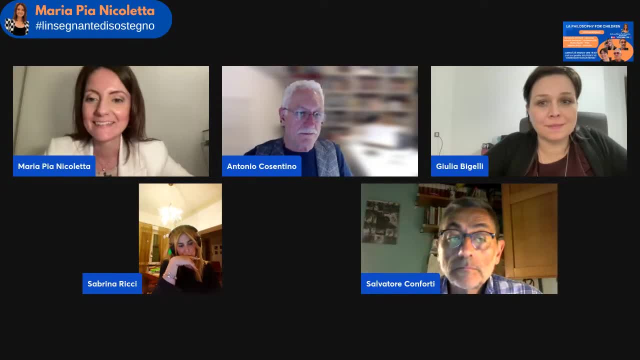 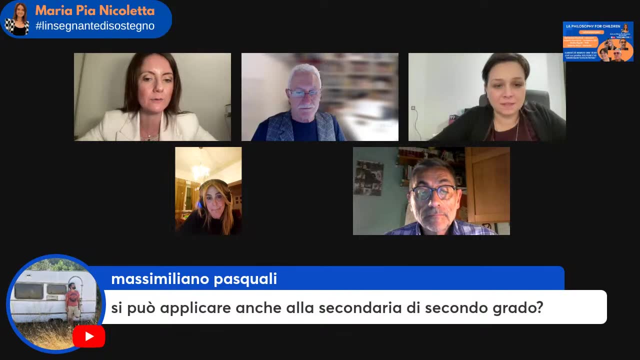 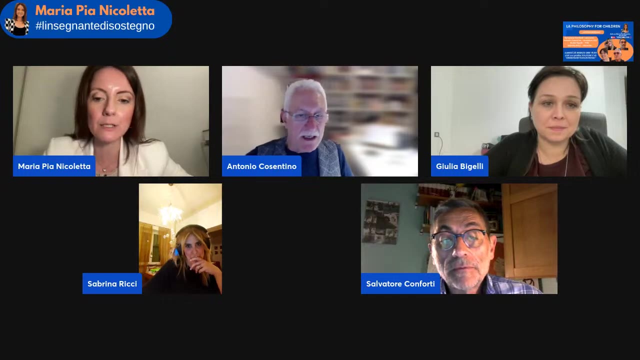 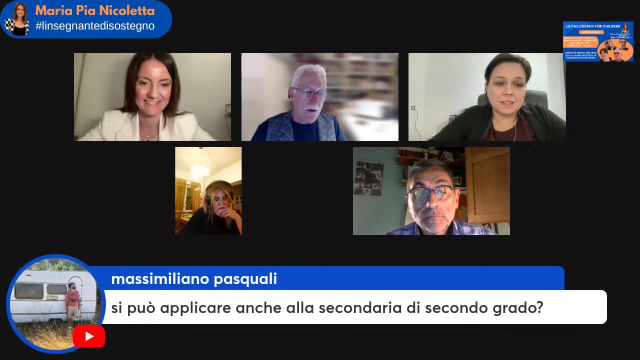 there is a question? Massimiliano does it. I show it here below. it can also be applied to secondary and second grade. Antonio, can you answer it? Wait, we open the microphone and Antonio re-opens the microphone. Yes, yes, philosophy of science is a vertical and horizontal curriculum. since it does not have 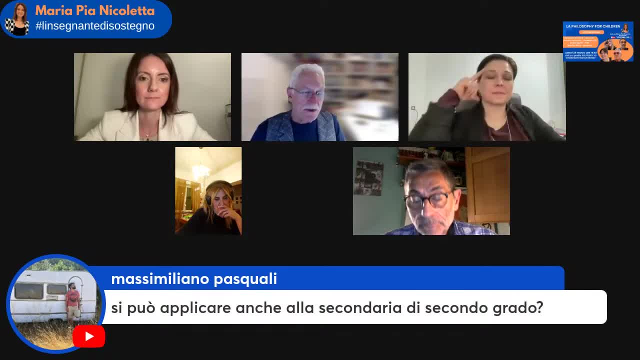 contents but, as we said, it is applied to processes, settings, etc. as a didactic of the research community, then, among the latest very recent research, it is an experimentation rather than an experience. what we are doing is how to teach philosophy, but also the more traditional one, that is, the one that also has 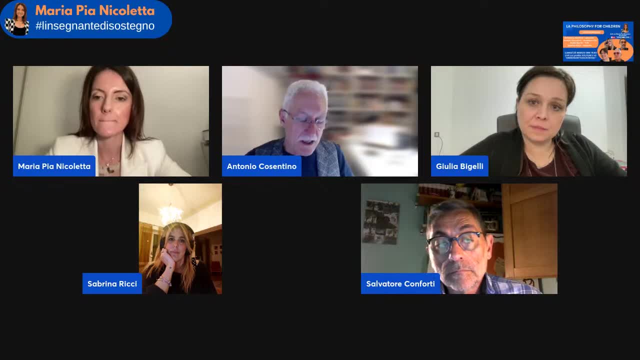 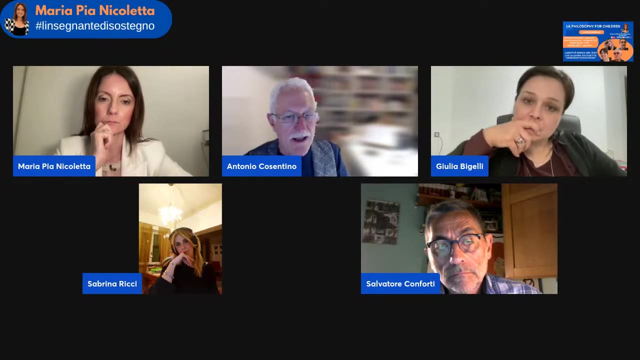 to do with the history of philosophy At high school and university. you have to study the authors if one wants to. I do not really know how to come out saying I know something about philosophy, but you can study in another way. philosophy of science suggests that you can study starting from the experience. the 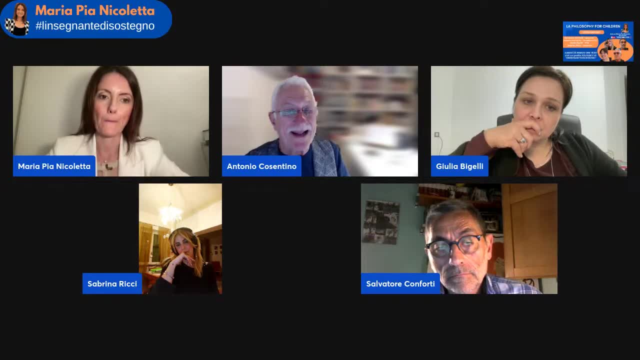 experience of the boys and reflecting on them. to arrive at the authors, the authors arrive as guests to the circle of dialogue. so, even there, or as you can do, you do as practices that are done once a week. what can be done about philosophy of science?